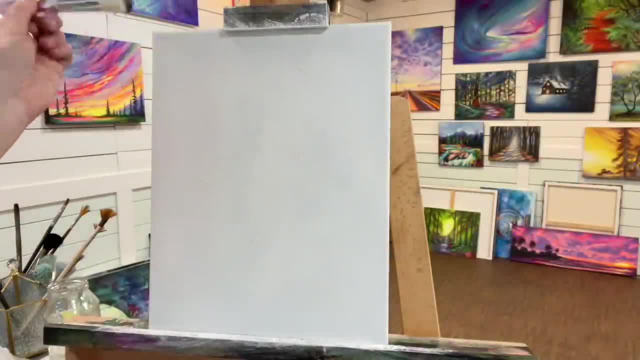 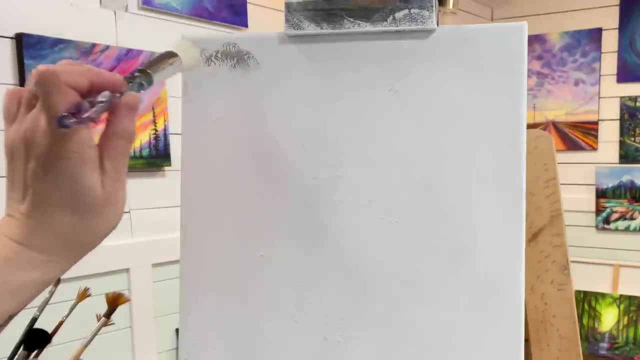 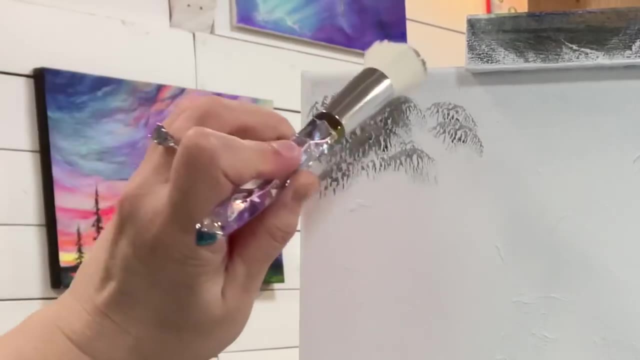 You always want to finish with that tap so you get that little shape that you want. so you're just going to push lightly and tap to see how you're left with those little spaces in between, and it just looks so natural and sometimes your brush is going to get wet from the paint right, so it's going to lose that. 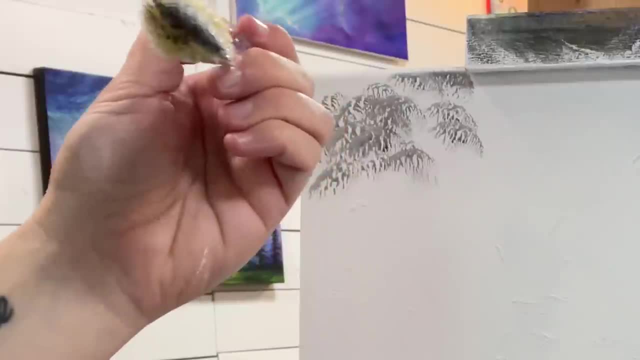 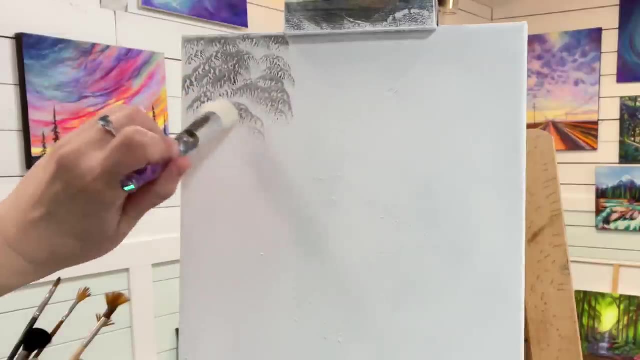 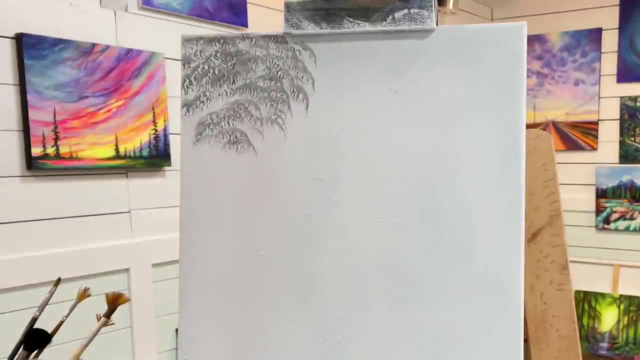 perfect round shape a little bit and kind of go into a little squeezed section like that. That's really nice for foliage as well. well, just take advantage of that, because you kind of get that filbert shape to your brush okay, and so that's one technique: the tapping for foliage. now what you can do after you can pull. 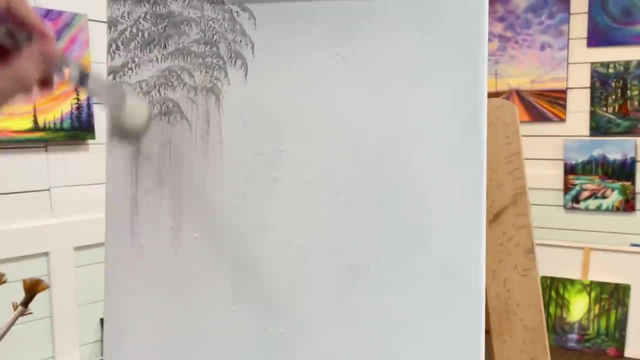 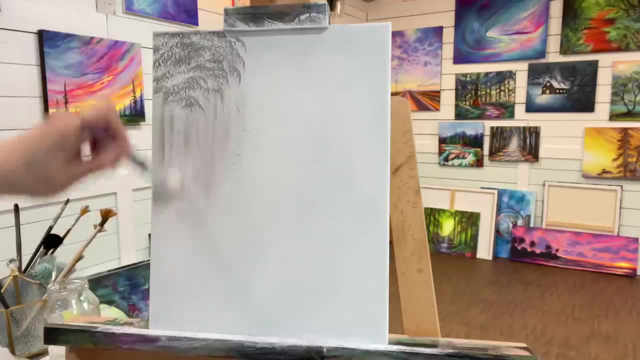 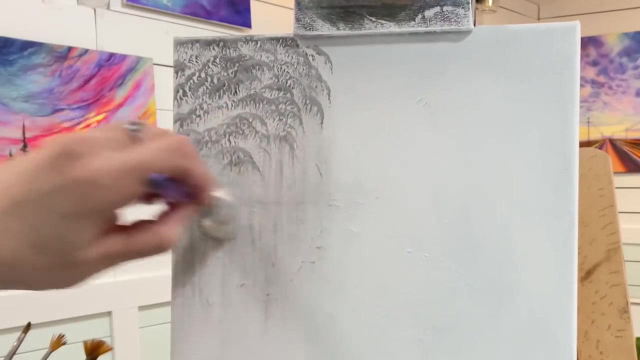 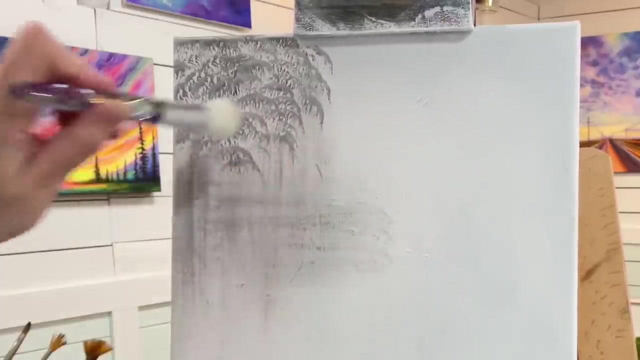 and drag and create this water reflection or sort of drippy, hangy moss. this will work with a little bit of water on your brush too after or dry. so if you go back this way, side to side and up and down, you can get that sort of reflective. 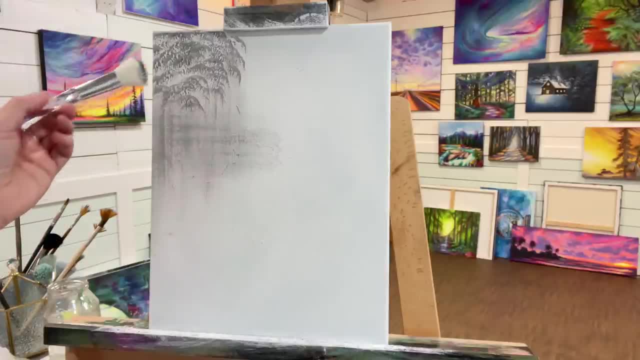 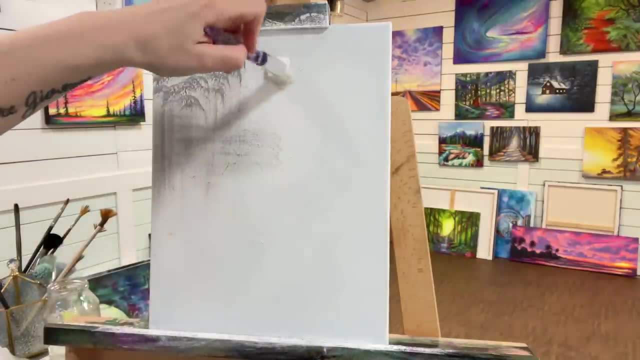 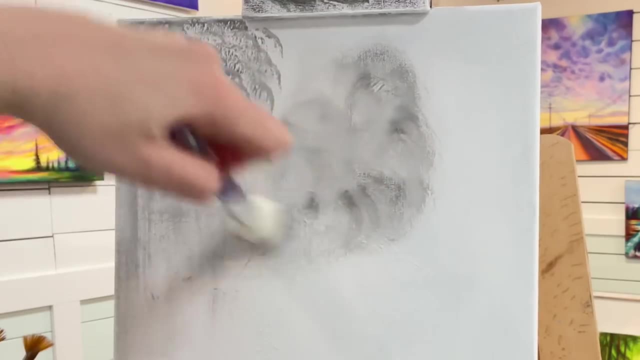 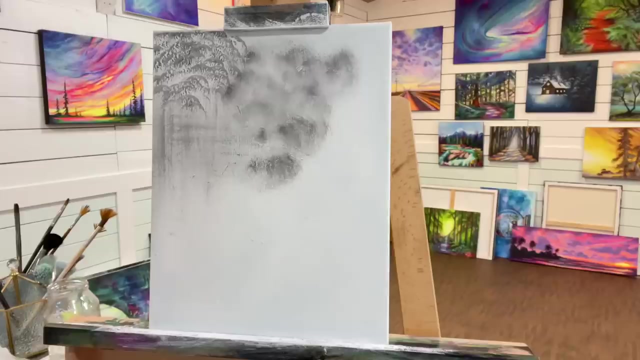 look, you can also use this for a background. and then the other thing that I like to, the other way that I like to use this brush, is by creating soft backgrounds. so I'll go clockwise and counterclockwise and get that really soft blended, almost a smoky, hazy look, and to keep your paints from drying out so that you can blend them a little. 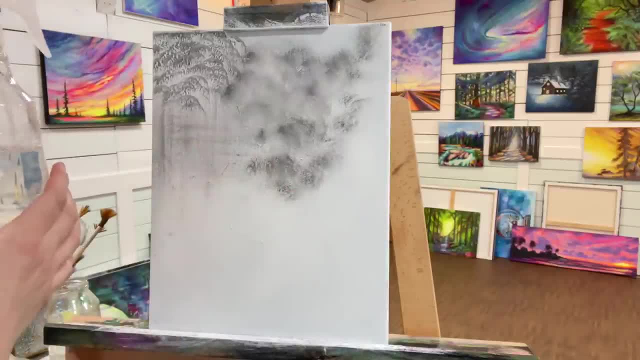 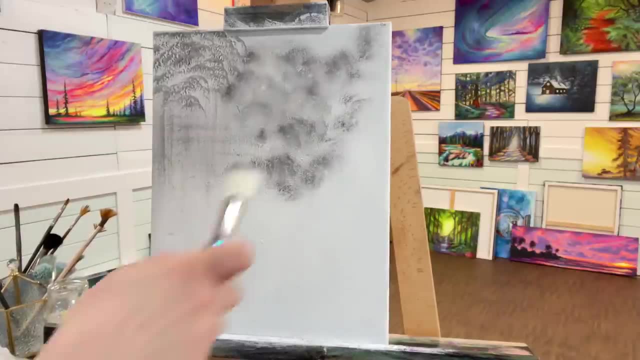 bit better. you might want to think about getting a little bottle like this little spray bottle. have it set to a fine mist and that will help even out the water rather than going right into your water and dipping your brush in, because that would be a lot of water. it's a little bit harder to control. 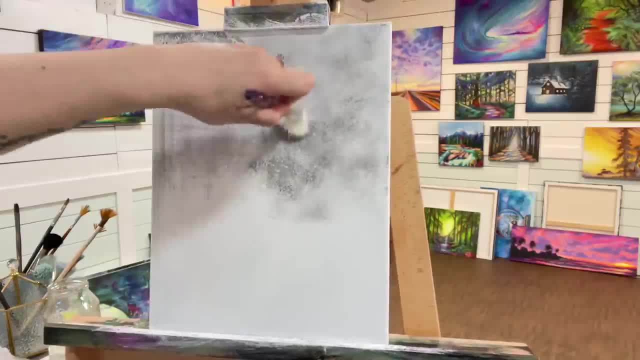 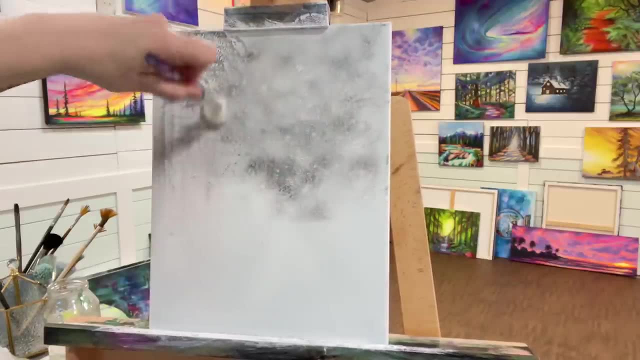 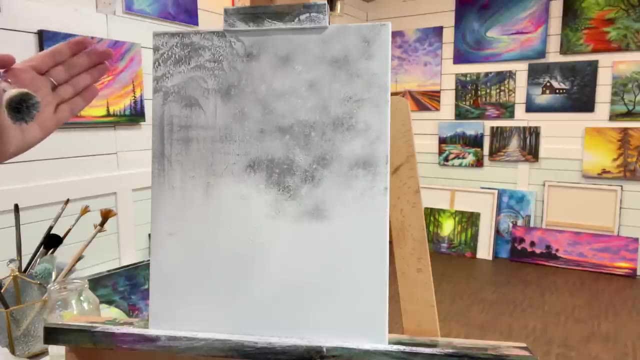 so this type of technique is really, really beneficial for creating soft backgrounds or adding over top of a tree and making it look like there's fog over it, or making it look like it's further back in the distance, making it a little bit softer in tone and a little bit blurry. 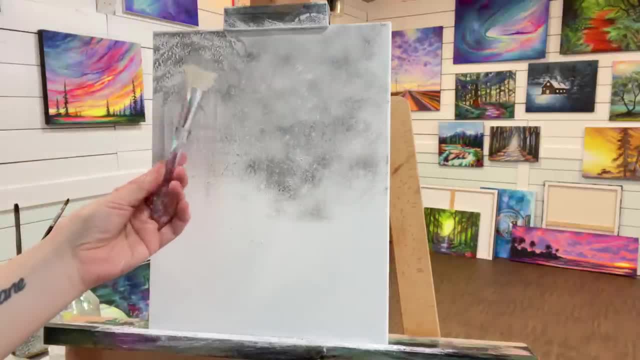 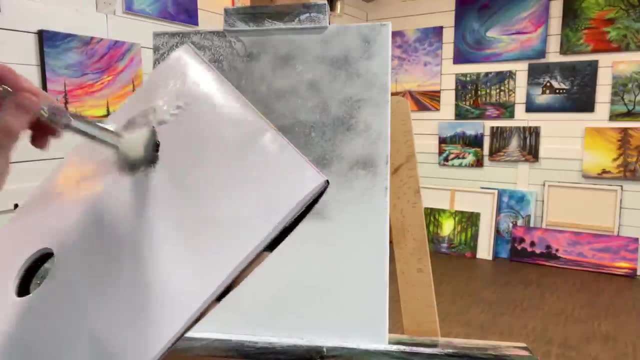 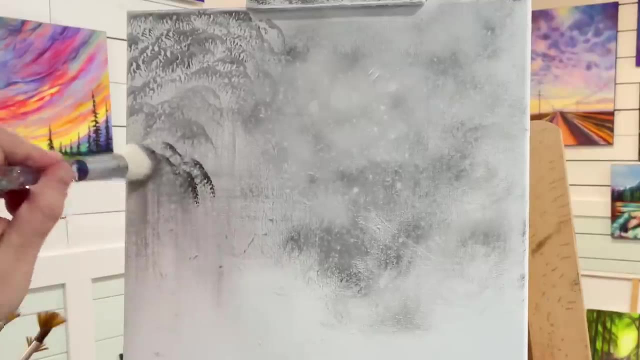 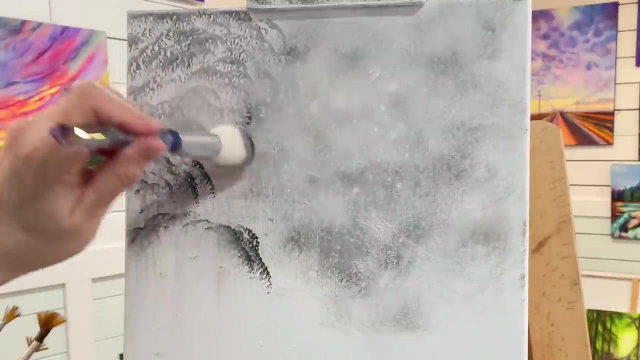 so there's quite a bit that you can do just with this blending mop brush. my favorite is creating little bushes and branches so you can see how I'm kind of pushing it on its side and I'm just using like the top of it. but you can also. 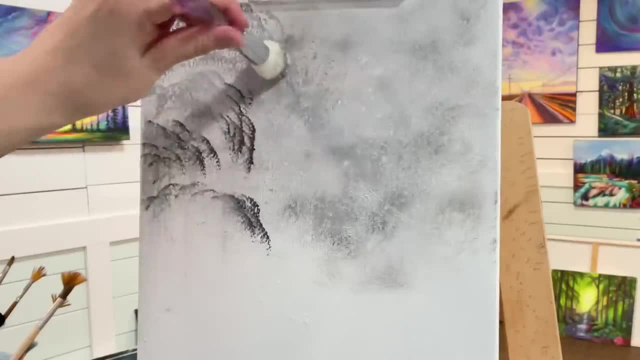 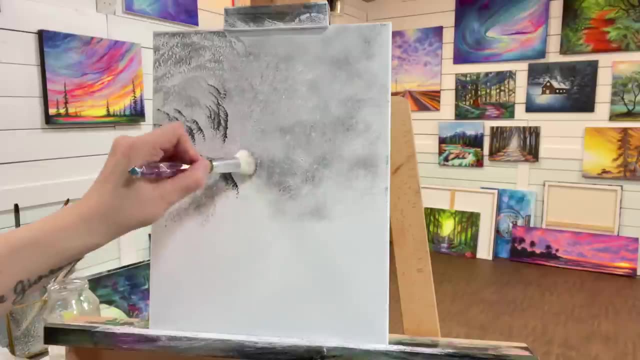 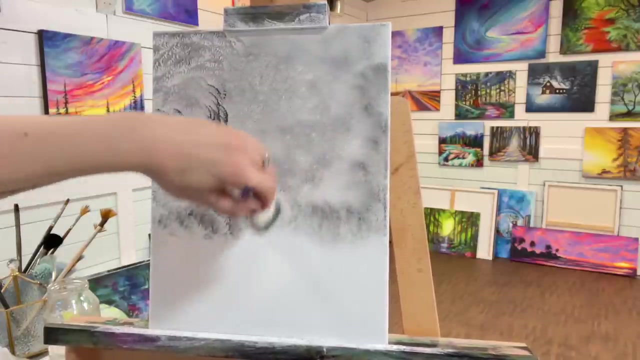 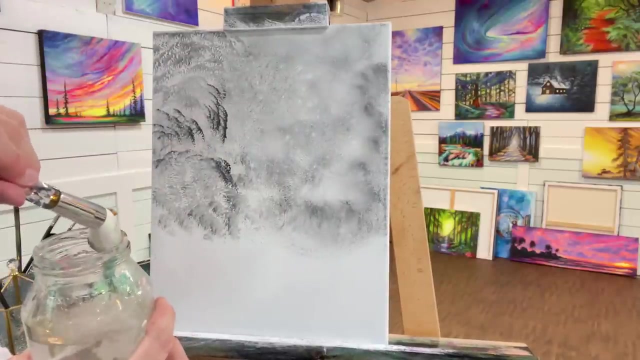 use the whole width to make fuller looking trees, making them look a little bit more round, but it will act. you can make your round. mop brushes act like little filbert brushes too. okay, now to when you get it wet. when you're done using it, sometimes I like to just go off the top. 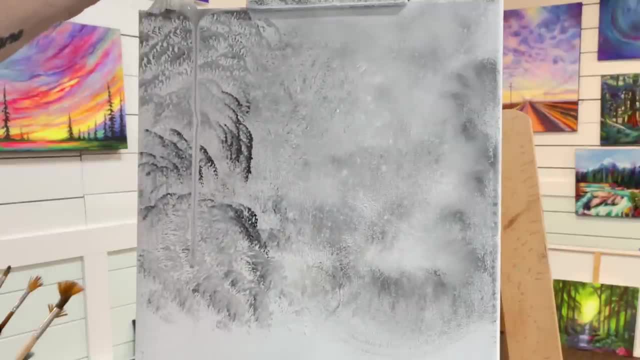 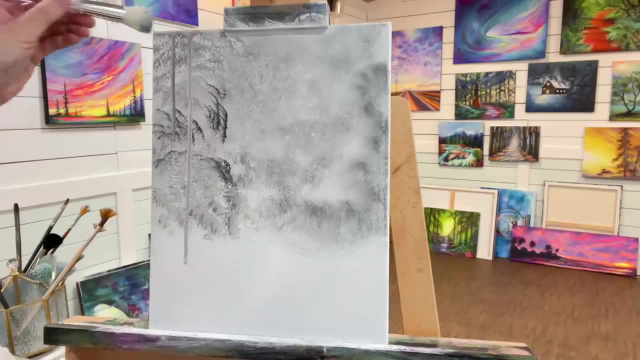 and create drips. I'll release the excess paint that's out of the brush and use it. make use of it in one of my paintings to create drips like this, with a bit of water just pushing and squeezing off the top of the canvas, and this is a really easy and instant way of making natural looking tree trunks and branches. 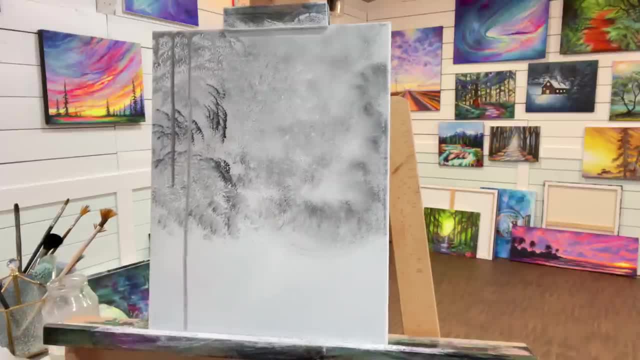 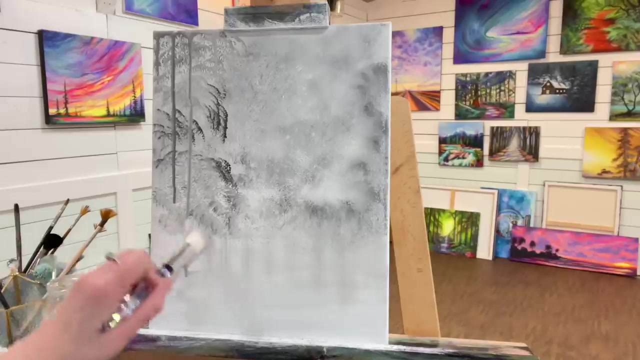 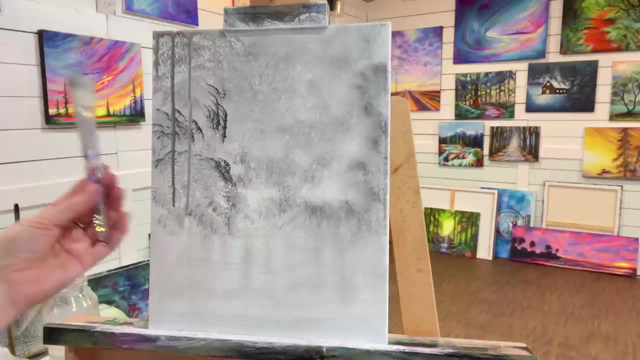 and vines in a painting, then with whatever is left in my brush after doing that, I'll sometimes just just pull down like this if I've got water- a lake or a river or a pond- and that's how I'll create that instant water reflection. look, That's all the. 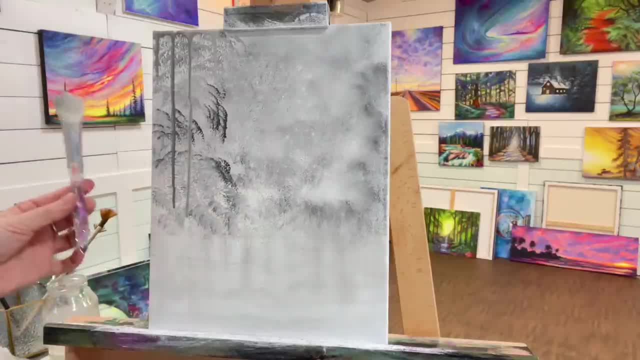 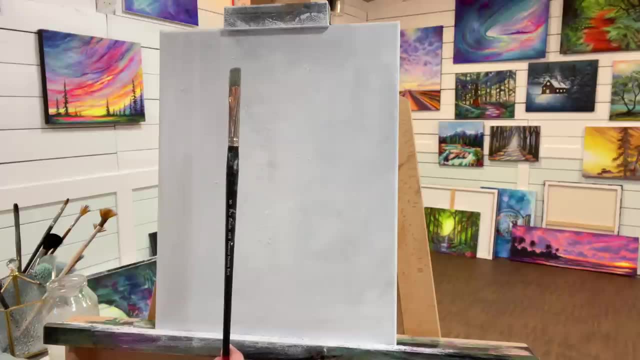 different techniques and ways and brushstrokes you can get by using a mop brush. Okay, so for our next brush, I'm going to be showing you guys all the different ways that you can use a flat brush, and I'm going to be using black and white again for this. and the first thing that I want to show you guys is: 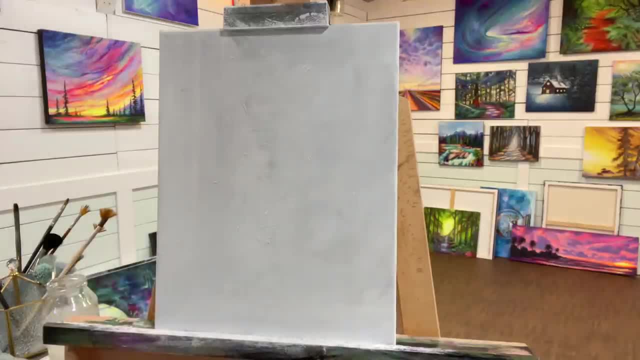 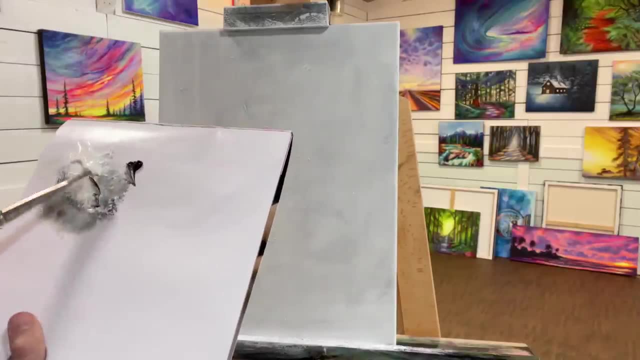 creating a crisscross background using a flat brush, So you're going to want to have a little bit of water first to work with and you want to take a little bit of whatever color or colors that you're using. I don't like to over blend. 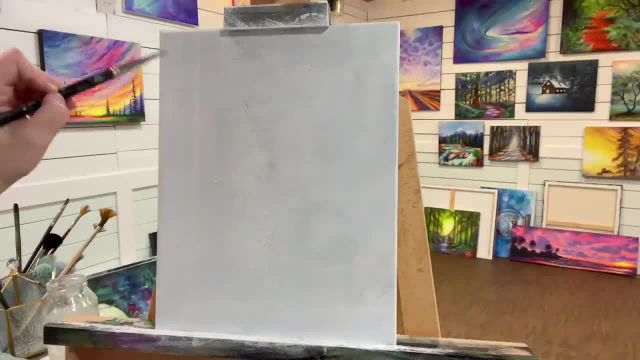 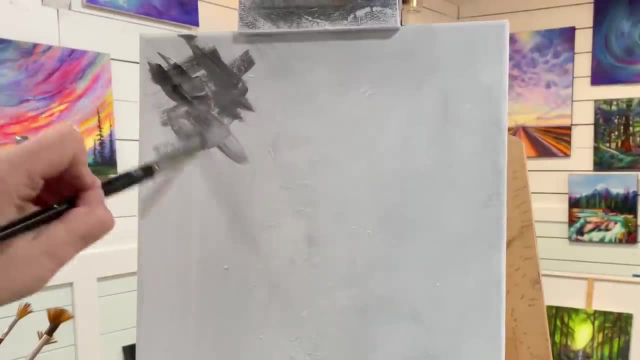 on my palette. I'd like to have a little bit of each color in my brush and just start painting and letting the colors work out of my brush and blend naturally on their own. So just a simple crisscross and I'm going to need a. 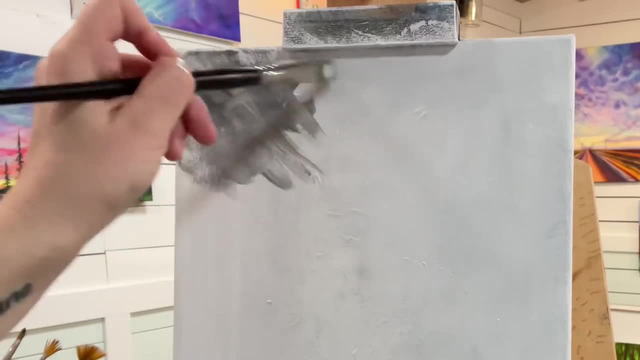 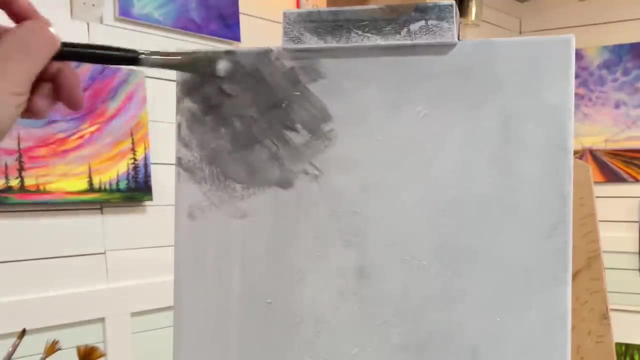 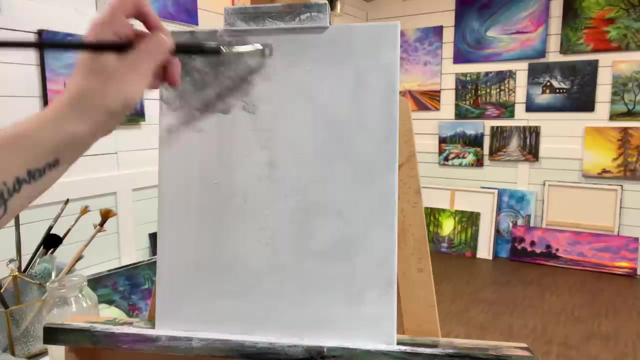 little bit more water. So if you're just looking for different ways and creating a little bit more of a textured looking background, you could just do this simple basic crisscross and you can layer over as much as you want, adding more white in certain areas or 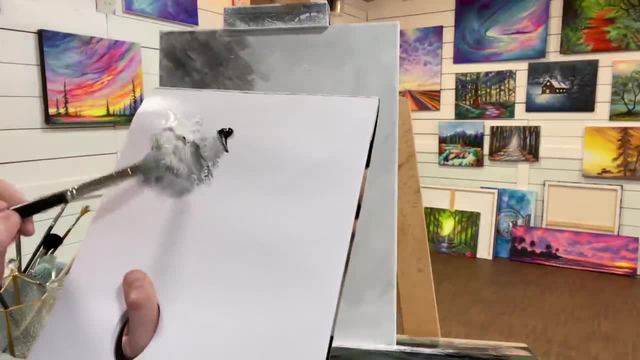 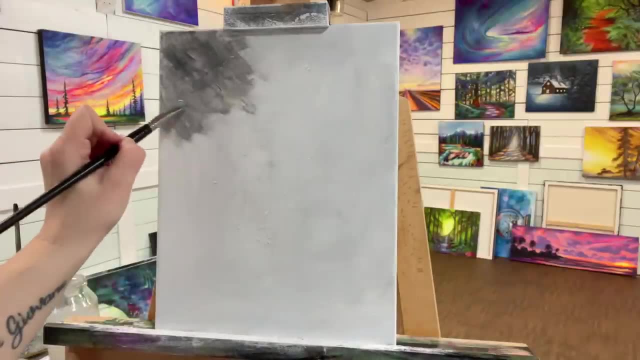 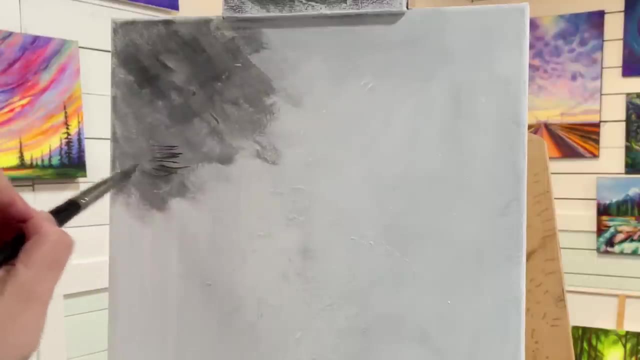 more of the color that you want to use. So the next thing that you can do with this brush is create a little path. Now I'll take a little bit more black, my darker color, first, So starting off just side to side, and you can start to turn your brush like: 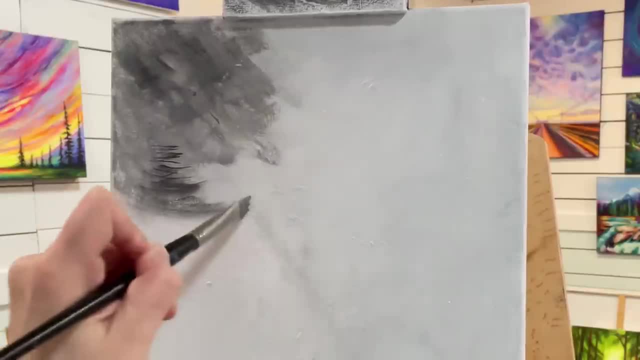 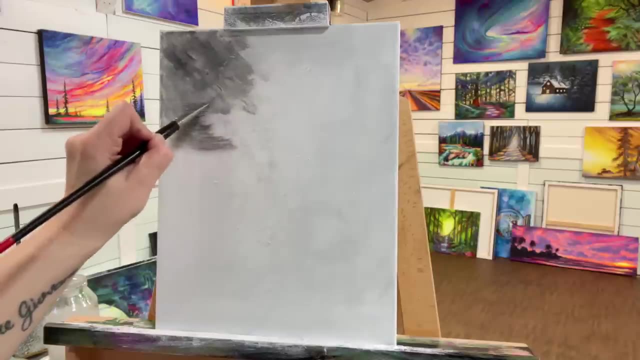 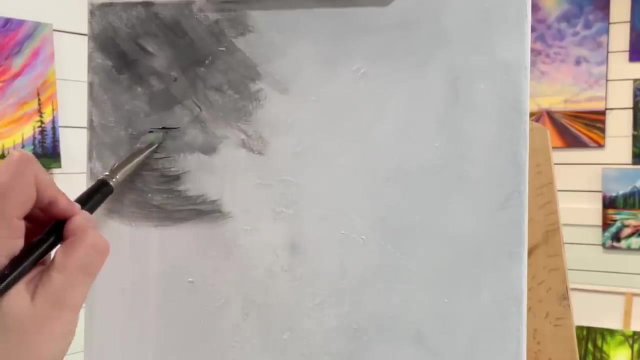 this: if you want to create more of a scoopy, well-beaten path, look And then, as the path gets further away, just do smaller lines so you can create a path or road Stairs. we can quickly change this into stairs. Just simple lines, just using the. 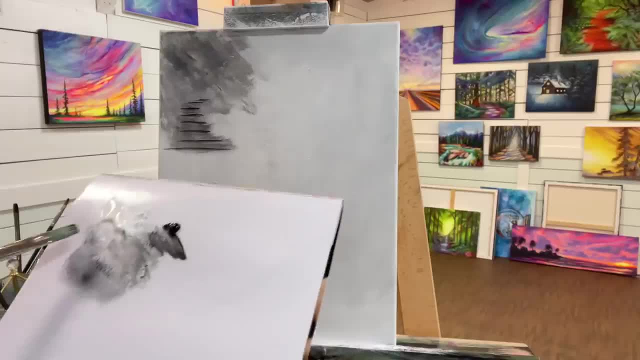 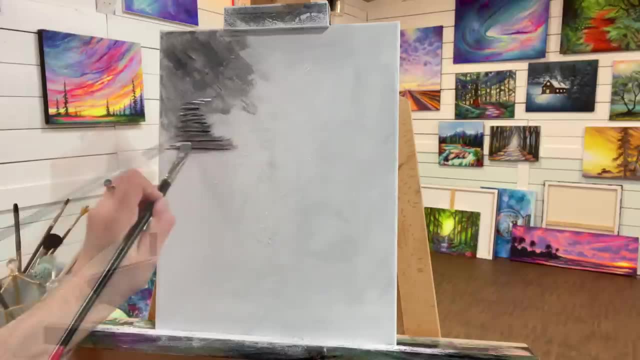 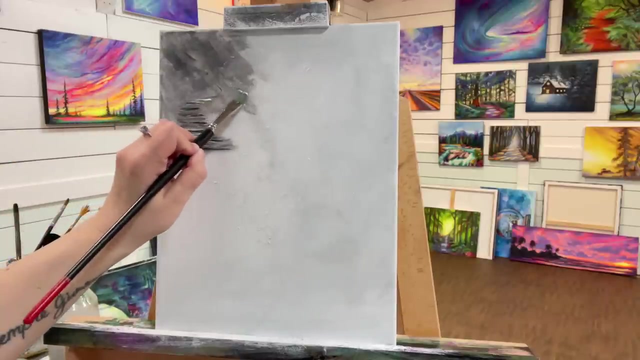 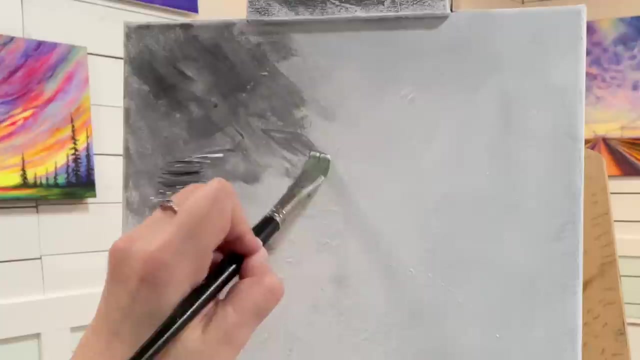 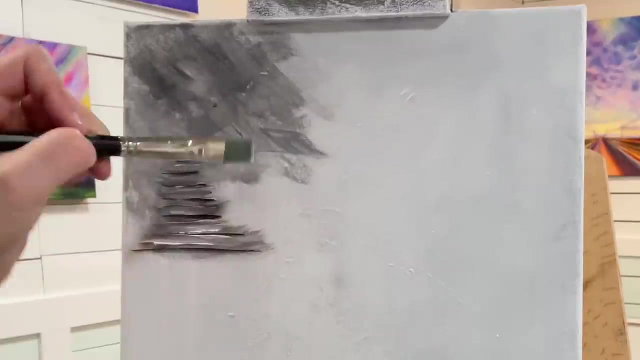 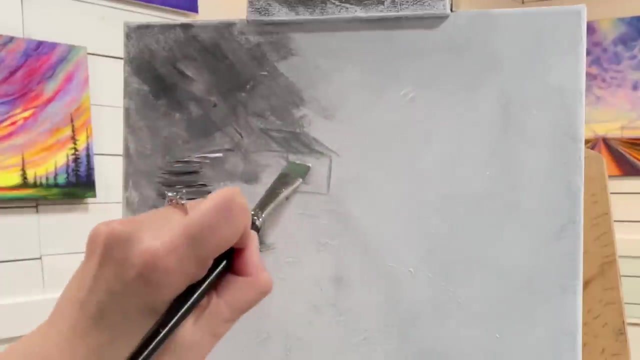 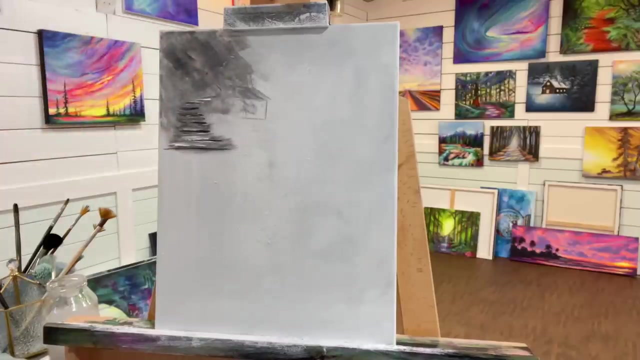 end of our brush. Okay, then you can take white. You can also use the nice edge and flat width of the brush to create a little house. So a flat brush is really nice for creating those straight lines and edges that you want. Okay, if you want to paint a structure, then this is what I would really. 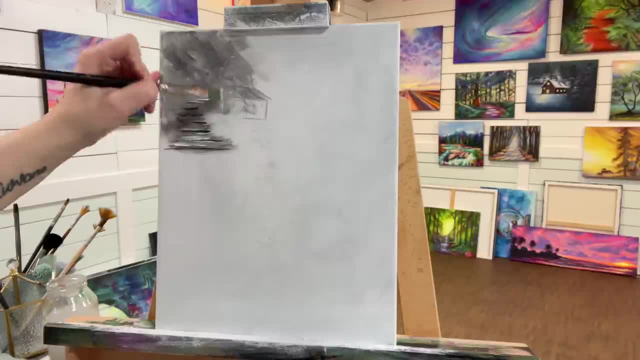 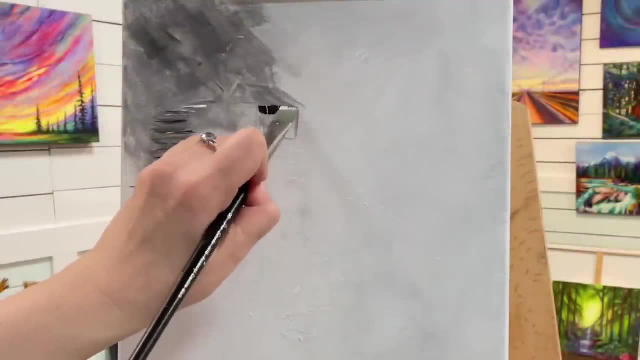 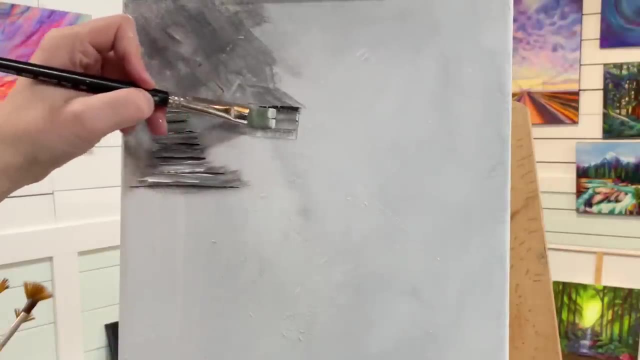 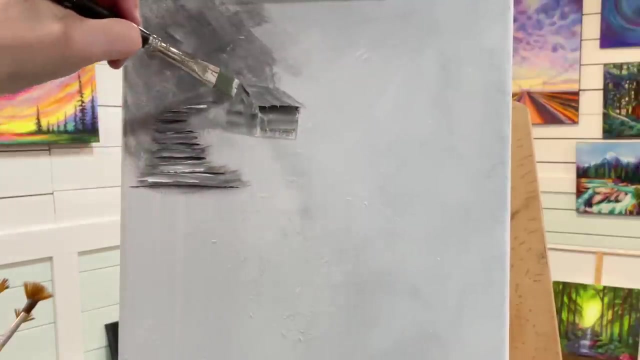 recommend using That's when you're really going to want to use the flat brush. I like to use my back of the brush to paint these, So that's something that I keep in mind when I paint, And then you can add some astonishment to this. 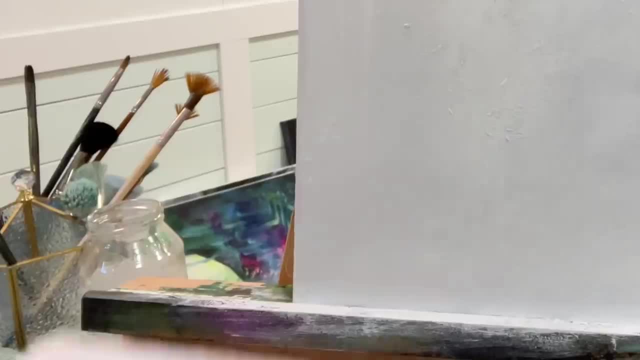 All right. so now I'm going to go ahead and start to paint my face. So start to paint my face in a similar way to what you've done before. So first I'm going to go ahead and shade this color. So I'm going to go ahead and just give that a little bit of a shade. 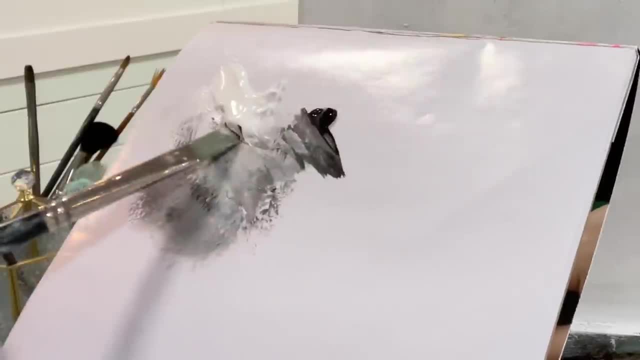 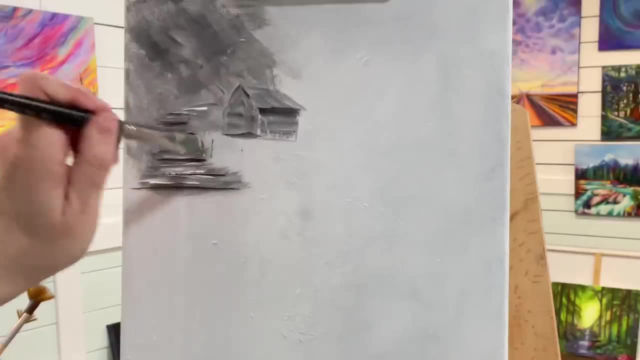 And then I'm going to go ahead and just take a shadow, And I'm going to take my brush and just go ahead and do the same thing that I just did: an instant fence, Depending on the width of your flat brush. sometimes you can just tap like that. 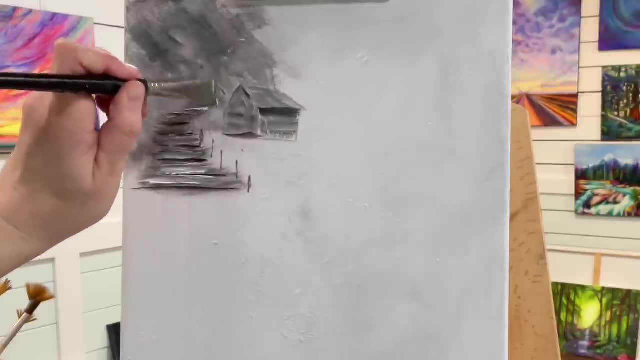 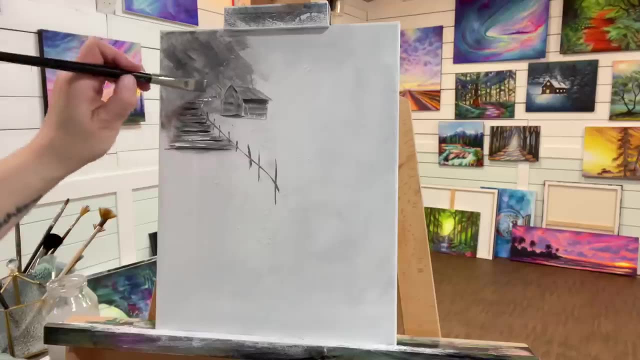 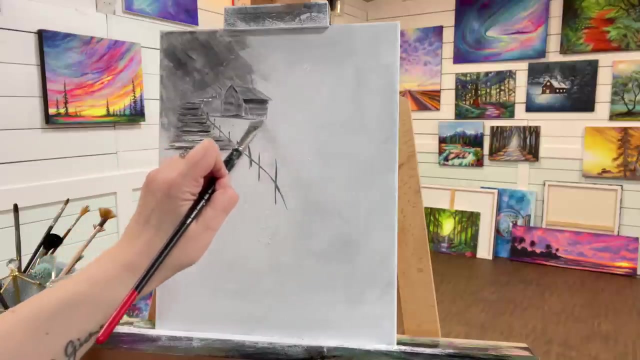 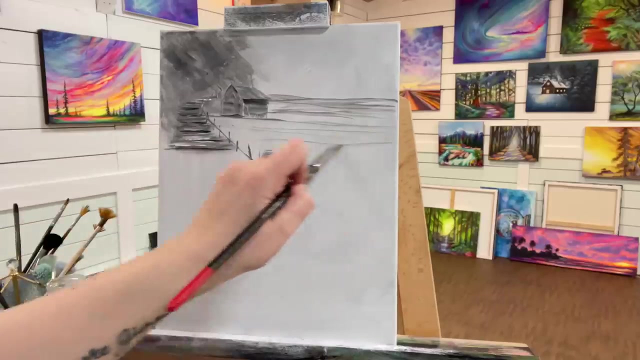 and then if you want them to be smaller, then just use the little corner of your brush or bigger, and then just pull a line through. And, of course, another thing you can do that's really helpful is creating some horizon lines, straighter lines. You're definitely going to want to use a flat brush. 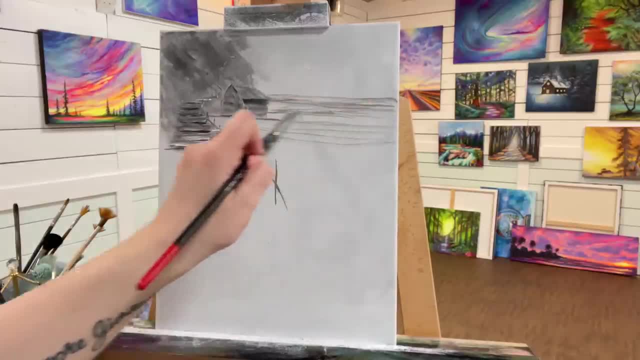 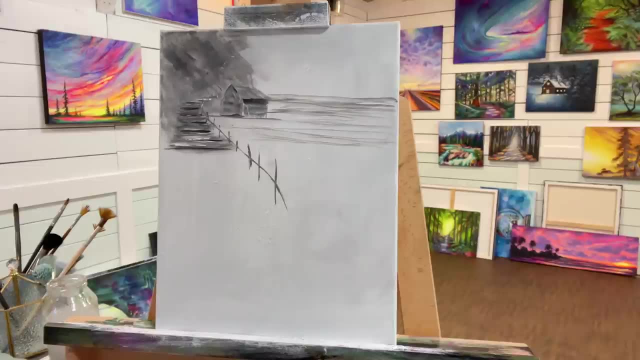 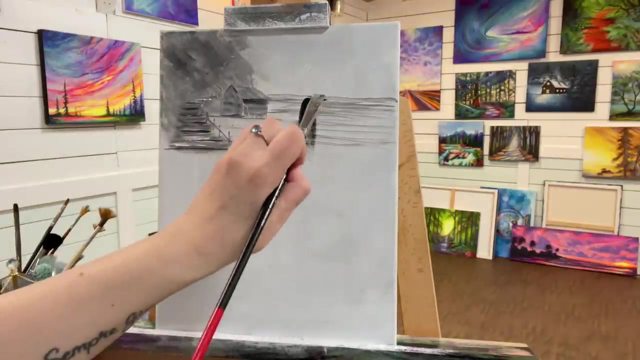 It's also handy for creating water ripples in the water, soft little waves and, of course, waterfalls. So I'm just going to create a dark background first, and you really want to have the paint like a quarter of the way down your brush and on the tip, And what I like to do is just line. 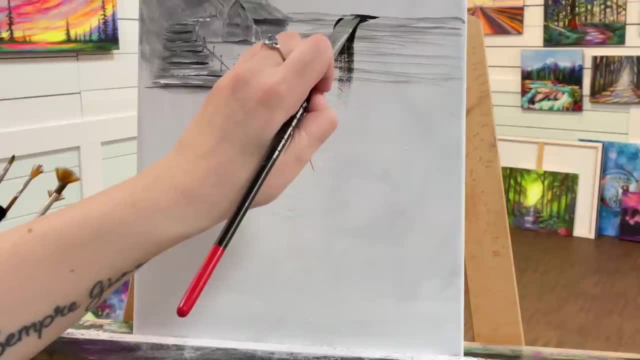 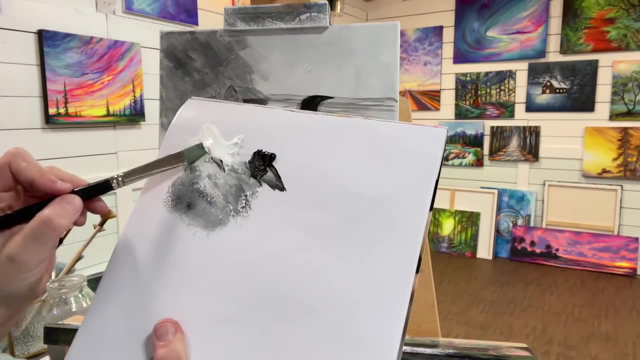 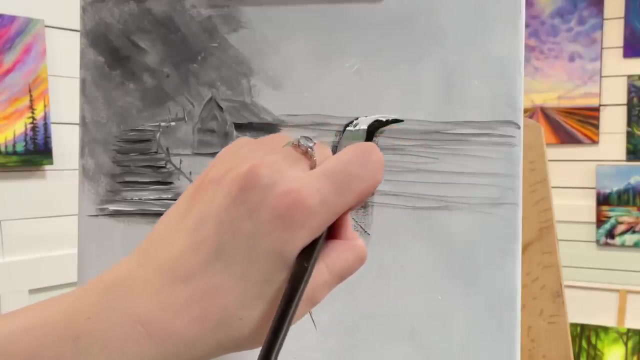 my brush up where I want my waterfall to start, and then pull, and then curve and flick. Pull, curve and flick And then take white, and this time not pushing as hard but just being very light. Same technique. I'm going to load my brush up again. This time I'm 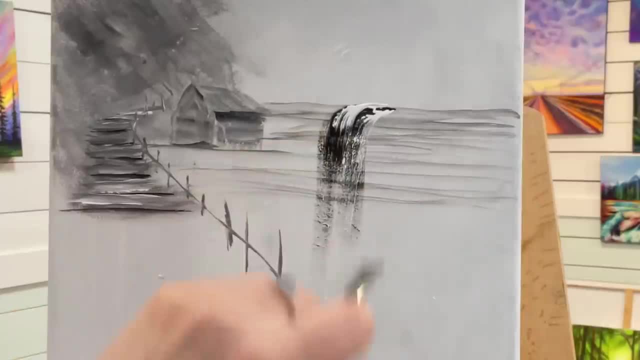 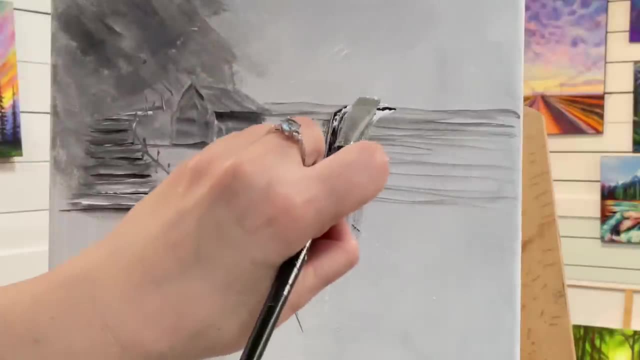 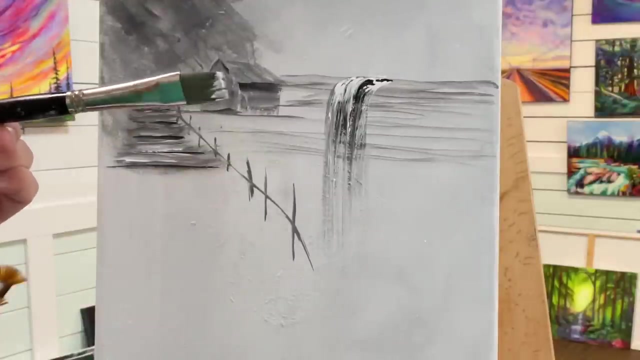 only putting it on the very tip of the brush And then, if you want, you can turn your brush to the side like this, And sometimes your flat brushes will kind of separate into chunks like this, leaving some spaces separating and leaving some spaces through. That's even more handy. 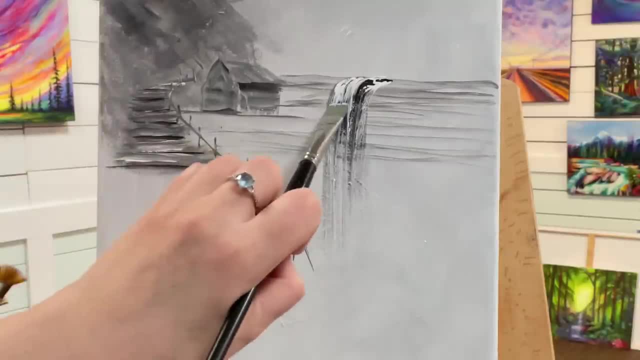 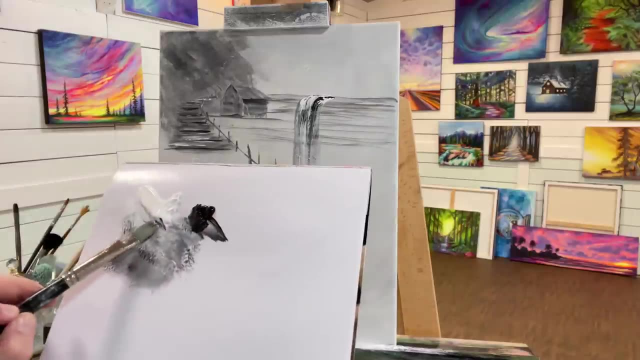 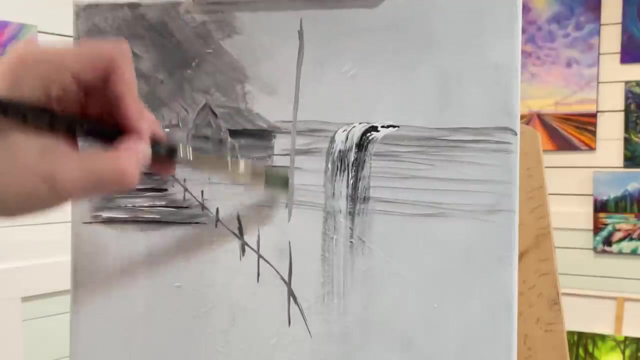 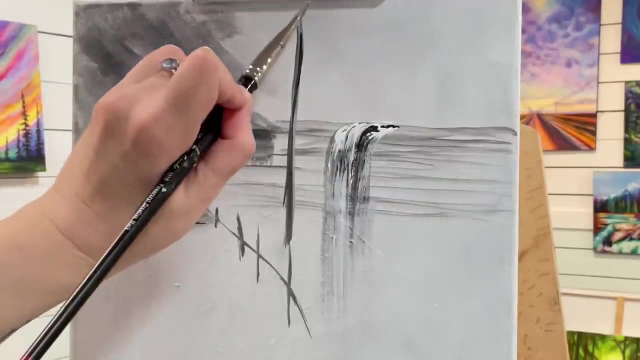 and helpful when painting waterfalls, because then you get those natural spaces in between. You can also paint tree trunks and trees. We'll do a tree trunk just with the very end of our brush. Use a little bit more black this time, And then at the top I'm just going to use the tip of my brush and then I'm going to start tapping. 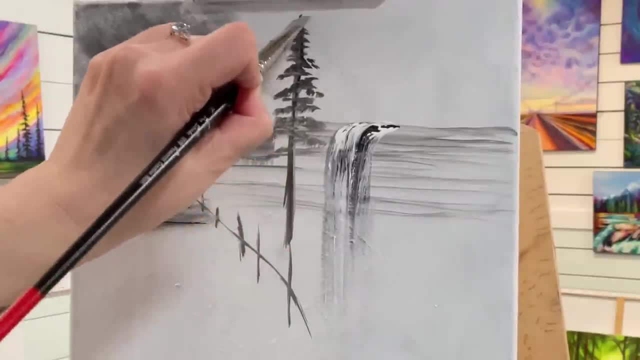 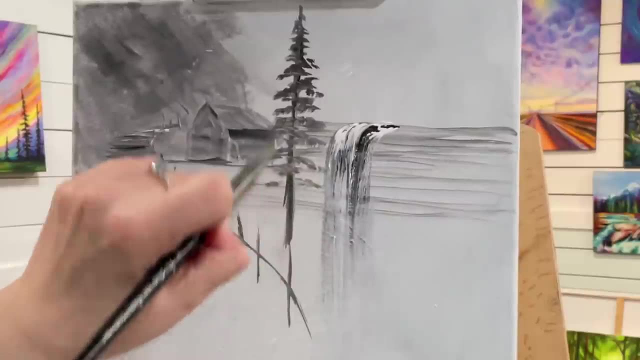 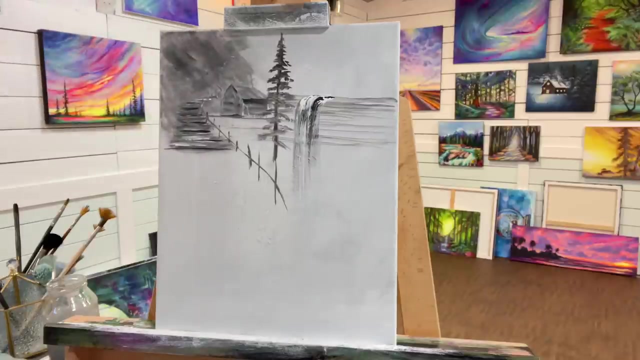 pushing and tapping And you can get sort of that stipple effect. I prefer, to be honest, using a filbert brush for these types of trees, But if you don't have a filbert brush, you can definitely use the flat brush. One more technique with a flat brush and then I'm going to move on to 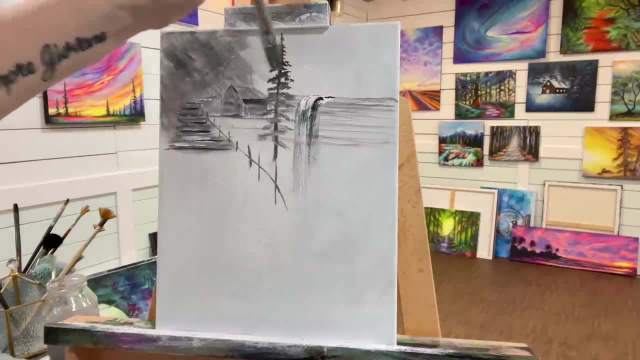 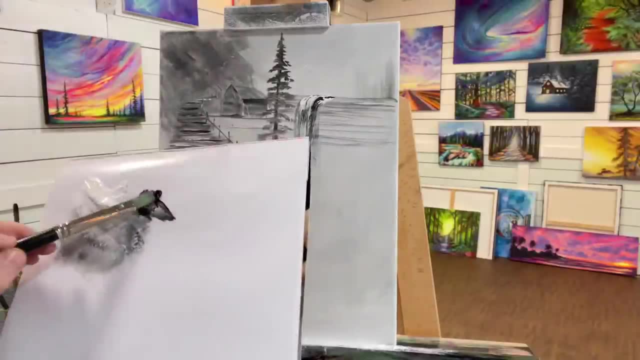 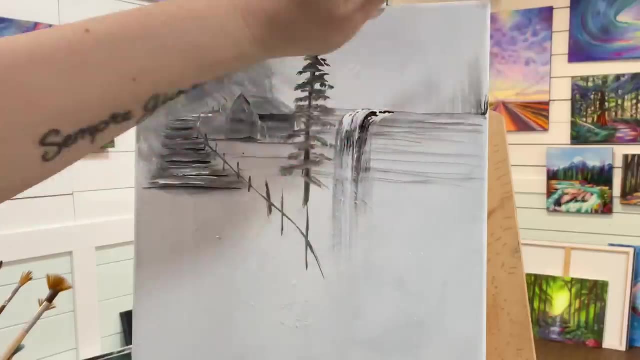 the fan brush And that's push, pull and flick, And what this does is it's going to give you a little bit of depth. So what this does is create an instant little background full of trees. You want to definitely have a little bit of water on your brush, So it's a really quick. 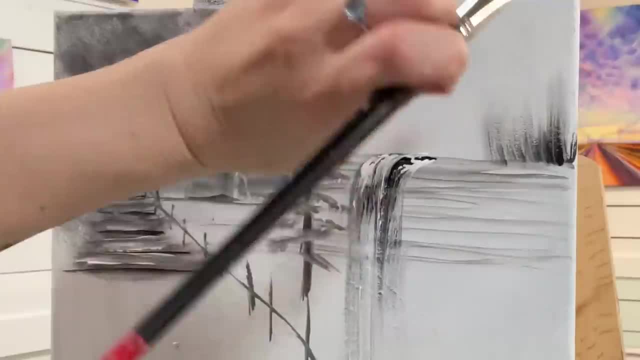 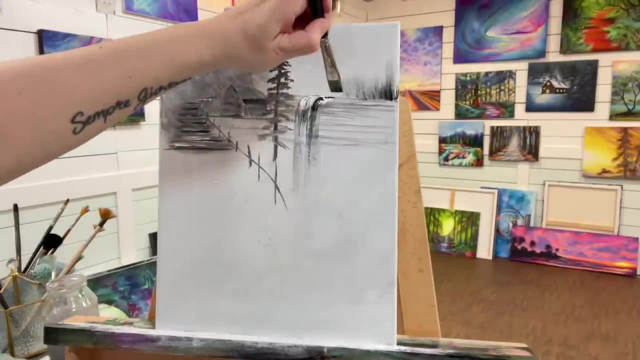 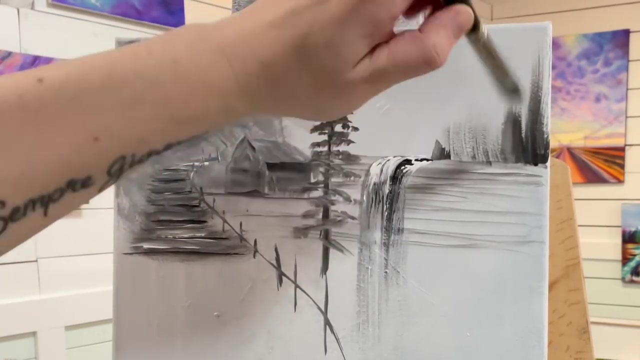 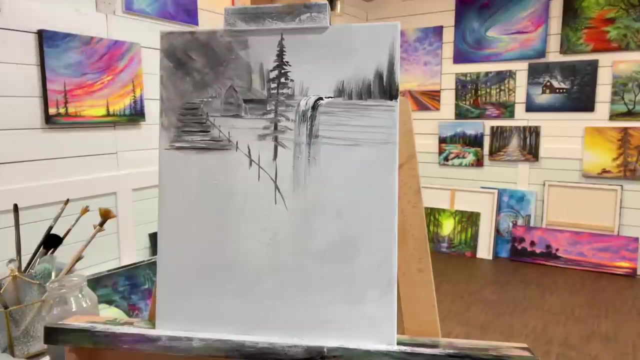 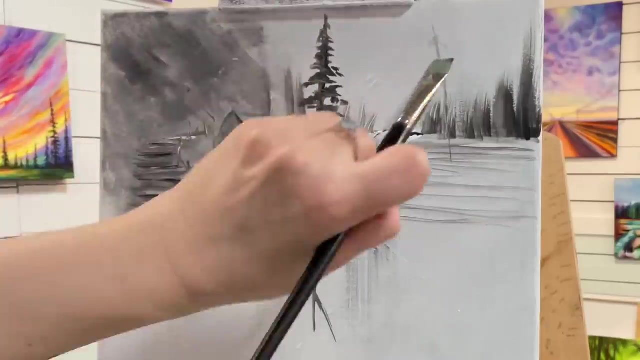 my wrist is going like this And I always like to create some perspective, making my paintings a little bit more dramatic, So I'll pull longer wherever I want my trees to be Taller, and then shorter little flicks. Okay. so let me get that instant forest look before you start adding your. 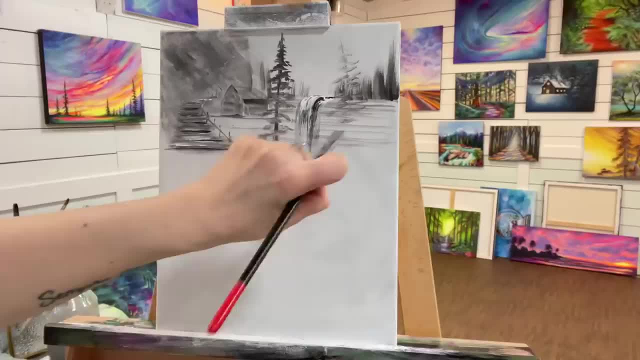 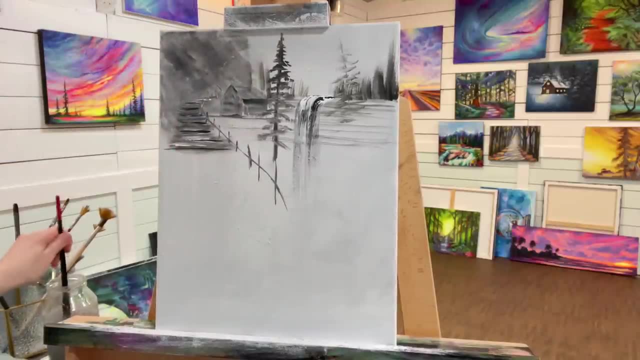 trees that are more in the foreground. It's a great way to build your landscape. Landscapes have been layers, Okay, so we're going to move on to the fan brush. next, I'm going to use a little bit more black, And then I'm going. 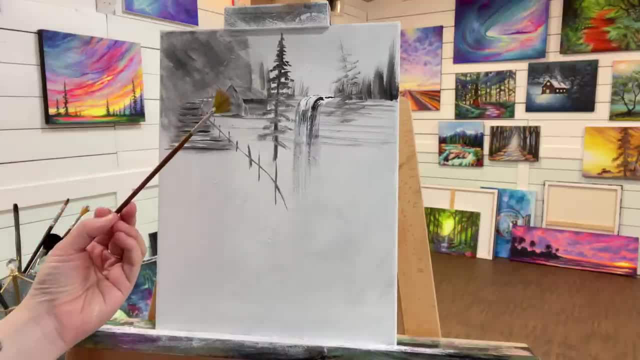 to add a little bit of color to the trees. So I'm going to add some more color to the trees And I've got a little fan brush here. This is the number two, but I've got lots of sizes And I really recommend- and I go over this a lot in my videos- when buying your brushes, make sure. 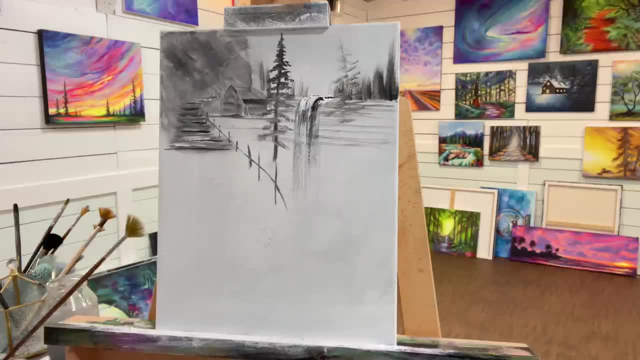 you try to buy two, at least two different sizes, So that you're able to paint a smaller tree with a small brush and not trying to paint something small with a brush that's way too big for that, Because it's going to be so difficult and make it a lot harder for you guys and you're going to get. 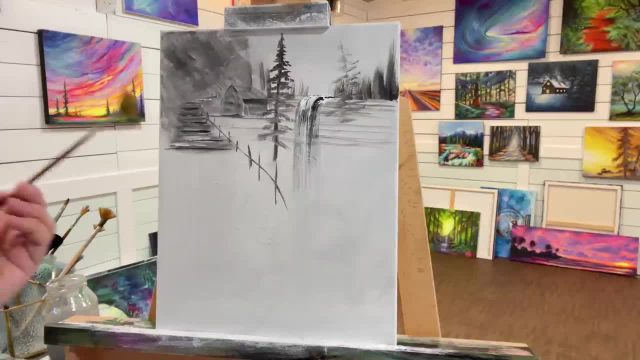 frustrated, So keep that in mind with all your brushes. So for the fan brush, there's a few different ways you can use it. You can use it dry, You can also use it wet. It's really, really an underrated brush. A lot of people think you can only use it. they associate it with just painting. 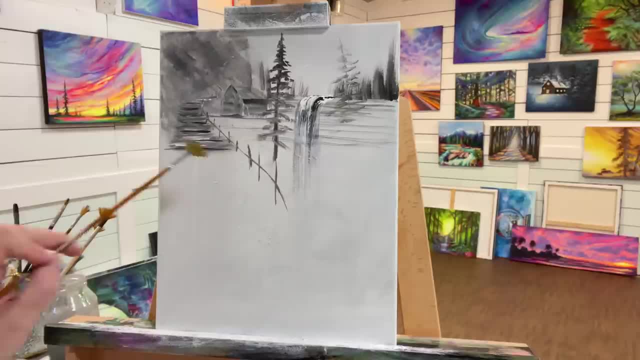 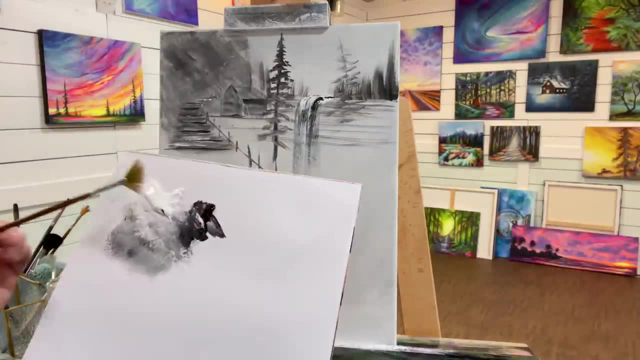 trees or waterfalls, But I use it for so many things. I use it for creating flowy paths and patterns. So I'll just give you a demonstration right now, First using it dry. So if I was going to paint a tree, 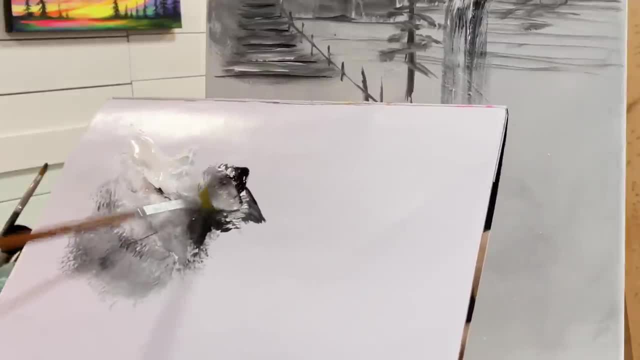 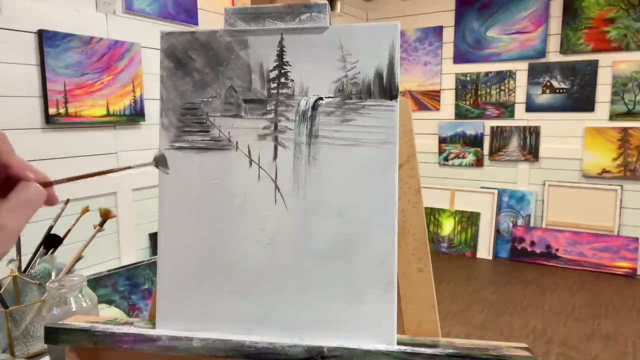 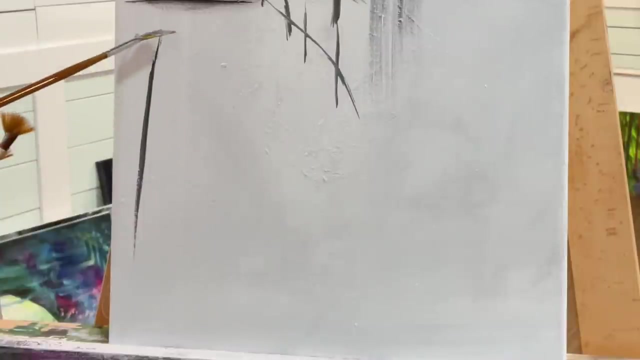 I would like to use my brush dry, So I'm going to make sort of a dark color here, Taking a bit of my white and my black, And I'm going to go right in here. That'll just pull the tree trunk right there And then I'm going to just start to tap. 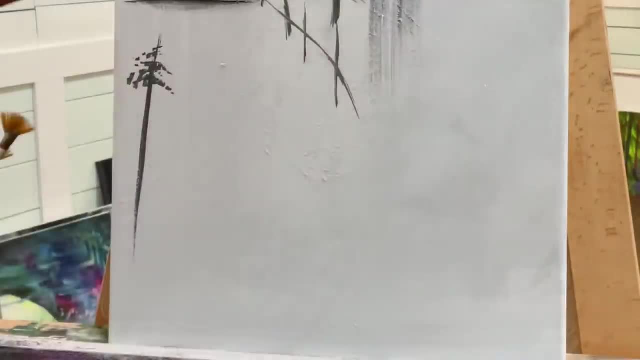 And right away. I'm already a bit frustrated because those bristles are spreading apart too much. That's why I like to use a few different other brushes for painting trees, But this is how I started out, So just by tapping. Let's see. it's going to keep doing that, So 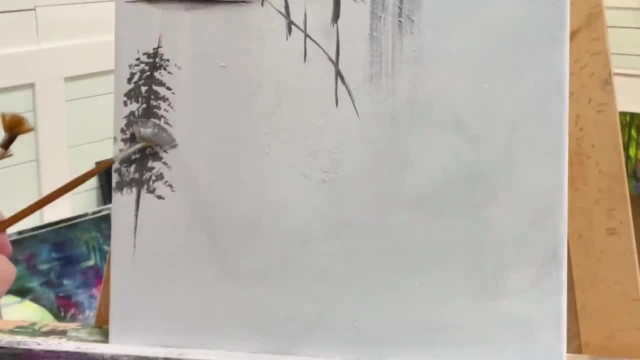 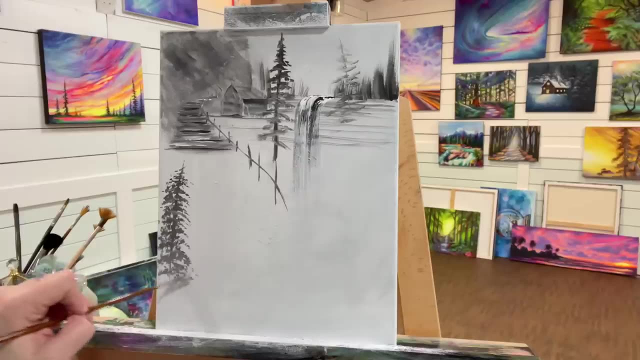 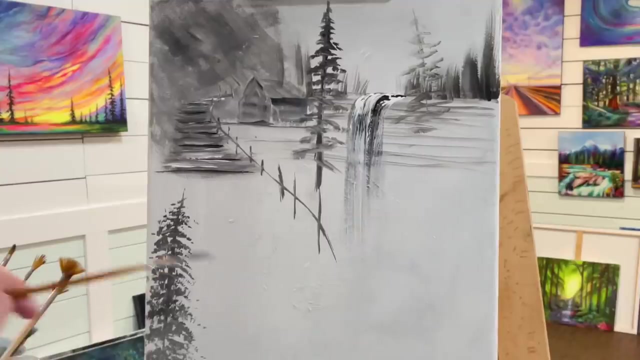 depending on what kind of fan brush you have. They don't all do that right away. They usually tend to do that when they have a lot of water. They'll separate. So you can see the difference in trees, The different texture you get. This is a little bit more fluffy, kind of messy. 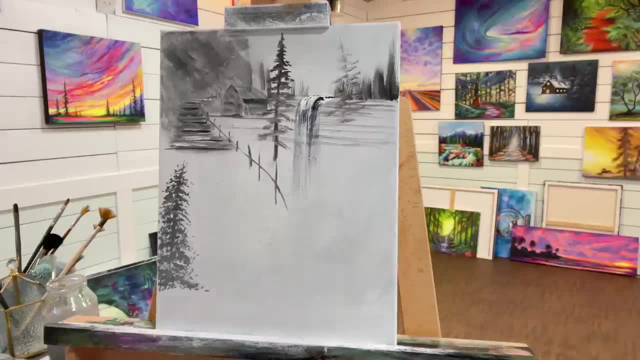 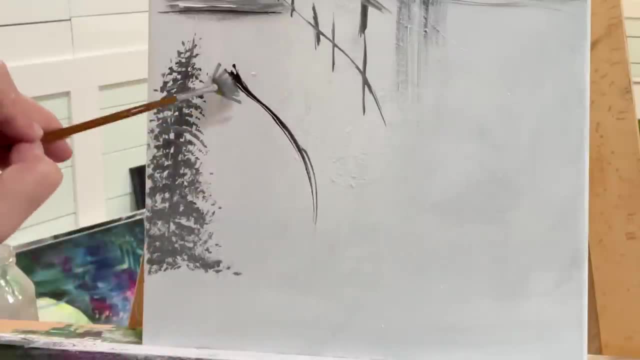 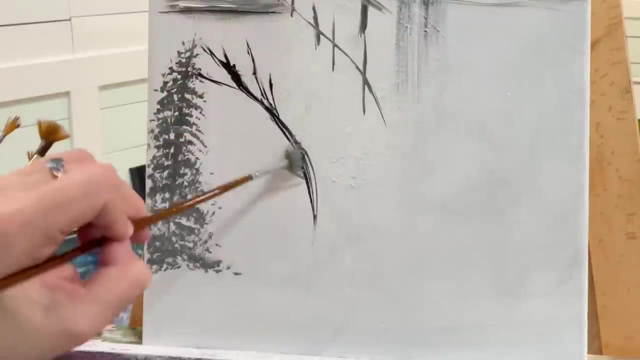 softer looking And you can also create more of a weeping willow kind of a tree. So I'm just using the very tip of my brush And I'm just going to add some little branches here And then I'm going to tap. 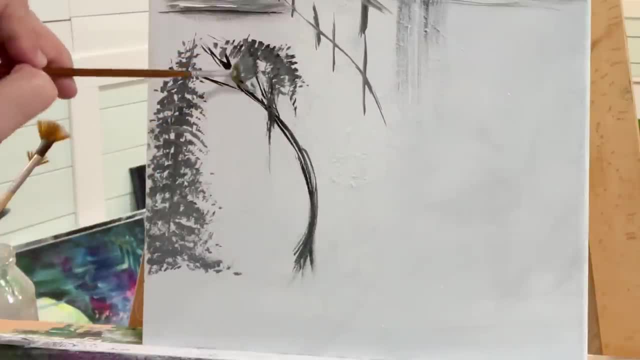 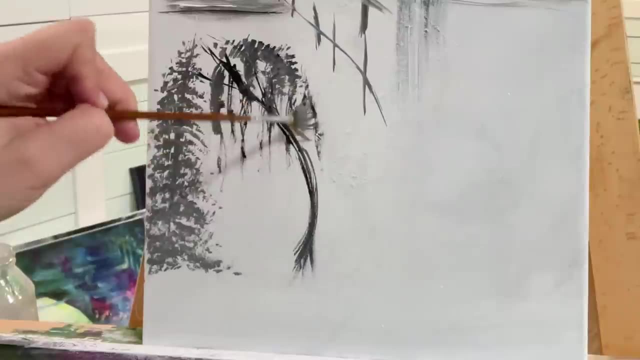 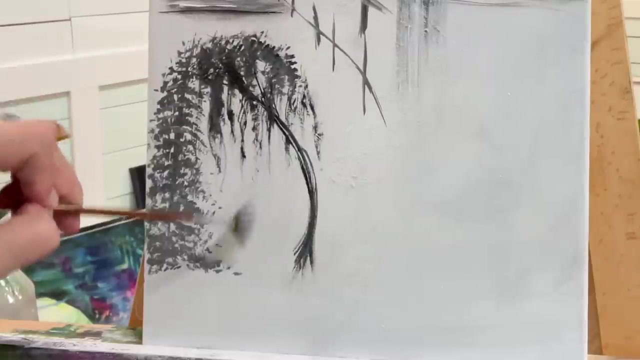 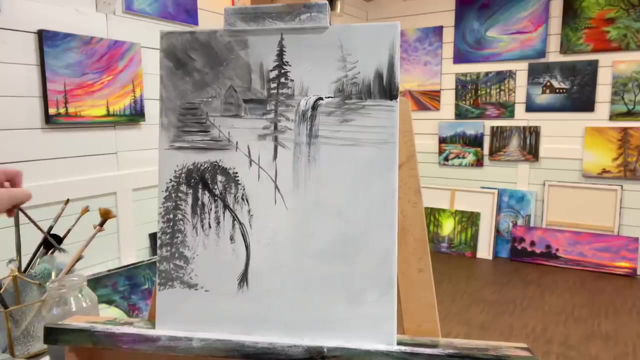 And then I'm going to turn my brush And I'm going to kind of tap, whittle and pull And this is just demonstrating how you would make the, how you could. This is just one way of making foliage on a weeping willow tree. We're kind of getting that vine type of a look And I'm going 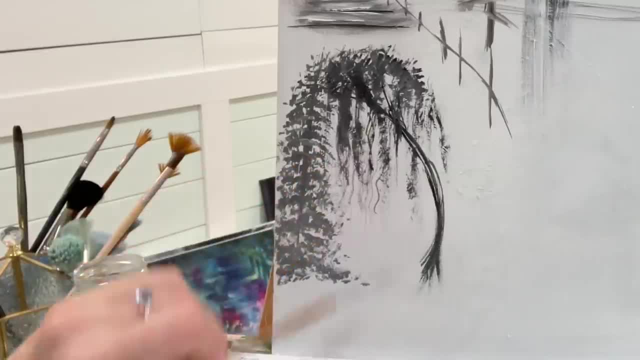 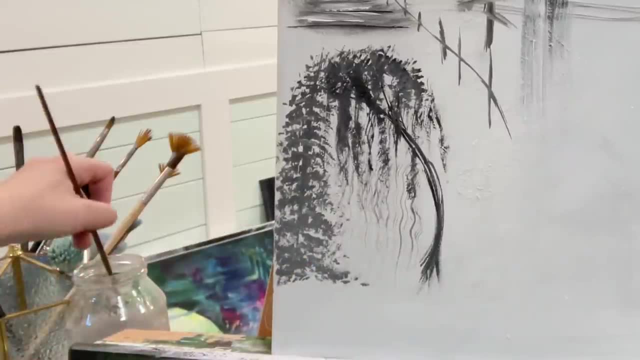 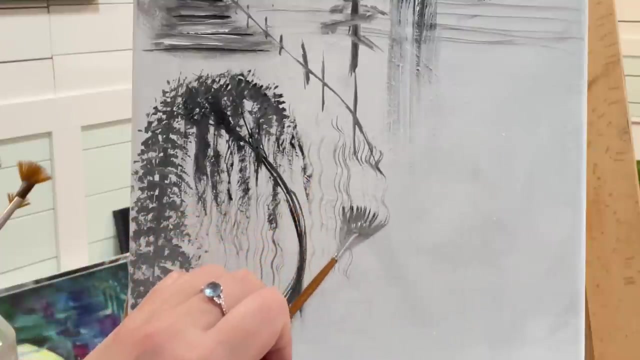 to get some water on my brush And you can kind of make these little squiggly, wiggly lines to take advantage of all those bristles kind of separating, Get a bit more water. So this here is what I'm doing here: creating these little ripples. It's really really. 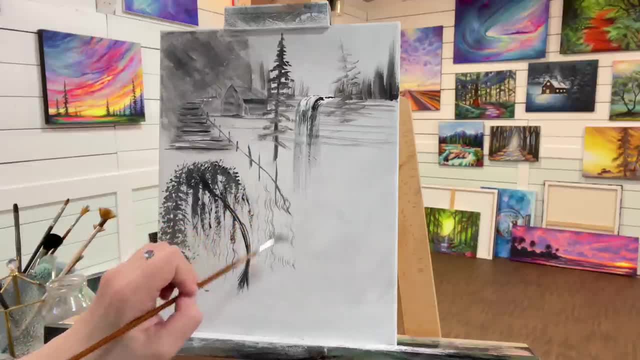 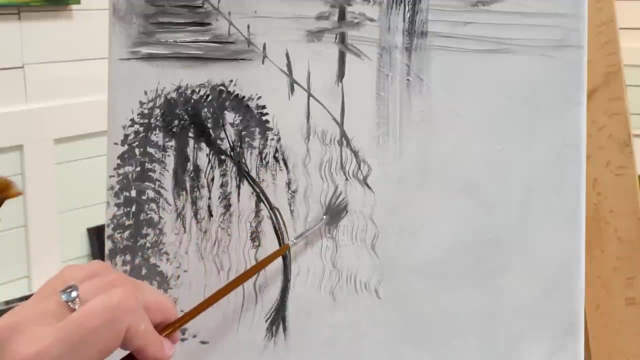 awesome for when you have that ripple reflective mirrored. look in the water Where you can see the reflection of the, say, we've got a dock above with a little post here, and in the water It's going to look a little wiggly from a bit of that movement, So you kind of can do that instant. 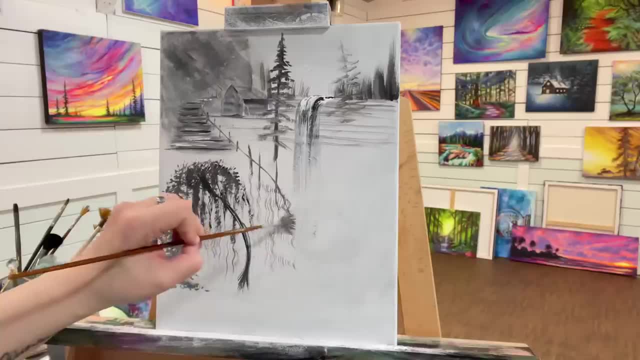 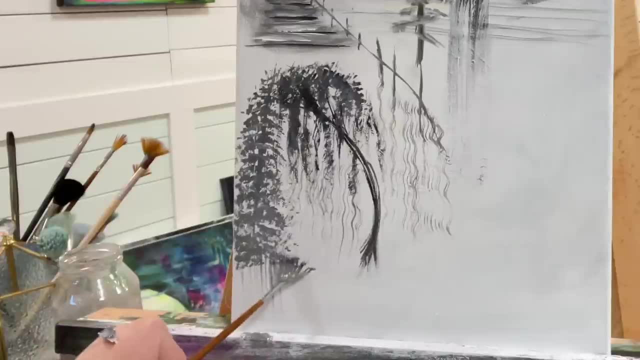 If you have a lot of them or just want to create some ripples, And the next thing you can do is pull straight down like this, with a bit of water. See how often I'm going back to the water to help blend. So that's what I like to do. 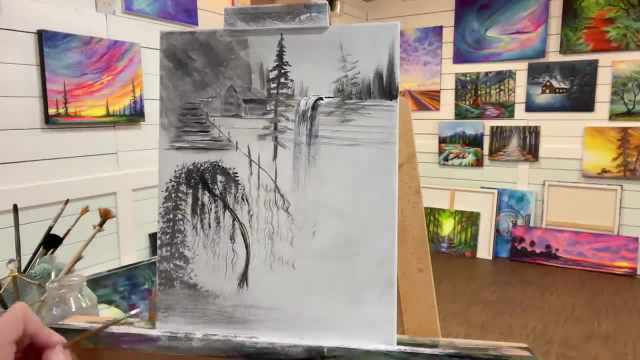 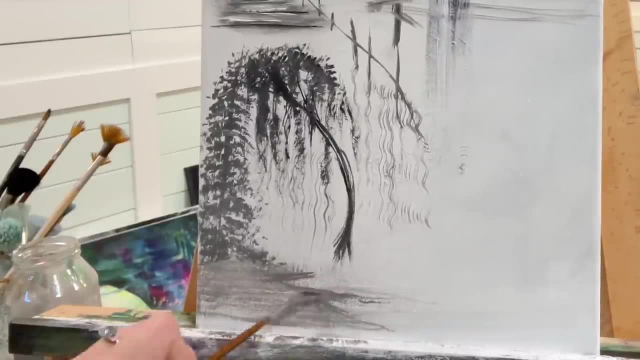 Is. use a water for blending my acrylics And you know, just kind of pulling and wiggling around, And you can create grass by using the fan brush too, especially when it separates and it looks like a rake. Just a little bit of water. 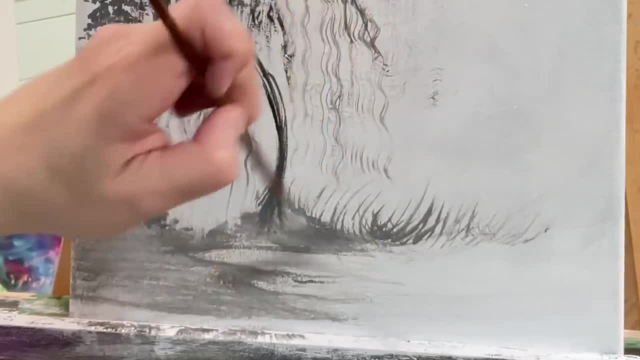 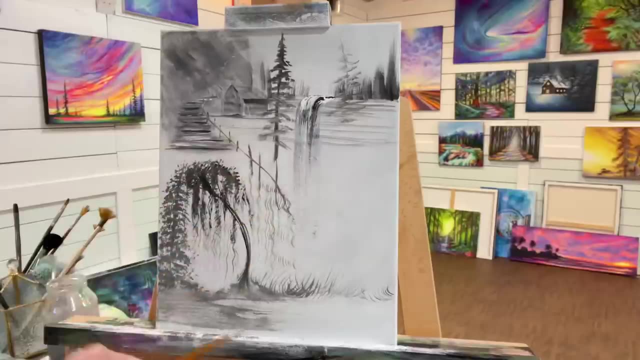 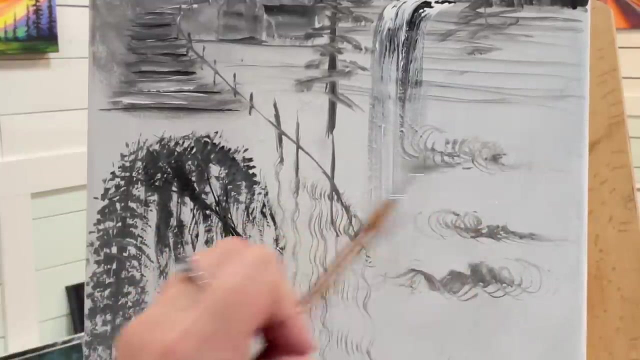 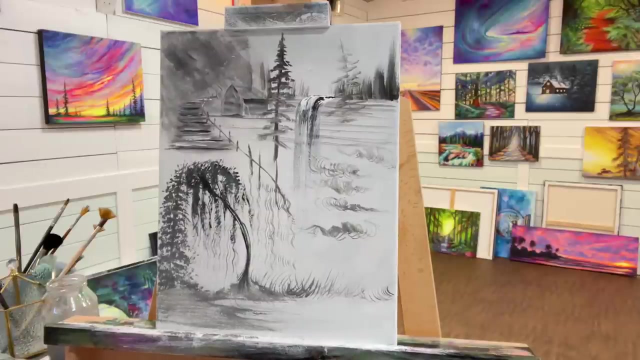 Just little pulls and flicks. Sometimes I like to make some whimsical looking clouds, So creating little scoops and circles and pulling and whisping off with my brush like that. And of course, the other thing that is wonderful is that you can use a little bit of water to get a little bit of depth. 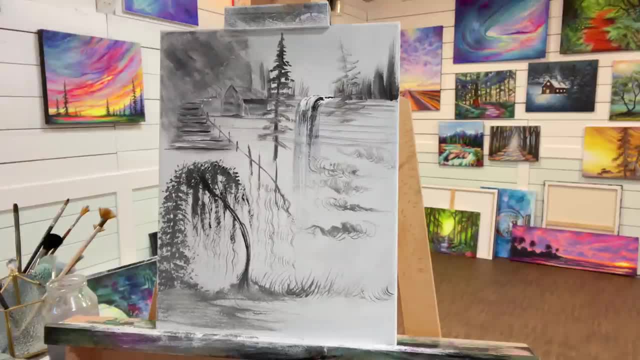 So that's what I like to do for a fan brush And that we all think of. well, this is what I always think of, And it's probably from watching Bob Ross when I was little. I couldn't wait. I think the first brush I wanted to get was a fan brush to create those waterfalls that he would create. 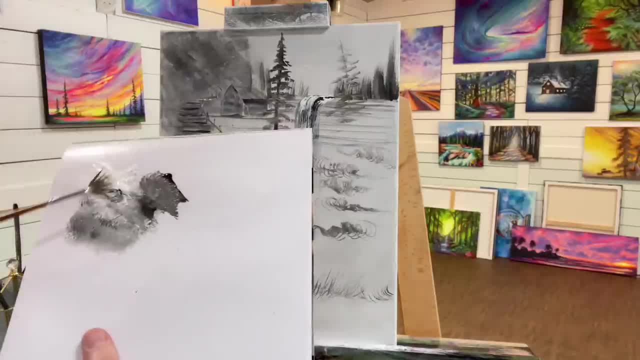 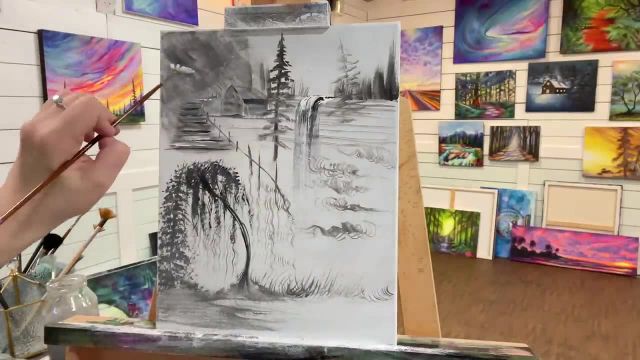 And he used a few other brushes, But the fan brush is a really fun one. So same technique as the flat brush, It's just going to look a little bit different. So already you can see, And if it bugs you, why not? 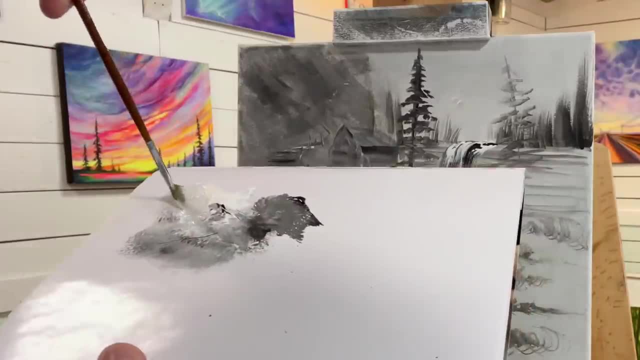 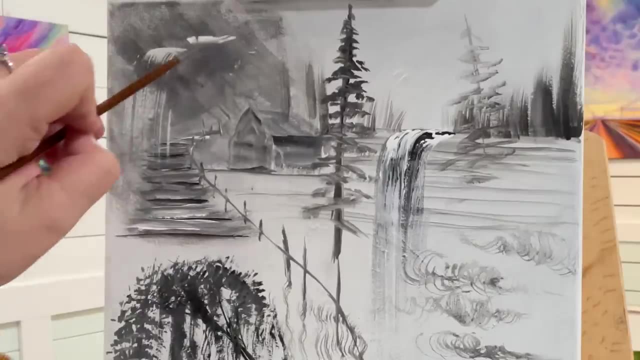 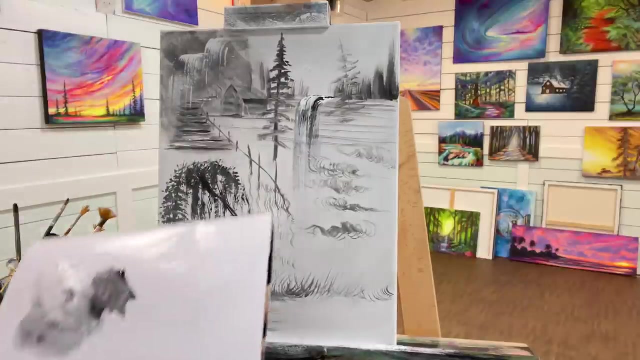 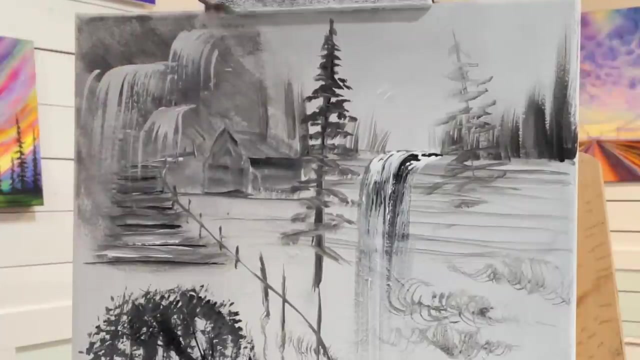 If it bugs you when your brush separates like that gently, like really gently, push and wiggle And they'll kind of go together again And then, yeah, same technique: Pull across and then curve And drop. Okay, guys, so those are all the ways that I like to use a fan brush. 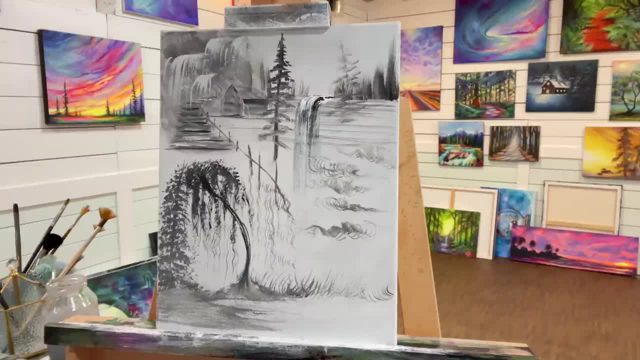 And maybe a few extra in there that you guys never thought about before or considered. So definitely include a fan brush in your supplies for painting. It's really, really useful. The next brush that I'm going to talk about and demonstrate is a filbert brush. 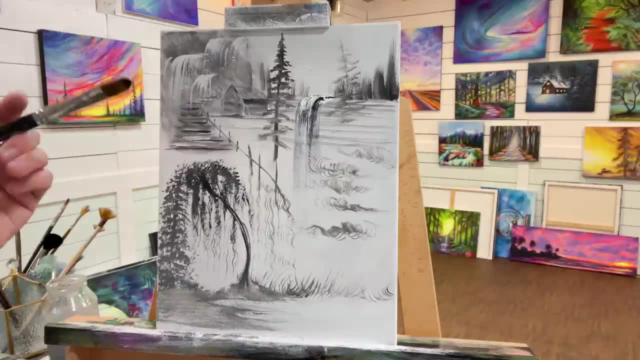 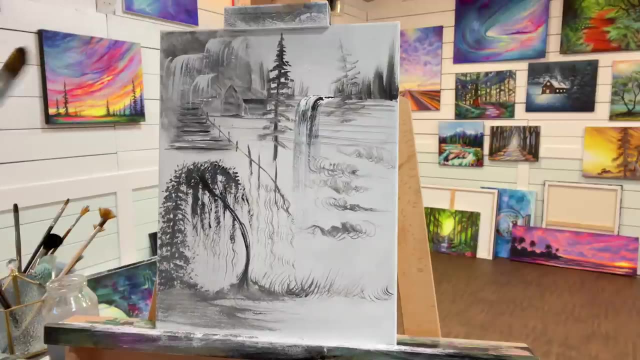 I've got quite a few different sizes of these. These are amazing. You could probably do an entire landscape just with using a filbert brush. So I'm going to show you first of all how I paint my trees with these, And these are my go-to brushes for painting trees. 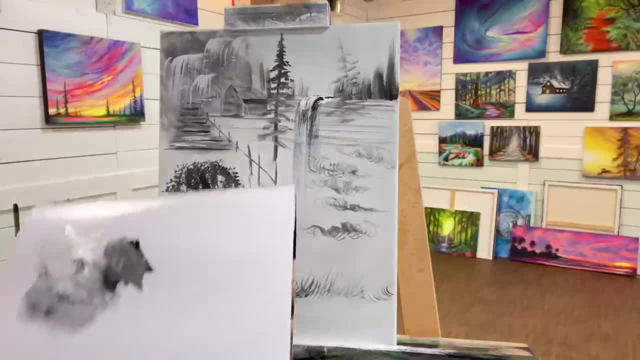 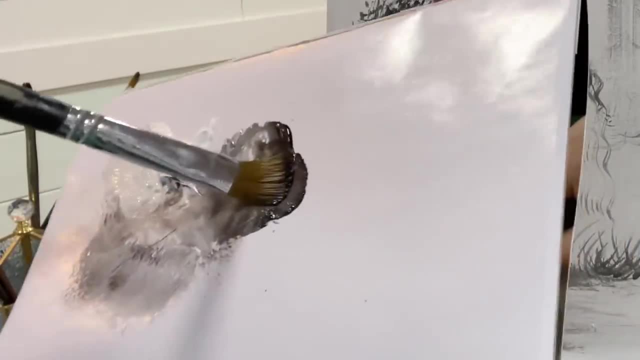 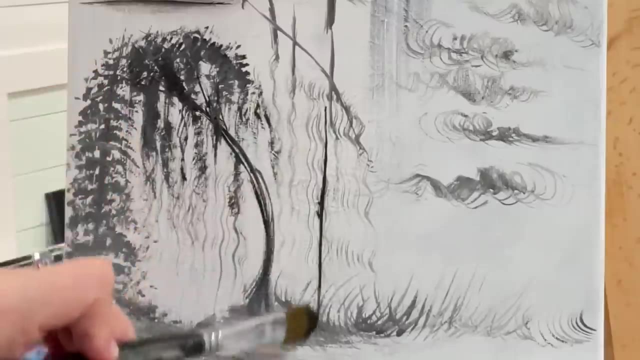 So I'm going to get my brush a little bit wet And I'm going to go into my black here. I like to push and wiggle and somewhat kind of push and fan it out, Manipulate that brush just a little bit And then I'll create a little tree trunk right here. 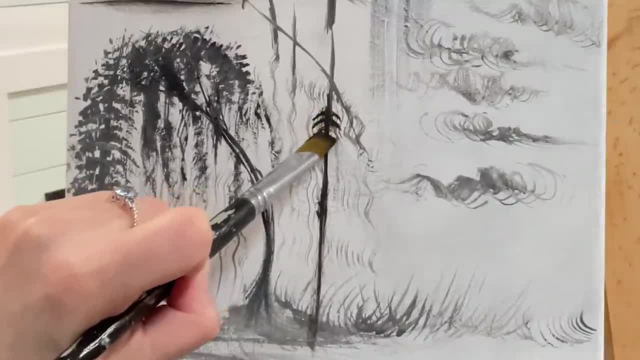 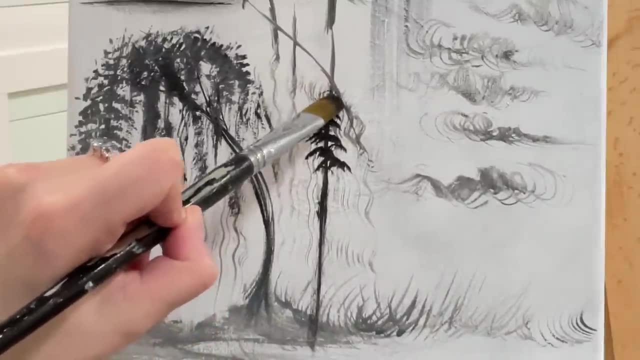 And then I'll create a little tree trunk right here And then I'm going to start with the top And I'm going to work side to side. Now, at first, when I'm doing the top of my tree, I'm hardly using any pressure or any part of the brush. 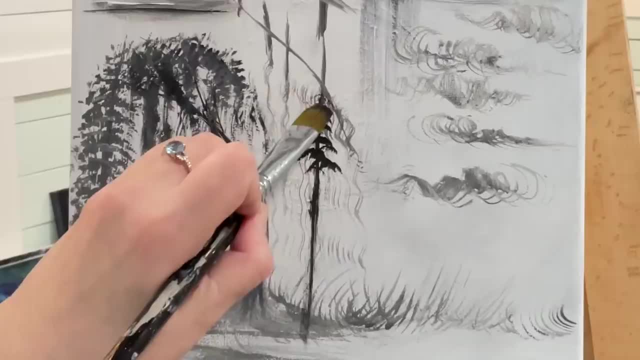 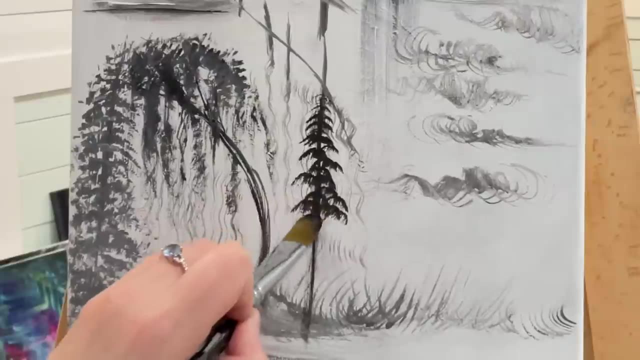 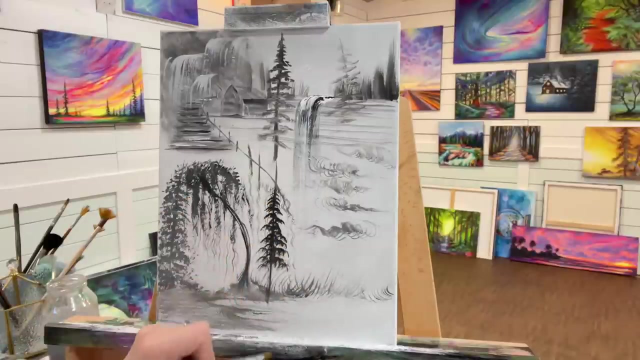 Just the very middle section of the brush on the tip And then, as we get towards the center of the tree, as we go down, it's going to be a lot bigger. But stay away from creating a big fat triangle. right It starts to get wider. 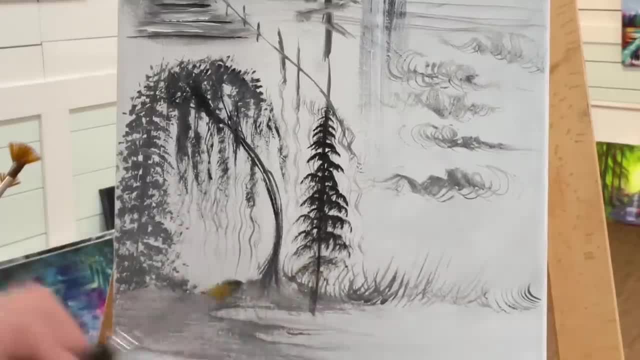 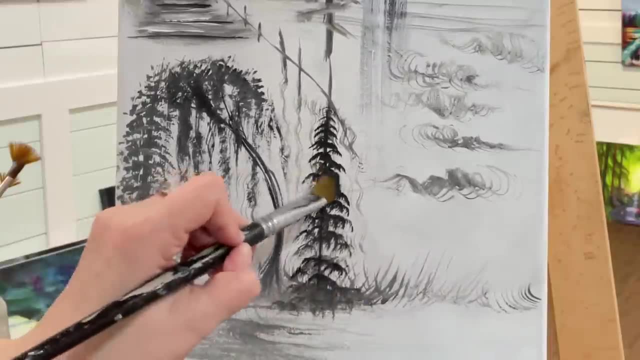 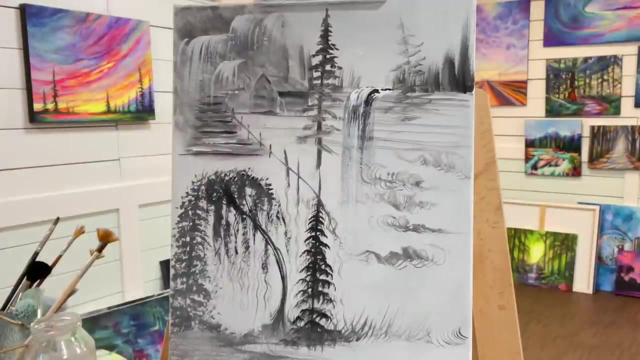 But then it just sort of balances out here at the bottom. So that's one of the biggest mistakes that I see beginners make with their trees: They get carried away and end up making a sort of a pyramid shaped tree. So out of all these trees and the three brushes that I used, I just prefer- and it's just it's personal preference. 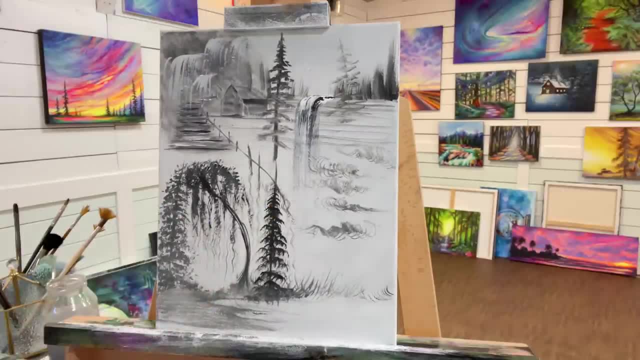 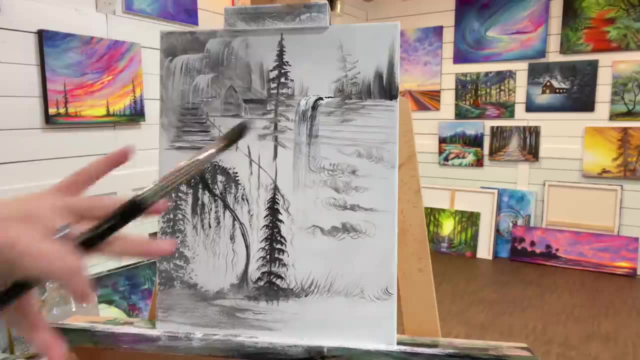 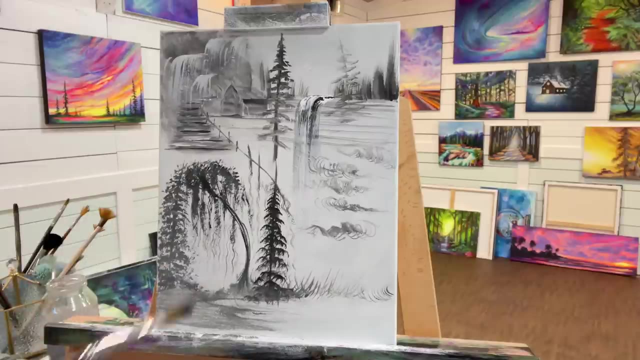 Everybody has different ways and likes or dislikes of trees and what trees they like And brushes to use, But this is my favorite. I just love the way they look like they're bowing over on the edge And especially for winter paintings it helps to create that snow heavy branch weighed down by a snow look. 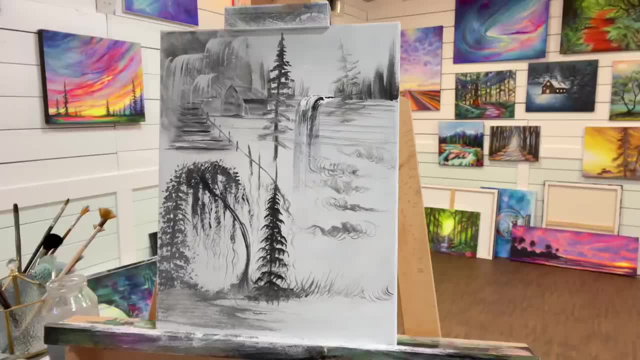 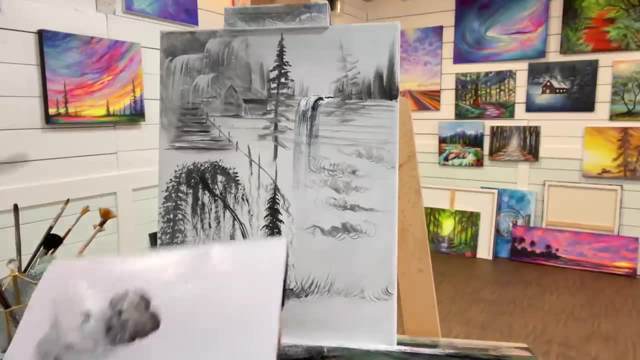 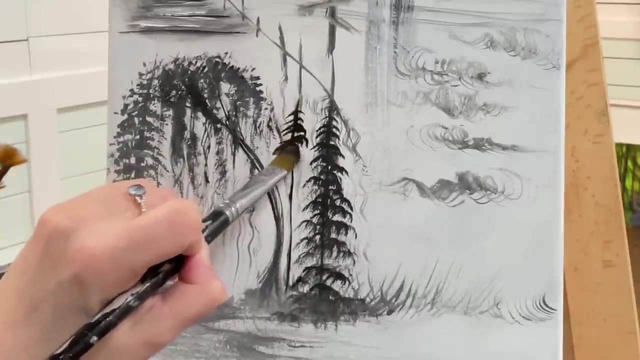 That adds a lot of character to a winter painting. So I really, really love this brush for that, And these are fun to paint And I've got leftover paint so I'm going to paint another one here. I learn a lot by repetition, so I'll demonstrate another one here. 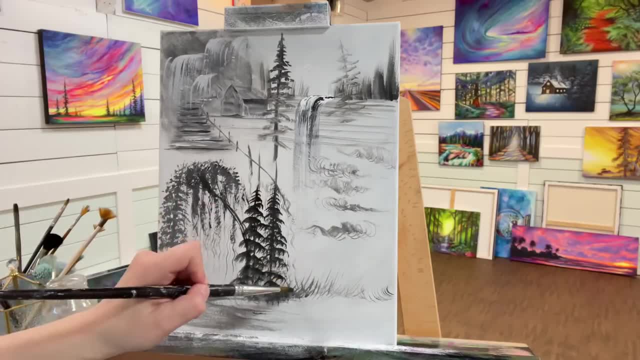 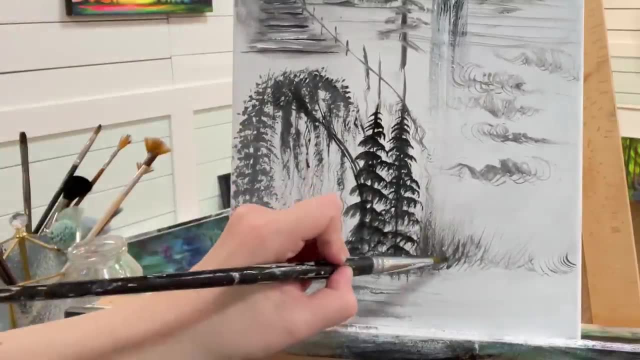 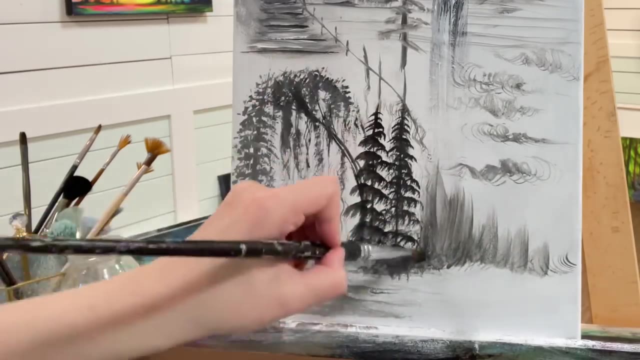 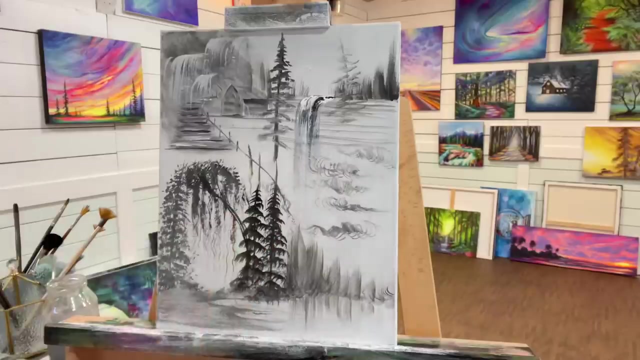 And you can also use this brush for the same technique. there, I just need to get a little bit of water in my brush: Press, pull and flick. Okay, A little bit of water if you want that reflection, And then for foliage it's a great brush. 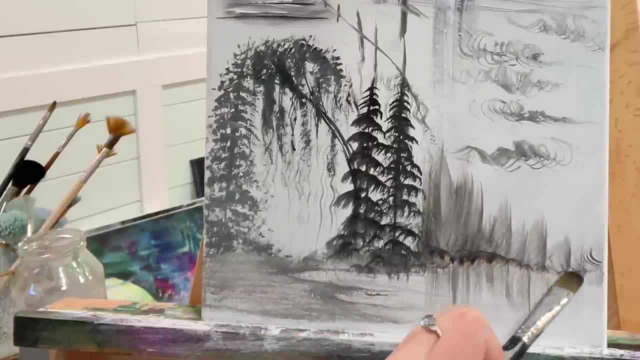 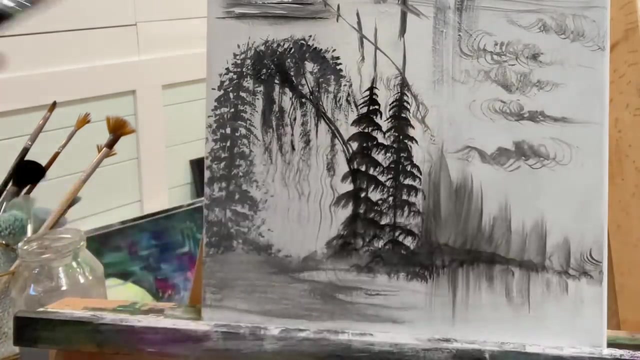 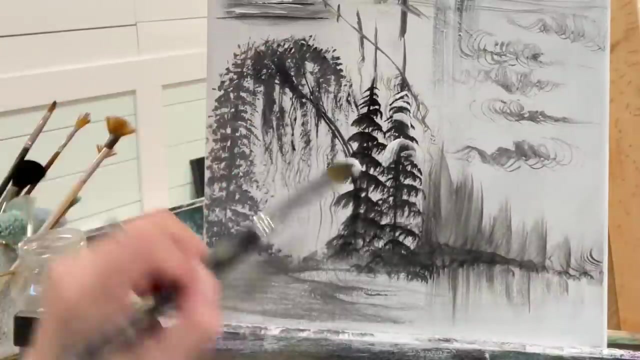 Tapping in and making it look like moss. So when you push you can make it look more fluffy and bigger And then let off using the tip And it looks farther away. You can highlight right away. So yeah, if you want to do some snow. 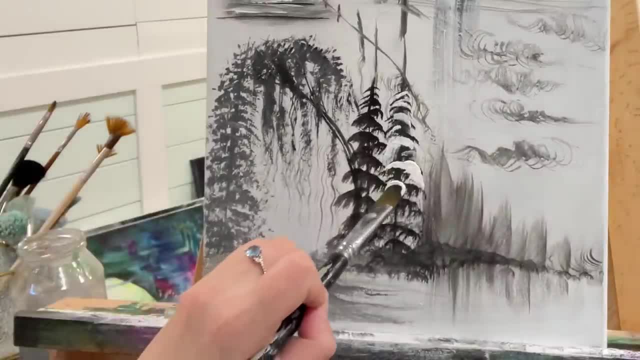 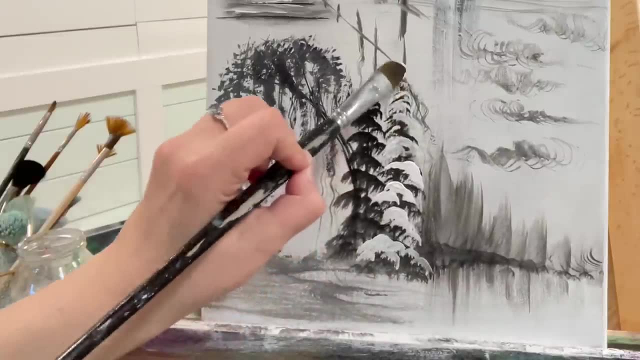 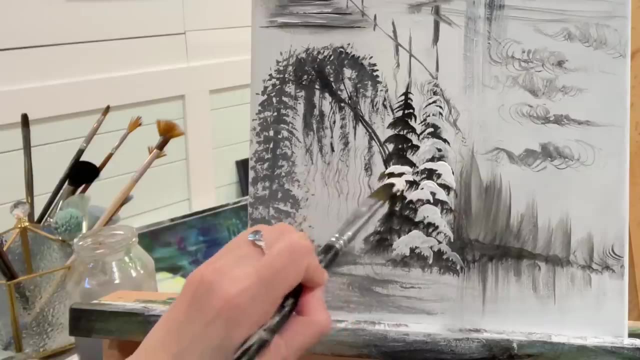 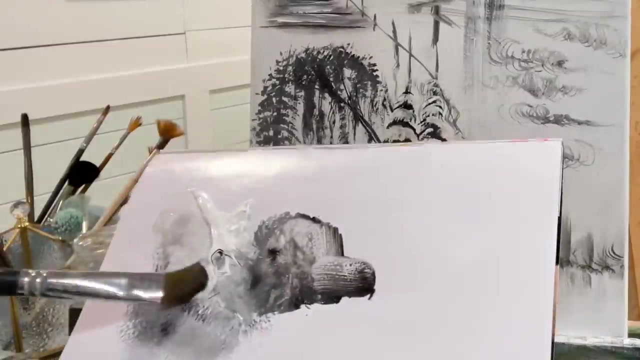 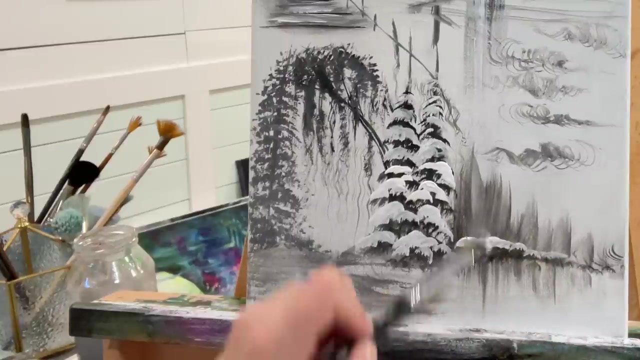 I've got a whole playlist on winter paintings. You just get that really snow covered tree. look Where it's just hanging over the edge And it's really weighed down. I love that look. So you can add that highlight And you can even with that background that we've got. 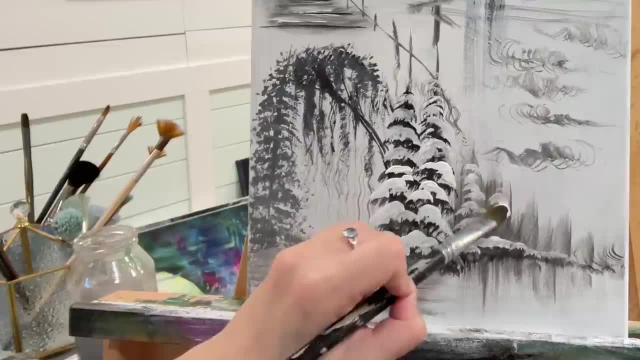 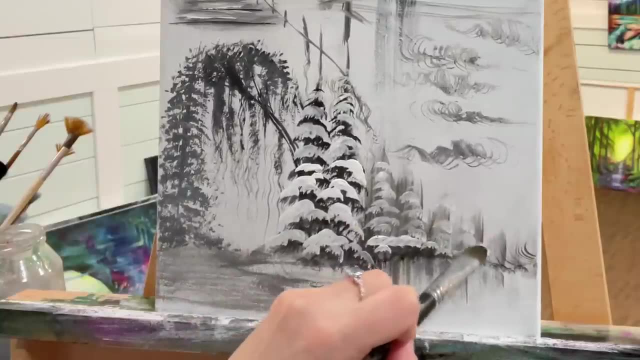 We can come in just with white, Just tapping a little bit like that And it looks nice And instantly making some snow covered trees Makes for a really nice background. You can do a little tap down in the bottom To indicate a reflection there. 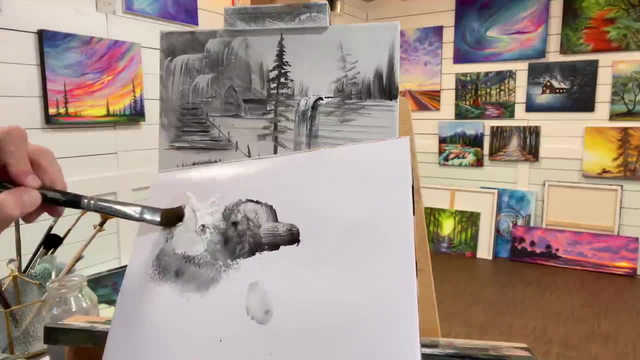 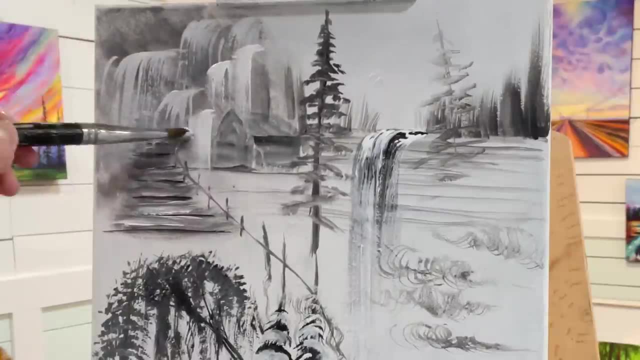 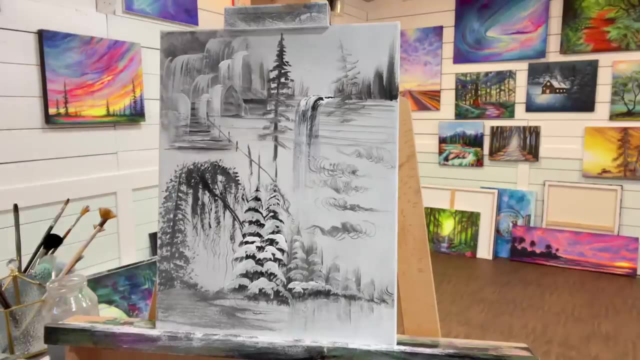 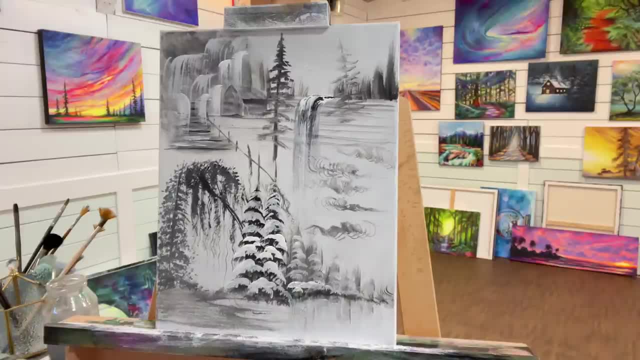 Using this brush, Using this brush. So there you go, guys. There's quite a few brush techniques For you using a few of my must have brushes, For you using a few of my must have brushes. I will quickly go over. 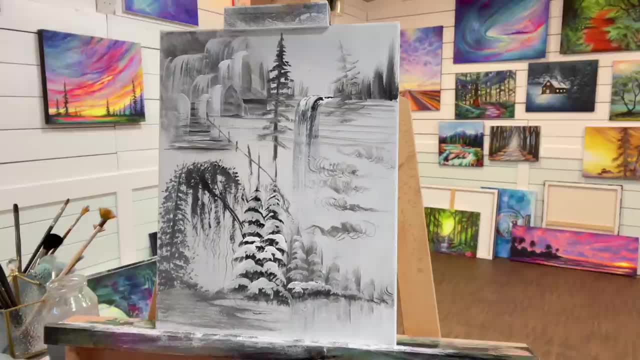 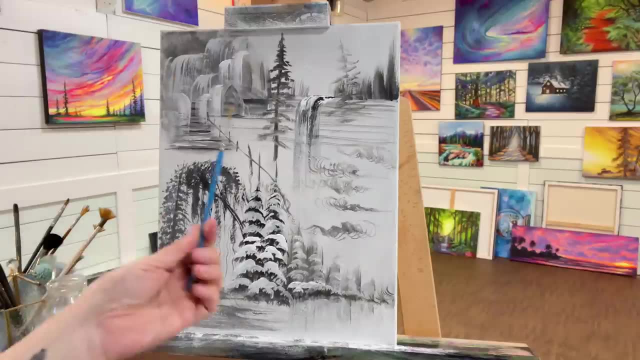 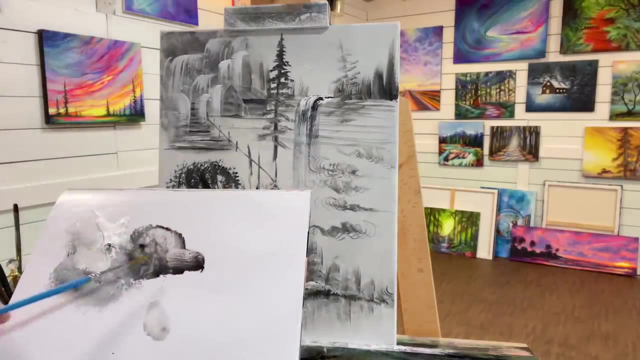 I wasn't going to add the liner brush, But I'm going to show you guys a few things with the liner brush- probably my opinion and experience of teaching for over 20 years- the most hated brush for beginners. the trick and the key of the liner brush is to make sure that you have enough water. 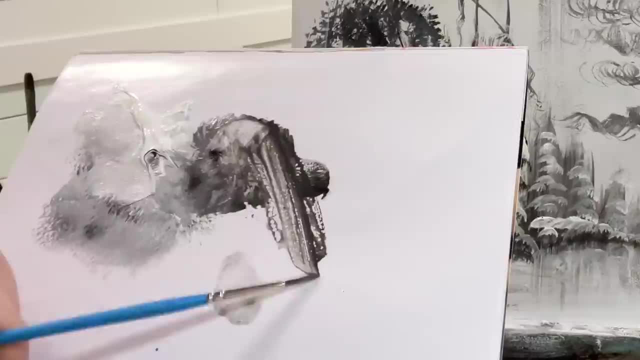 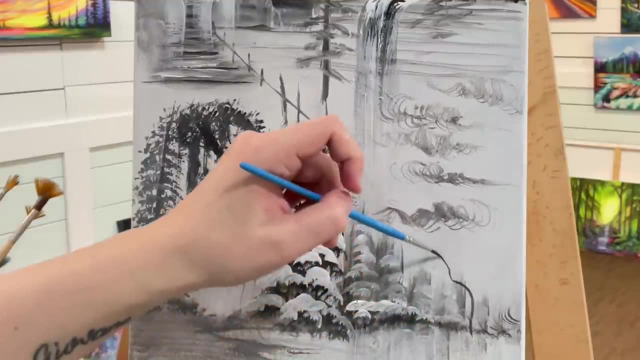 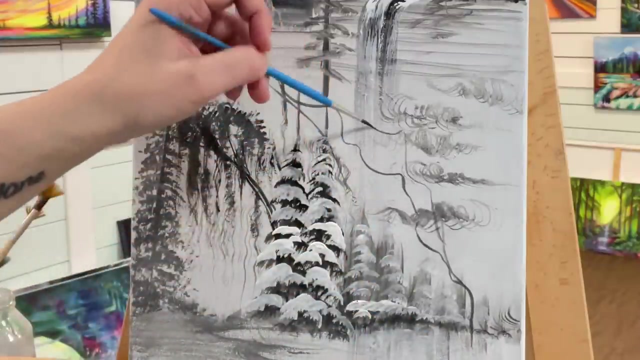 so oftentimes students go for more paint if it's running out of their brush. they think they need more paint, but what you need is more water. so when you have water, look how easily and effortlessly- and i'm just twisting lightly and pulling and wiggling with my brush to create little branches- 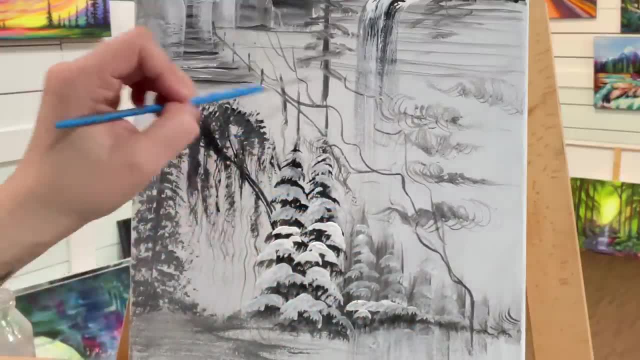 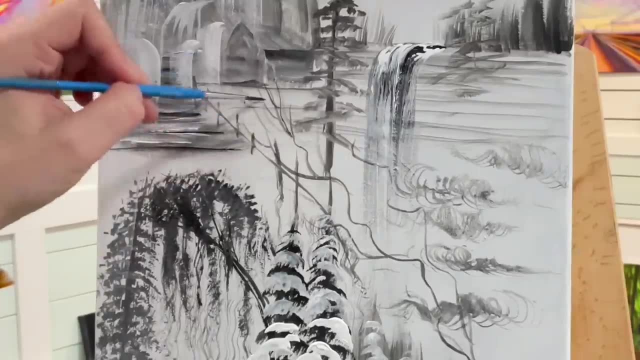 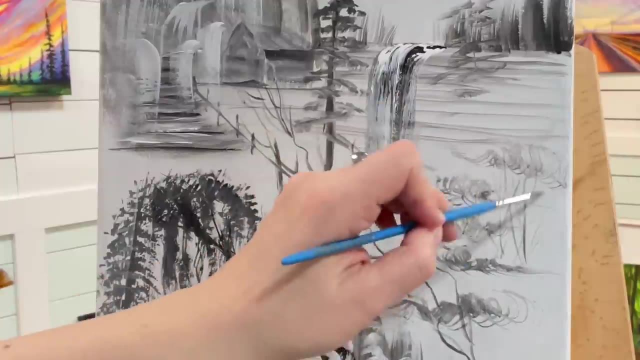 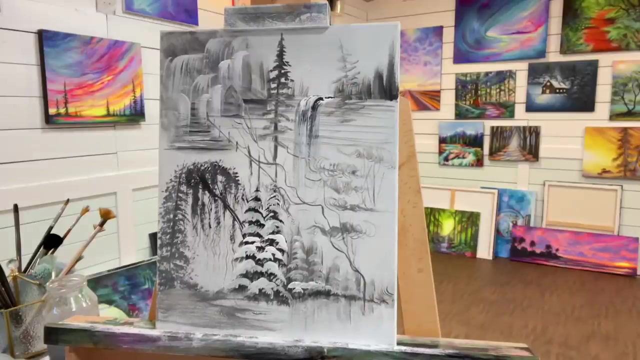 and this is why i love to use the liner brush, because i love the very delicate branches that i get let off. it's very wispy looking and, of course, a liner brush is excellent for any small, tiny details, fine details that you have in a painting. depending on what you're working on, you could use them for. 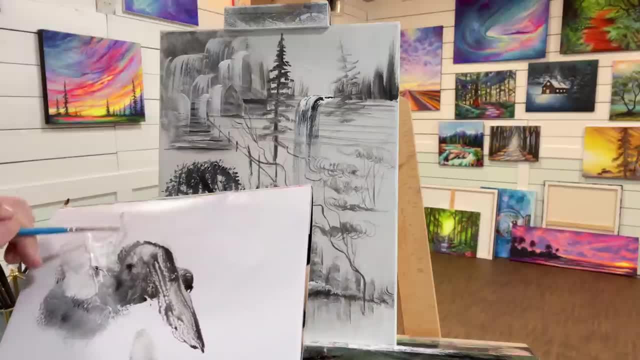 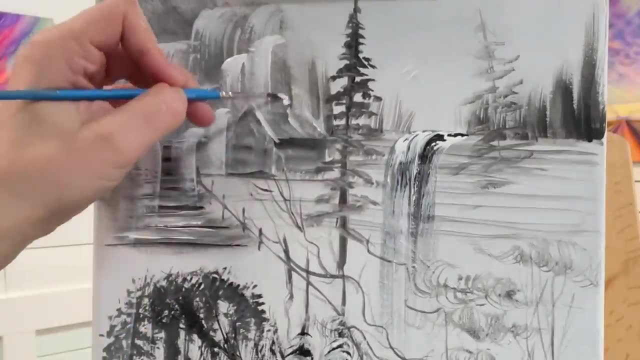 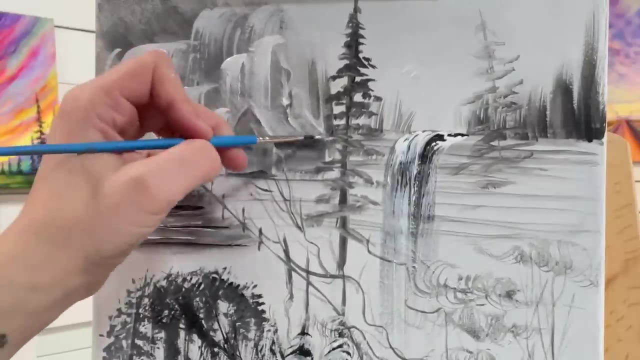 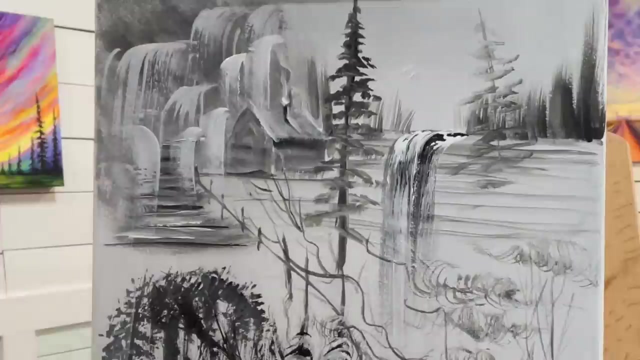 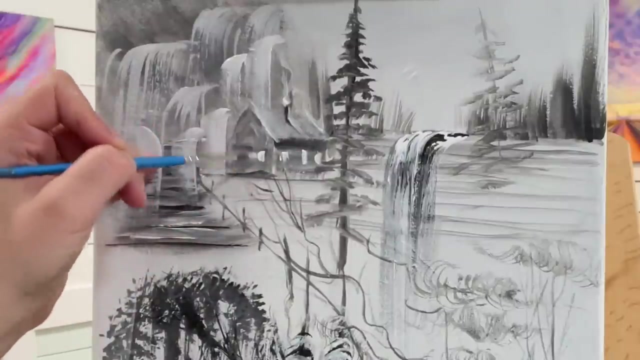 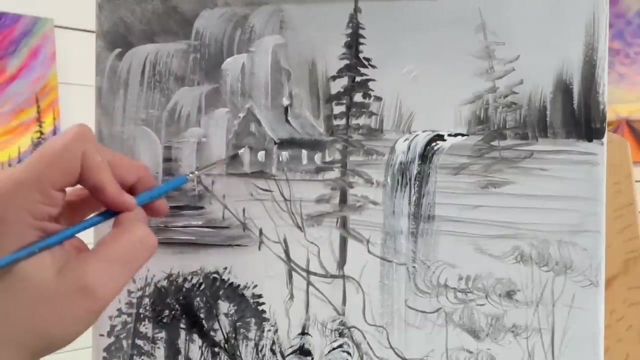 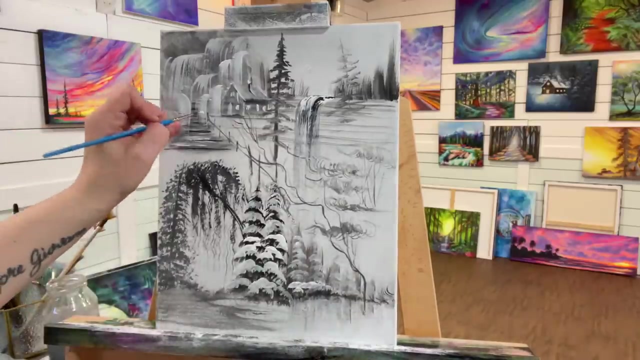 i'll just take a little bit of my white here, so if i wanted to have a little chimney or a little window. this brush is nice and small that i can just add a few little dabs here. dab, dab, dab, and i use it sometimes for painting. 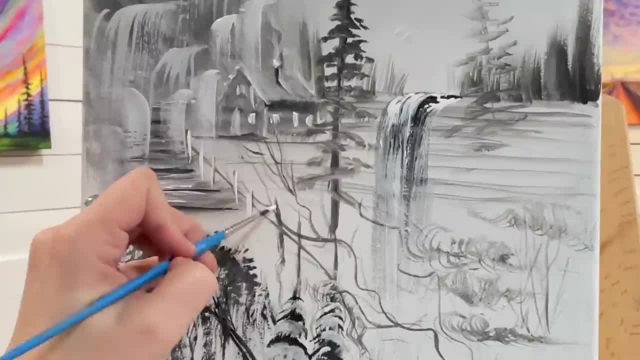 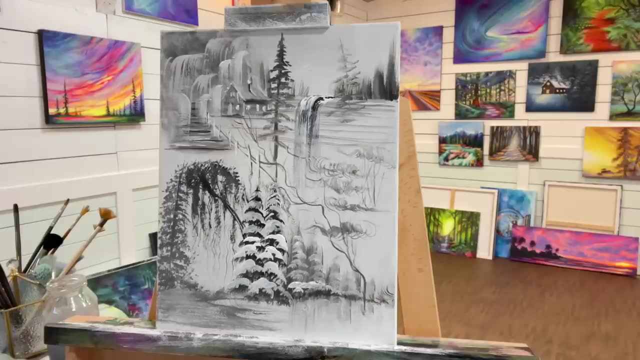 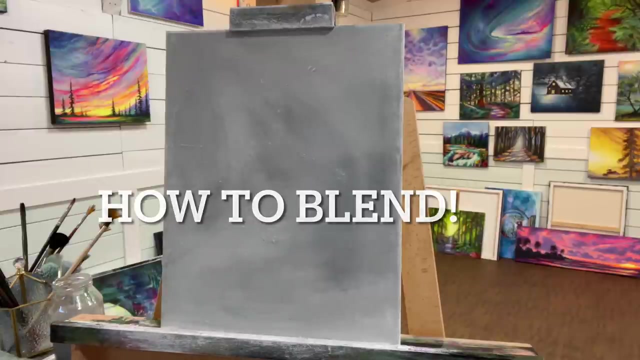 fence posts too, so it's really important to have a few different brushes in order to paint all the different things that you might need to in your painting. okay, guys, so now i'm going to go into how to blend your acrylics more easily. so a lot. 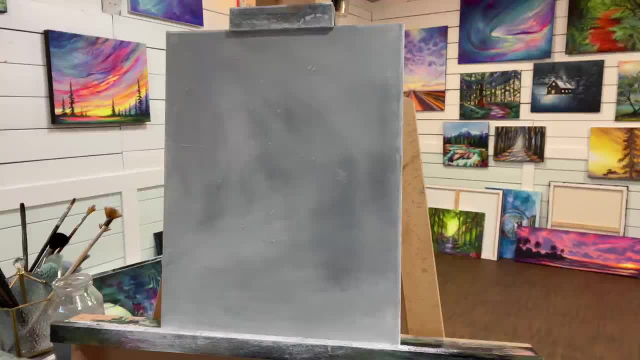 of people, when they're just beginning, have a really hard time with the blending, simply say, ah well, it doesn't matter. composites are recording my painting process, and that i'm thinking because i have no Amarus kind of acrylic. that's what want to do. i want to kind of create a sort of yellow actinic. 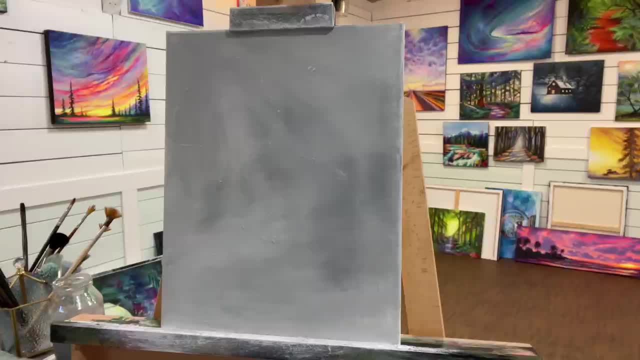 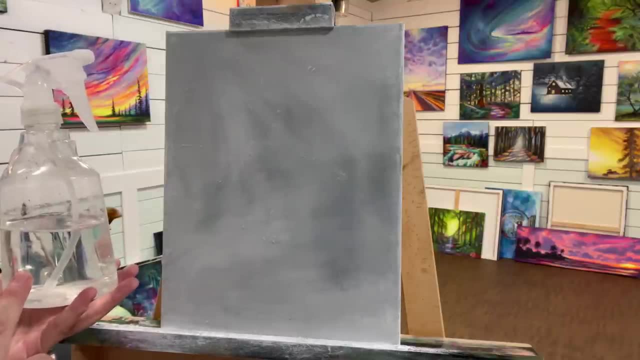 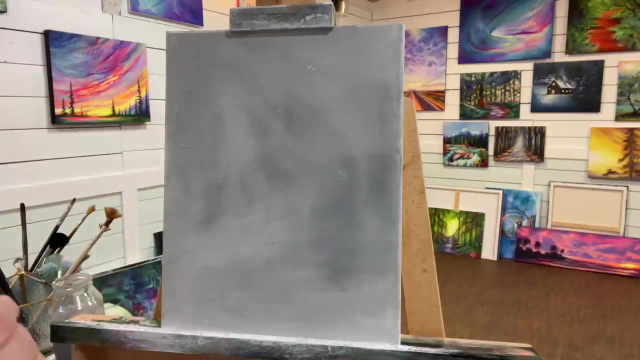 to do Michael B time with them drying too fast. there's a few different things you can do, so i talk about this: a lot water, uh, misting with a water bottle. so to create, if you're going to work on a background, say, you want to cover up a background, so you'll just lightly mist and i've got a little bit of bubbles. 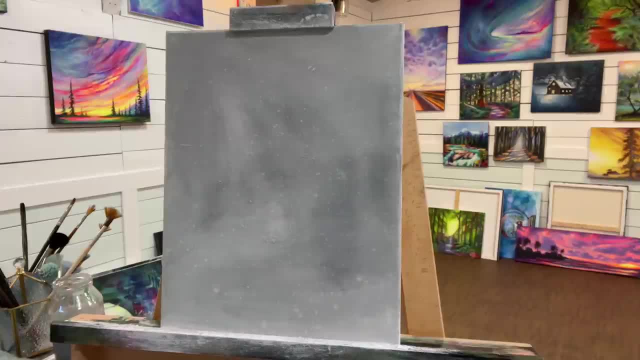 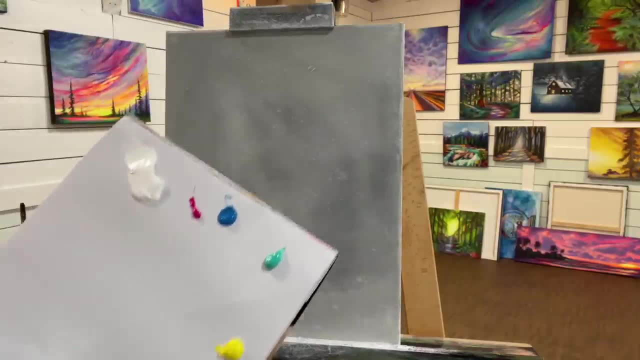 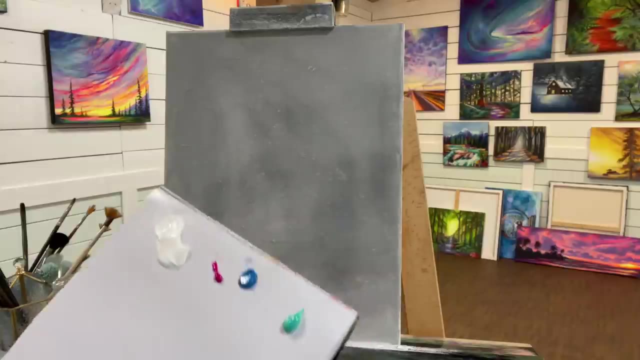 in there lightly mist the background. you can also mist your palette every so often, maybe every, depending on how quickly it's drying out. keep in mind, you'll be able to blend your acrylics a lot easier if you have the temperature cool in your studio and it's not so hot, so that will keep your 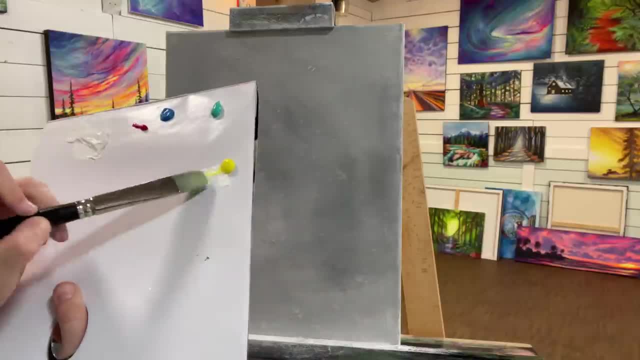 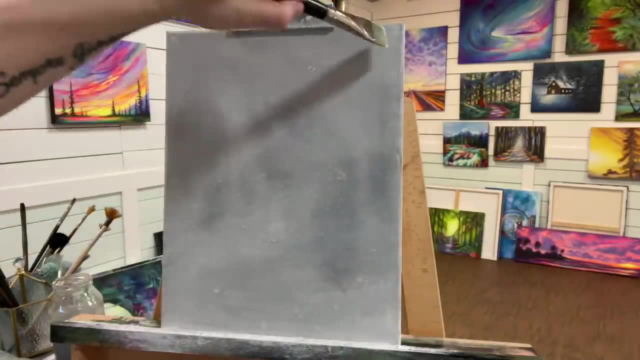 acrylics from drying out too fast. but what i want to do first is take a bit of white with yellow. i've got cadmium yellow cool here. it's like a lemon yellow and i'm just going to start adding this on the background. i'm going to work on 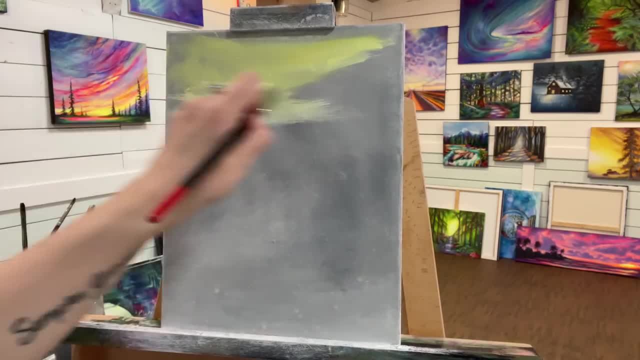 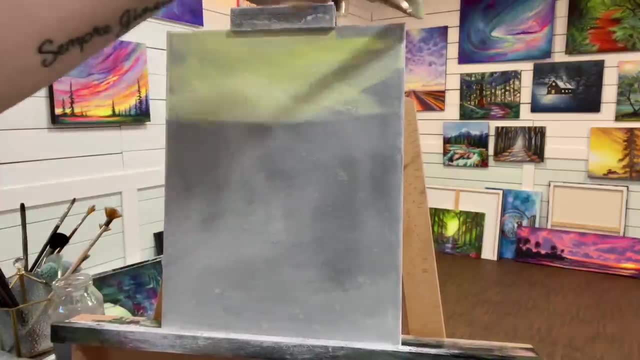 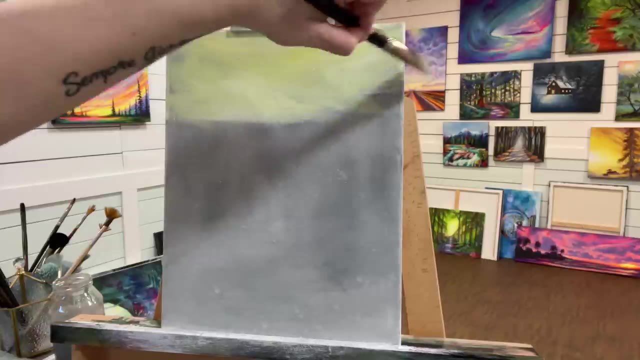 the sky and i'm going to work my way up to sort of a tropical seascape for you guys and show you how to blend, and i'm just kind of doing a crisscross method here. i'm working on a light gray background under painting here, just because i really like the way colors look on a soft gray. 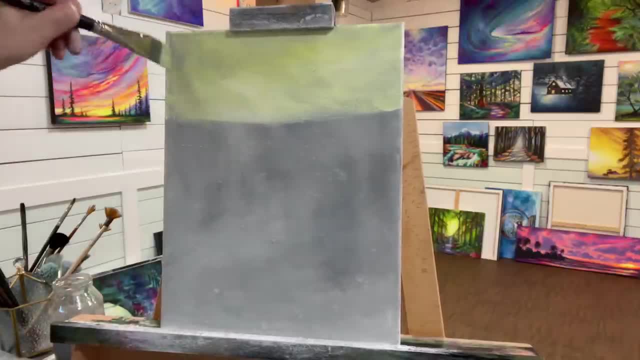 background. so it's still a little bit dry. i'm not able to blend right there. so if i pick up a little bit of white, i'm going to work my way up to sort of a tropical seascape for you guys and quickly work the two together. so water is your friend. there's other things you can use. 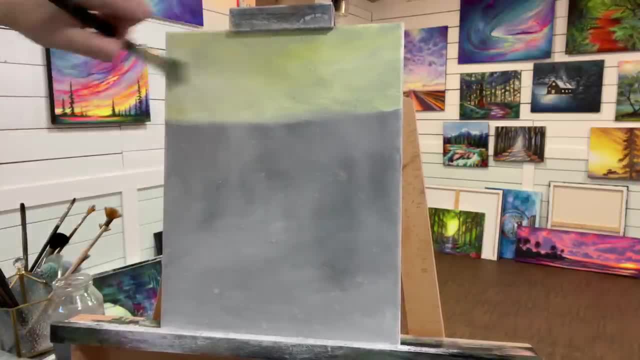 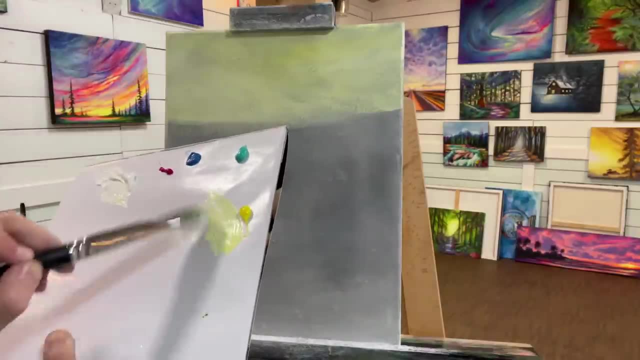 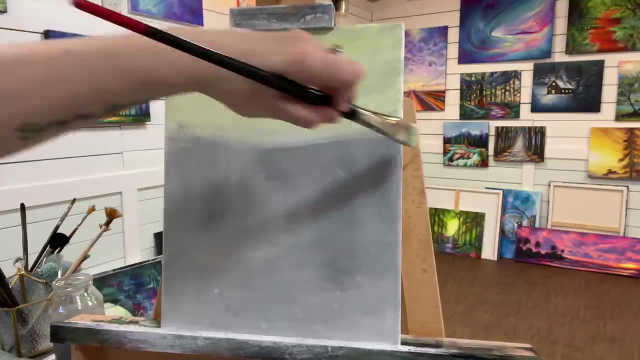 to make your acrylics blend a little bit better. if you don't want to use water, there's definitely other mediums out there, but in this video i'm just showing you how to do it on a budget with water. so what i like to do is just going to work this out of my brush. 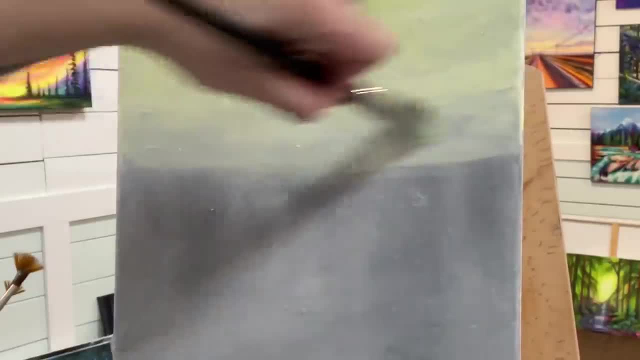 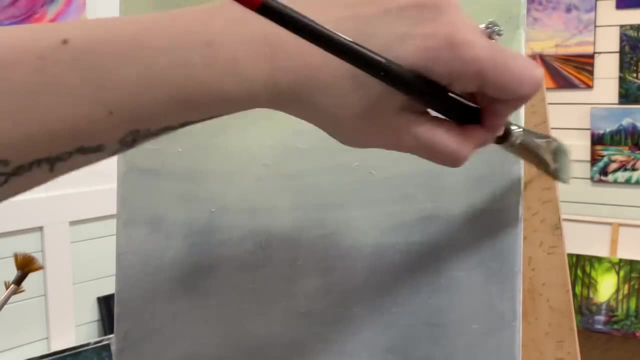 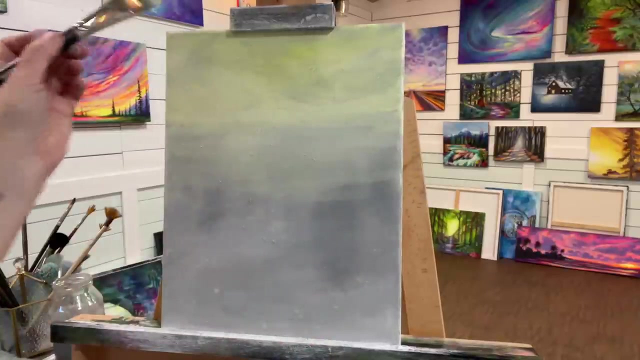 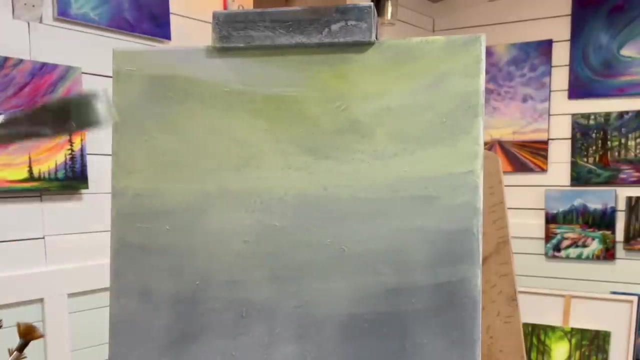 making it thinner by adding more water each time as i go down, so you can see how much water you add. depending on how much water you add, it's going to thin that paint out. it's going to. so no water at all, just complete straight paint. it's going to be thick and then more water. 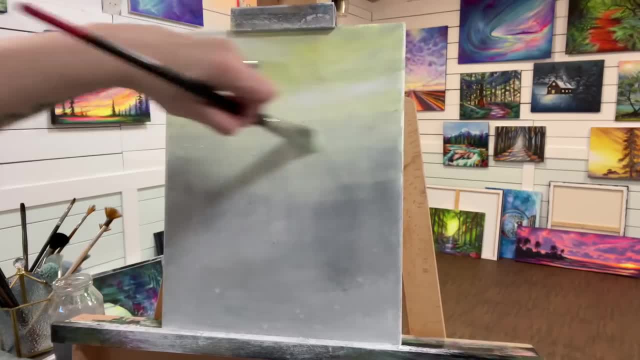 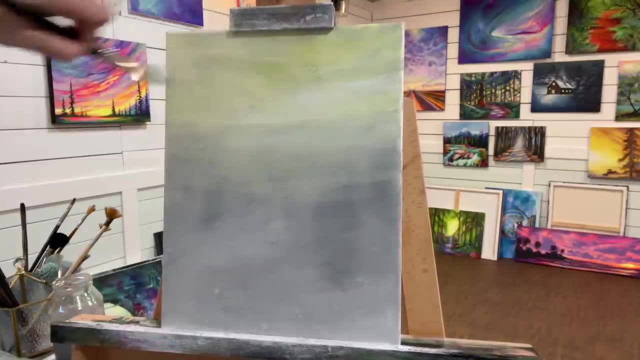 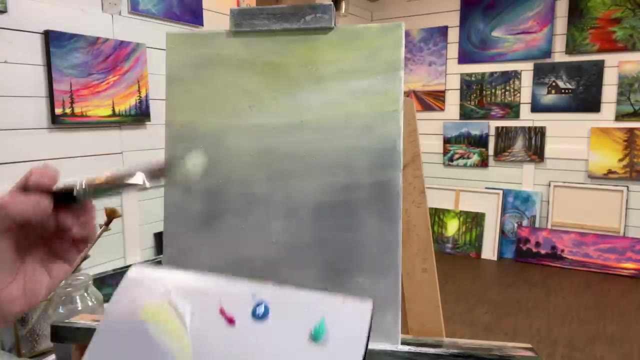 it's going to thin that paint out and eventually make it transparent. so keep that in mind. unless you want it to be transparent, don't use too much water. okay, so now i'm going to blend and make a soft turquoisey color. i'm going to get a little bit. 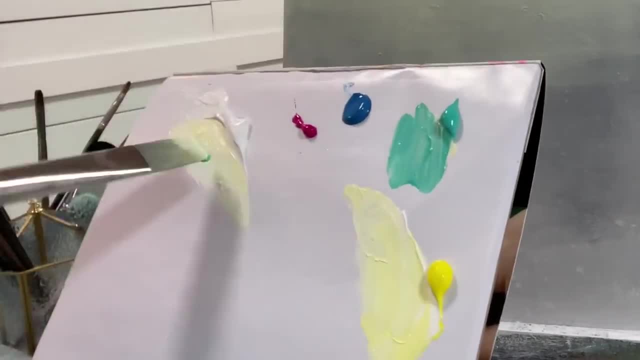 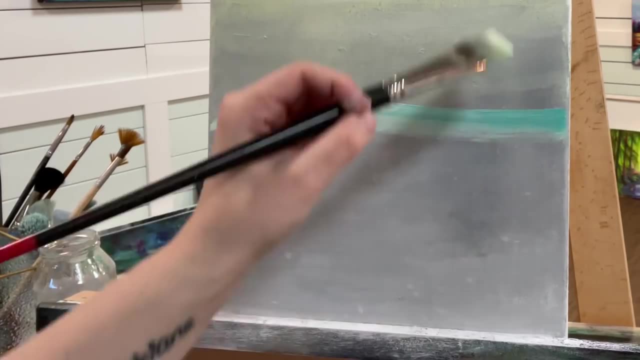 of water on my brush with that white, the yellow and the turquoise and i'm going to just have it all on my brush like that and i'm going to start pulling. we'll just put the horizon right in here. i'm going to push and pull nice long strokes. 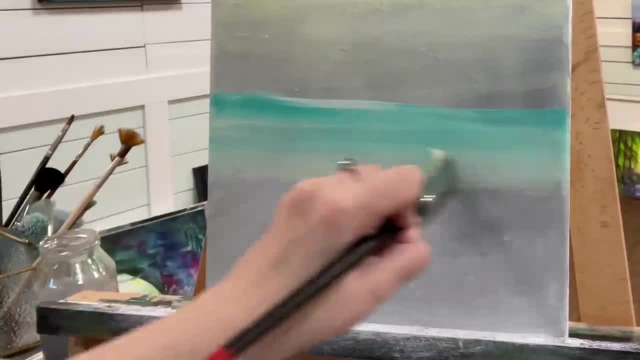 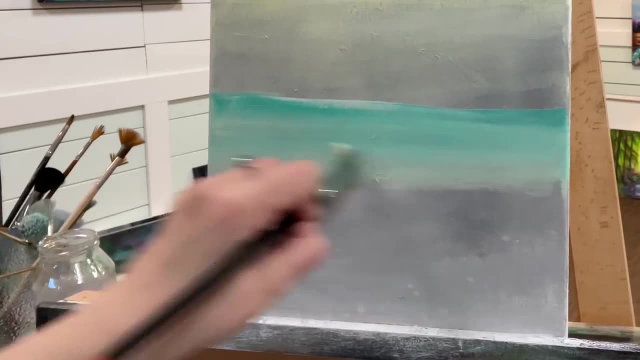 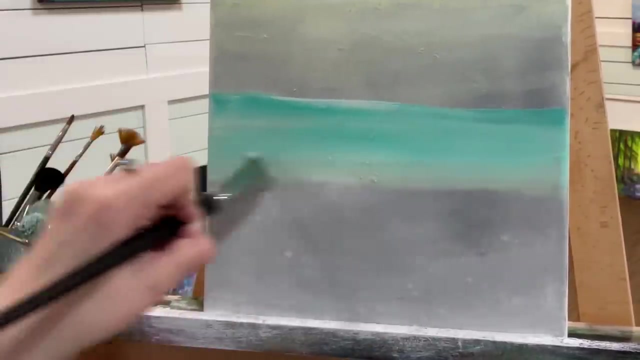 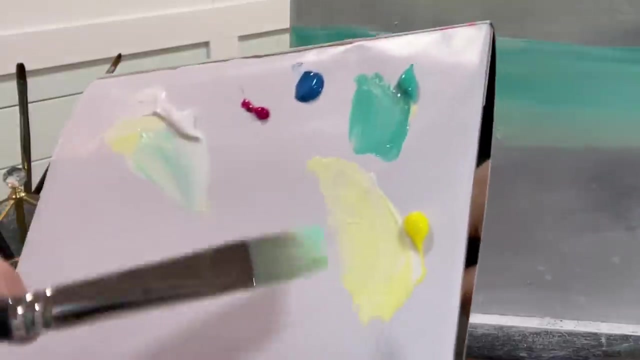 blending them all into one another. so each time i pull my brush i'm blending in to the previous stroke. that will make it more seamless if you want a really smooth blended look. it gives it that creamy kind of a look. that's really pretty, and then i'll make it a little bit lighter here. 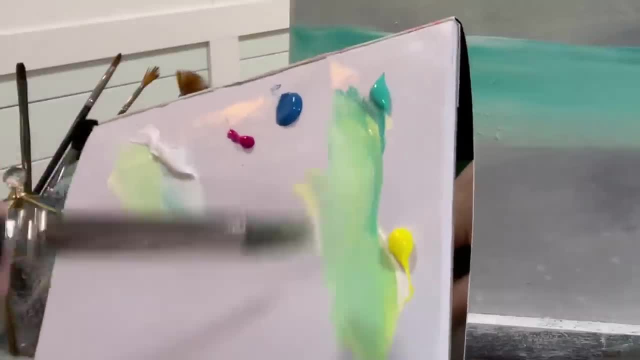 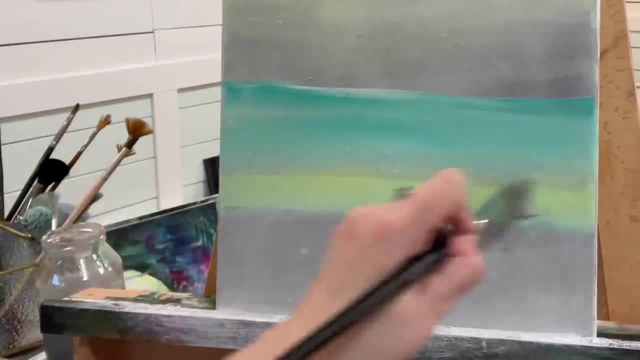 so i'm going to blend the yellow, white, less turquoise, and i'm going to start right below where i left off, but then i'm going to work my way up. now, to do this, the paint has to be wet still, so you want to have enough water. 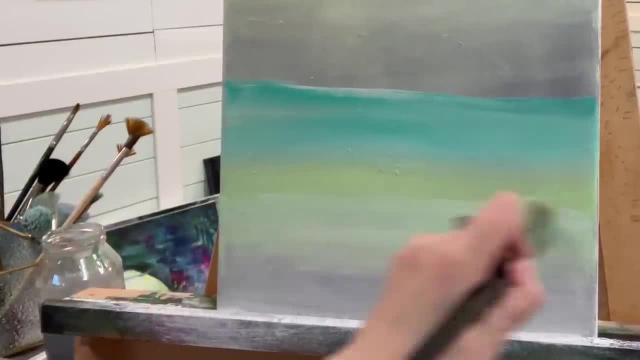 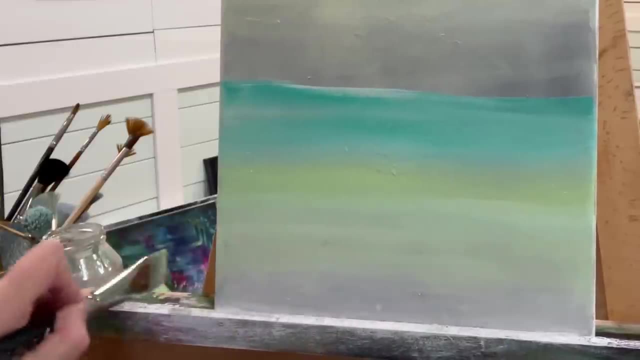 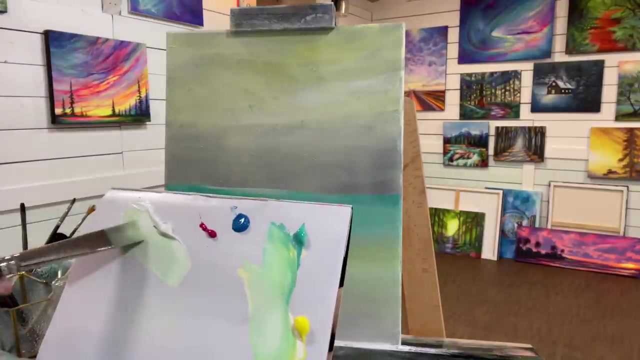 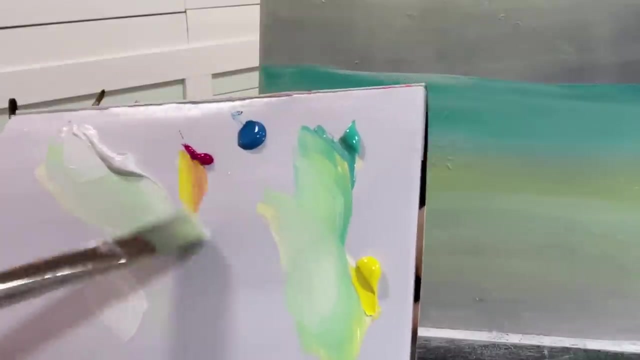 and you want to work quite quickly too. now i've worked most of that turquoise set in my brush, i'm left with a little bit of yellow and white. say, i want to make a beach color, sand color, i'll take a little bit of magenta yellow. 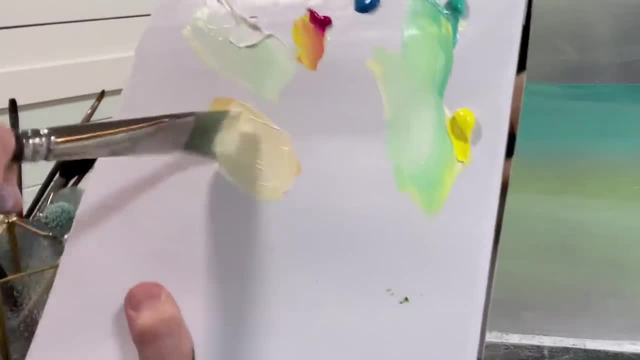 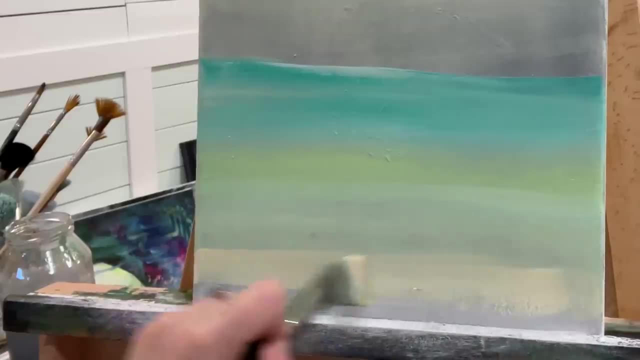 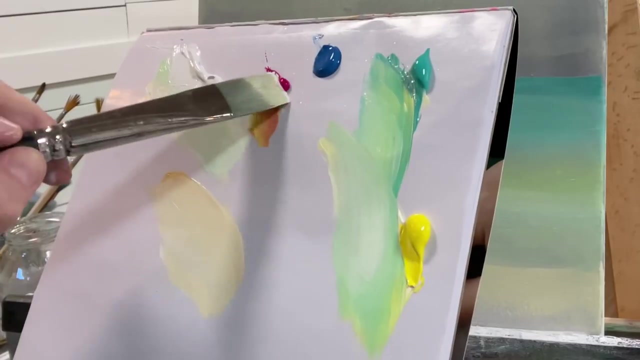 and white a little bit more, and i'll just sort of crisscross to blend those colors together and i'm going to start right over top of where i left off. now that looks a little bit yellowy still, so what i'm going to do is take a little bit more my magenta. 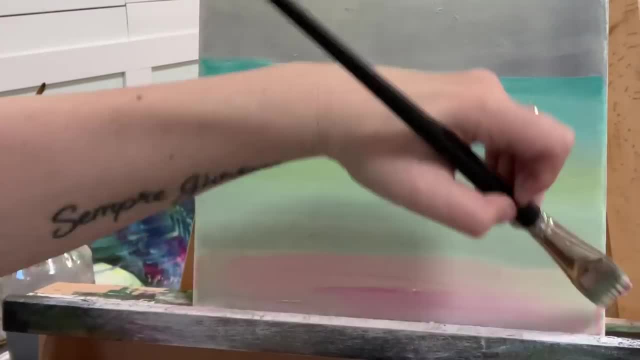 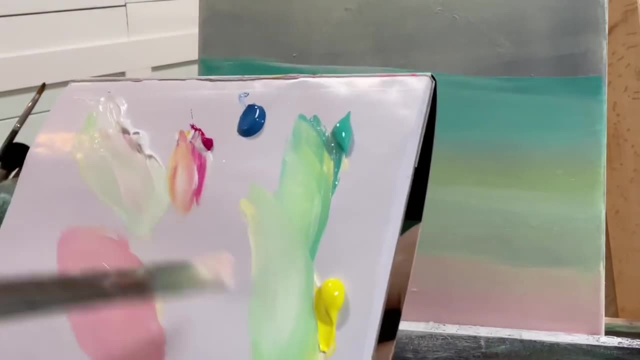 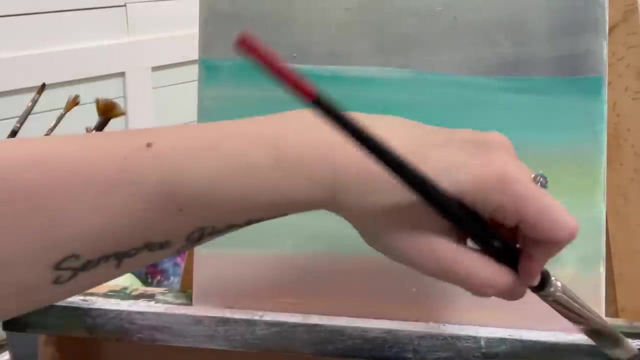 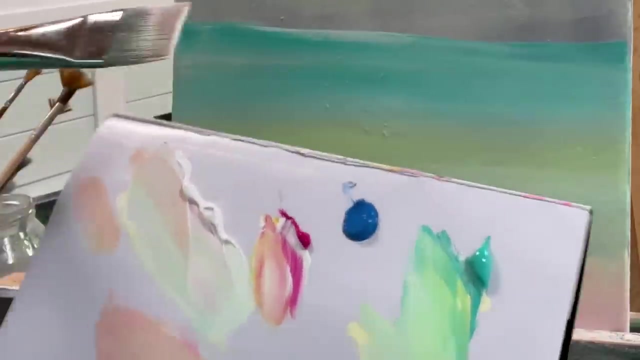 and make more of a pinky sand, and then i'm going to go over and balance it out. it's a bit too pinky for my liking, so just simply adding a little bit more yellow like that will even that out. i'm just going to push and cut right into that white and by using the tip of my brush now. 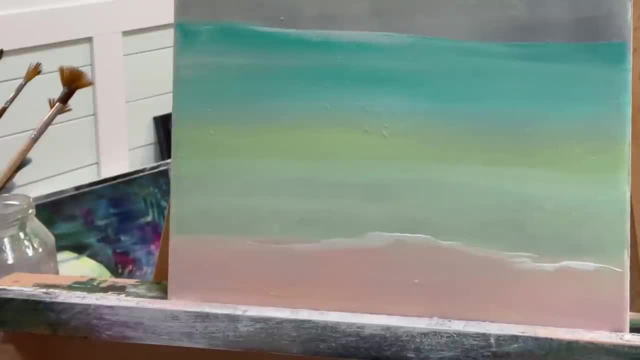 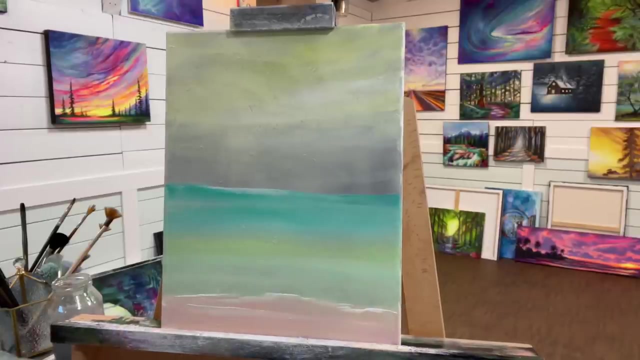 i can create a little bit of that white color. there we go, and then i'm going to take a little bit of this white foam and then we'll softly blend, pull back and forth and blend a little bit right there into the sand and wash all that out of my brush. 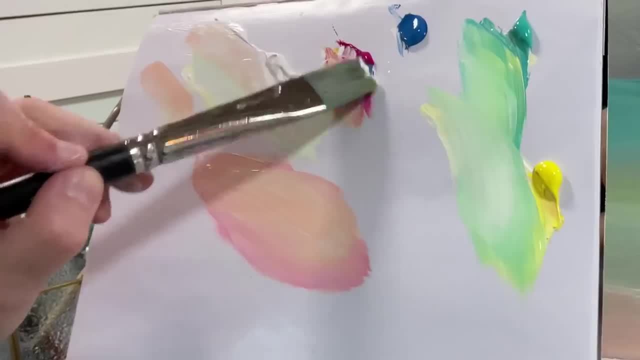 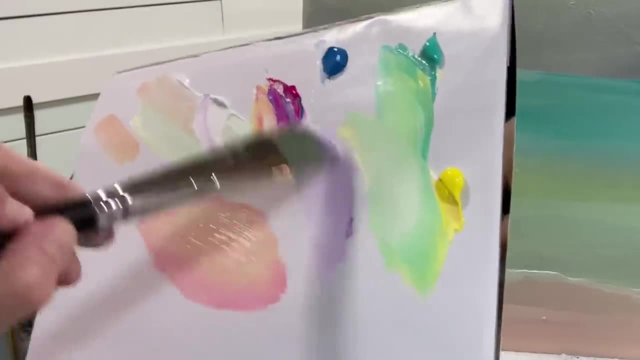 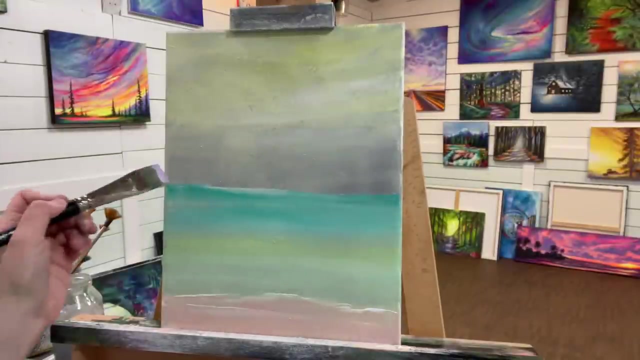 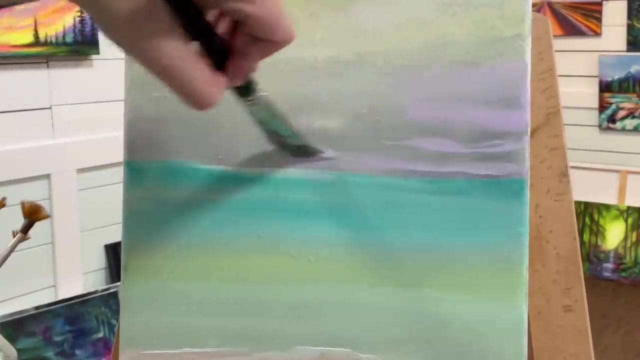 and i'm going to take a bit of white, cerulean blue. you can use any blue and magenta, so magenta blue and white- and we blend those together with water and we get a pretty lilac-y color that i'm going to use for some clouds in the sky here. 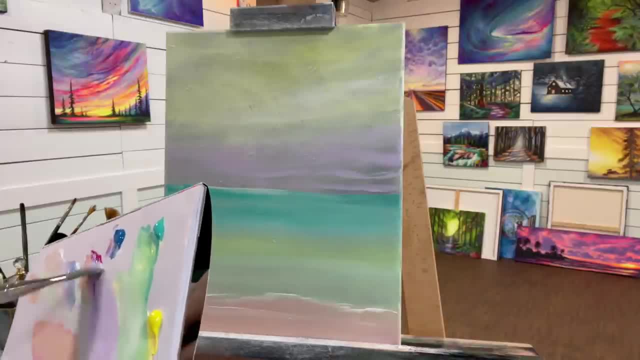 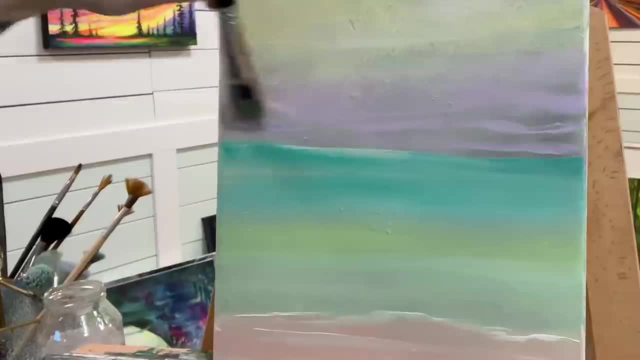 so see how easy it is to do that with a little bit of water. i'm going to finish that in a little teensy bit of수 of a few different colors and look how quickly that we've been able to do this. Now I'm going to take a bit of water and the paint that's left in my brush and 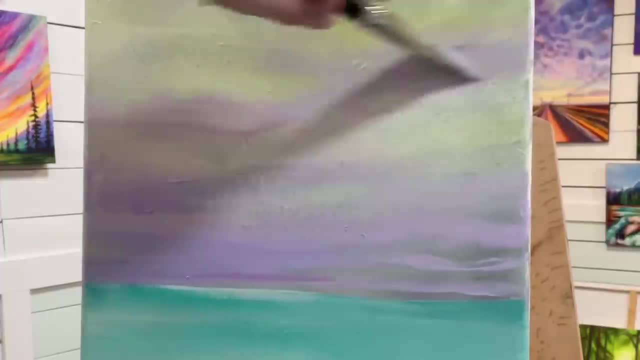 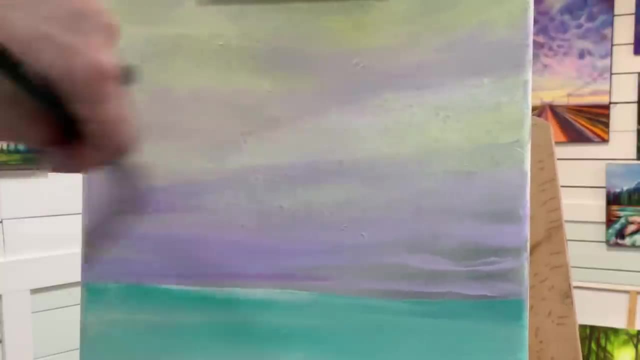 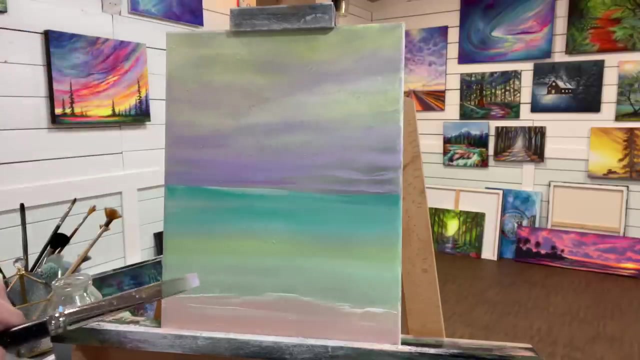 I'm going to work my way up and pull it into part of that yellow Now by now. depending on the drying time it takes for your paint to dry this, the yellow background could be all completely dry by now or it might still be a little bit. 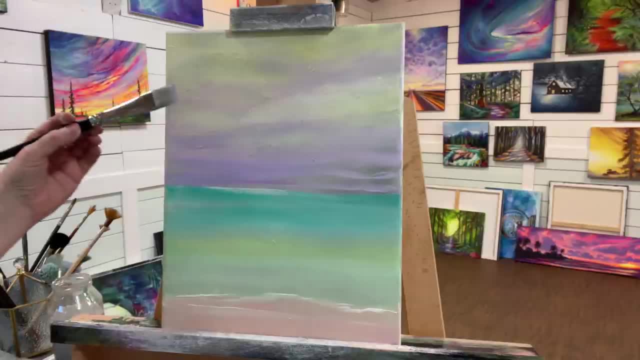 wet Mine's a bit in between. it's not that tacky. it's kind of tacky where you can. it feels a little bit sticky on my brush, so I either push a little bit harder with my brush to blend it in and take advantage of that. it's still a. 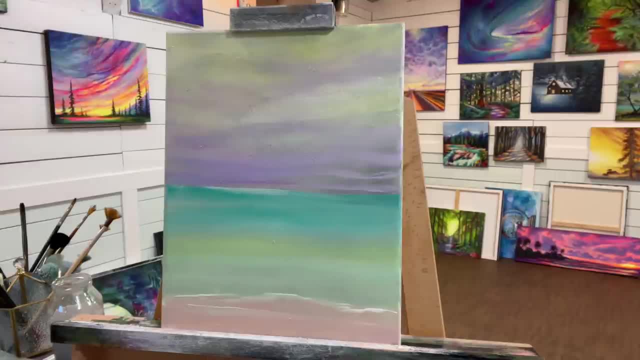 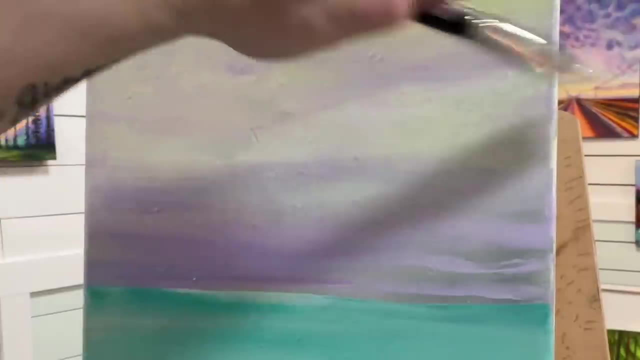 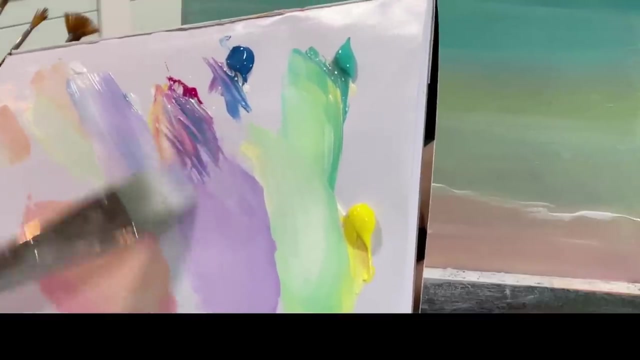 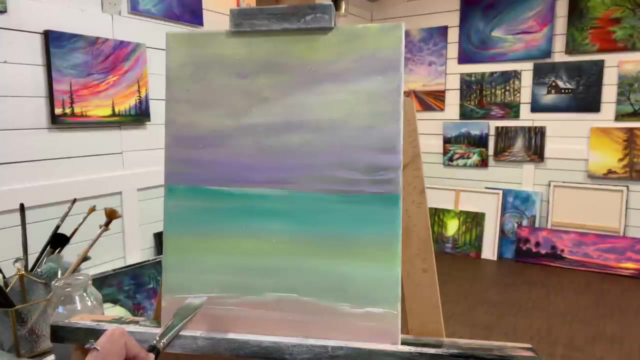 little bit wet, or you can just take a little bit of water. a little bit of a dry brushing also works too. so dry brushing, something kind of like that, where you hear that a light little brush, and then sometimes what I like to do is just take a little bit of shadow color, for in this case the blue and a little bit of purple. 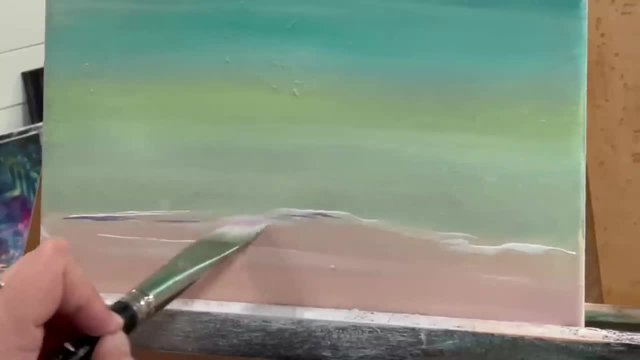 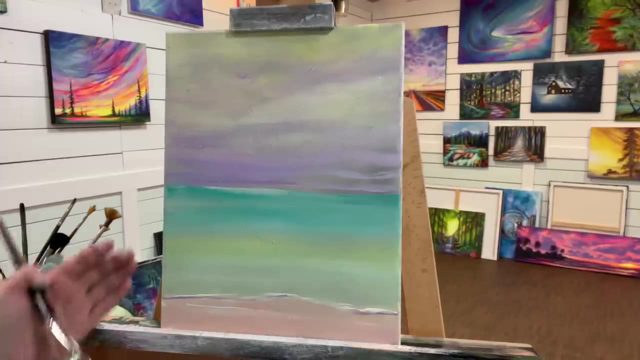 and just come right under this and create a little bit of a shadow under that wave and that kind of makes it feel like it's 3d that's coming up. So now I'm going to show you, guys, I'm going to paint a palm tree- and show you how to make green by blending and mixing. 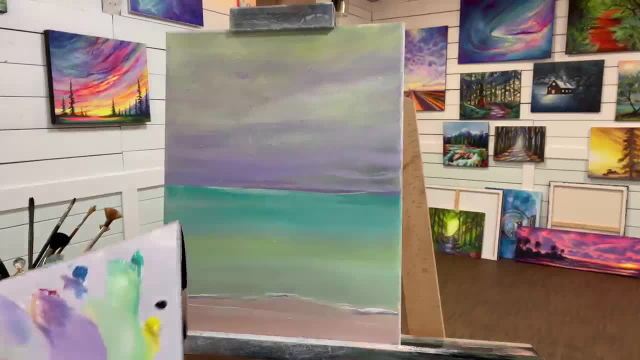 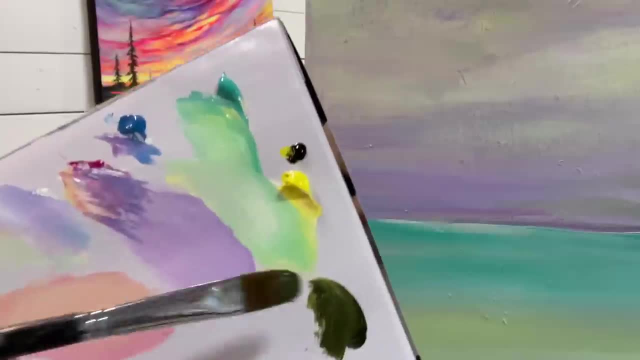 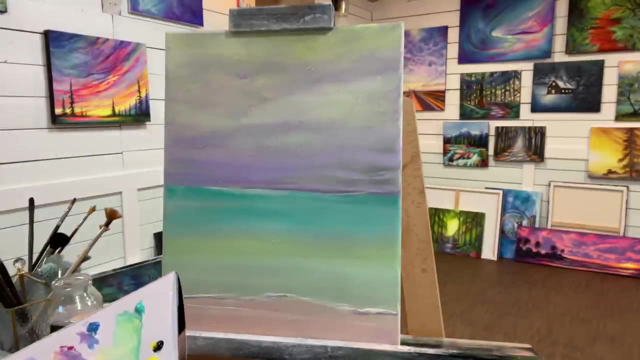 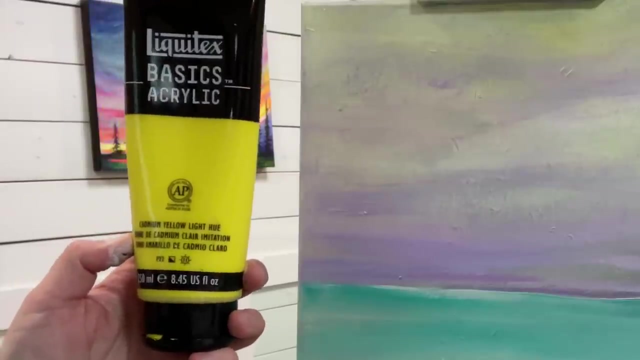 yellow and black together. The reason why I like to mix those two colors together- the yellow and the black- is because I get sort of an earthy or palm colored green. that is depends on what yellow you're using. the one that I'm using here is cadmium, yellow, light hue and it's by lipotex. basics: acrylic. 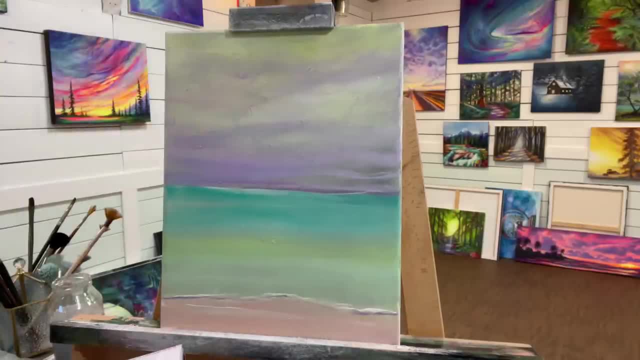 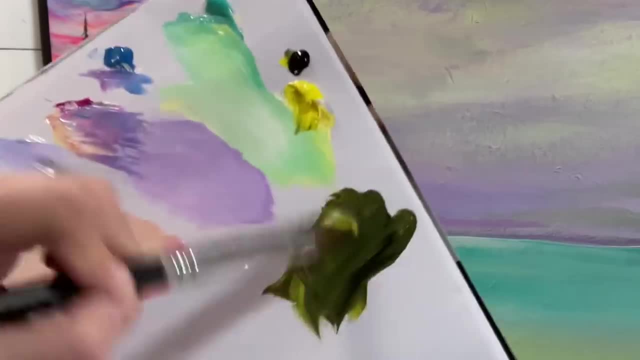 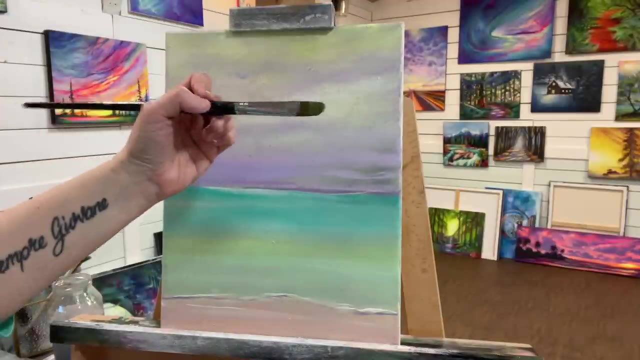 so, depending on what shade and hue of yellow you're using, it's going to change it. but it's kind of like fail proof. so I'm just going to crisscross, blend the two together and then I kind of pull off and get some on. mostly it's all over my brush, but mostly on the tip, and well, I'll. 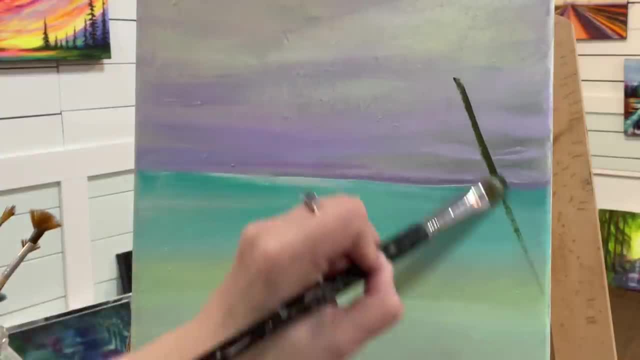 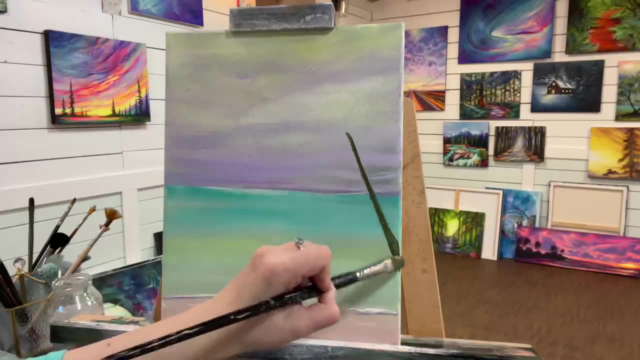 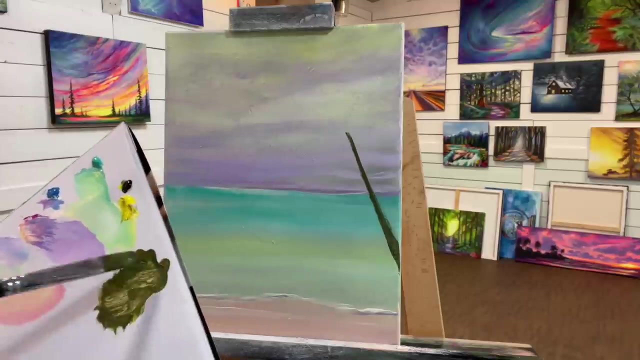 just the tree trunk's not really this color, but I'll add a little tree trunk here, making it a little bit thicker, and I need a little bit of water on my brush because it's feeling a little bit dry and I've got lots of paint on there, I just need to loosen it up. 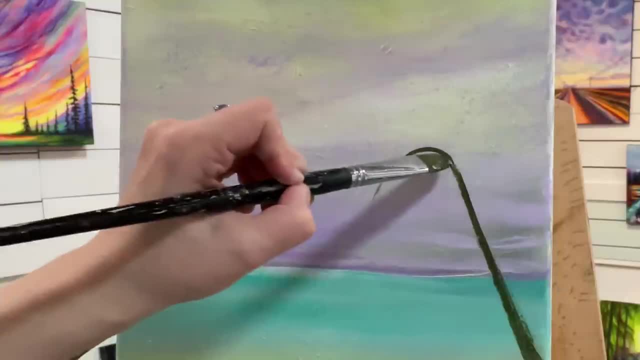 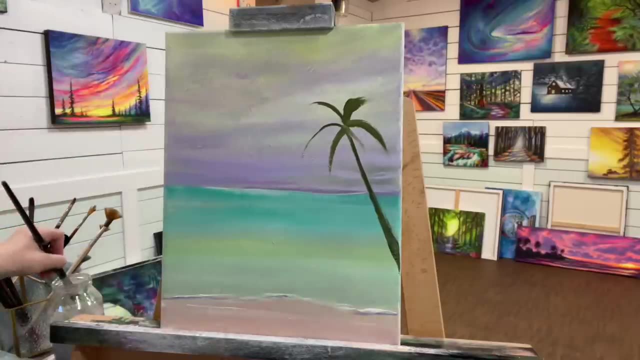 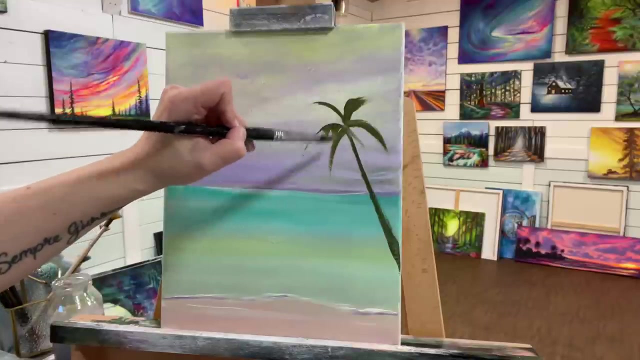 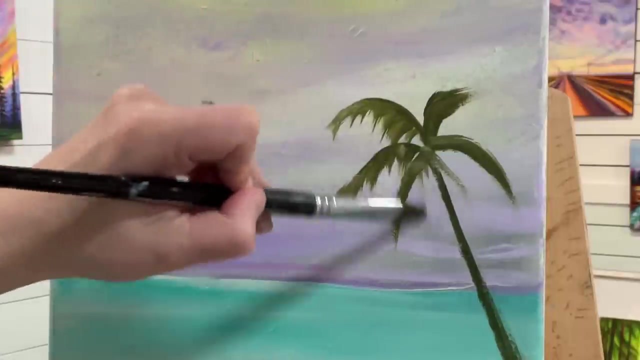 so I'm just going to start pulling, and I'm using the filbert brush for this, because I I really enjoy painting palm leaves with a filbert brush, and so you can see, I just went back for some more water, but I still have a lot of paint, so I know I don't really need yet to go back to more paint. 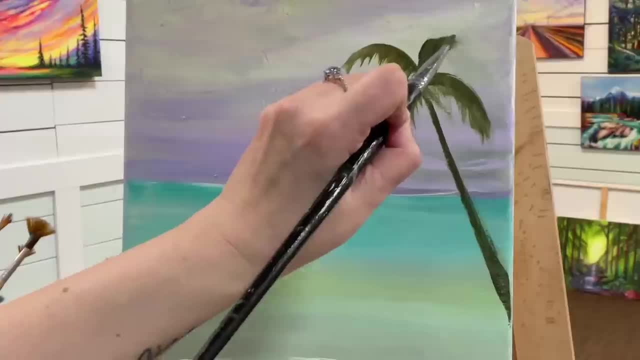 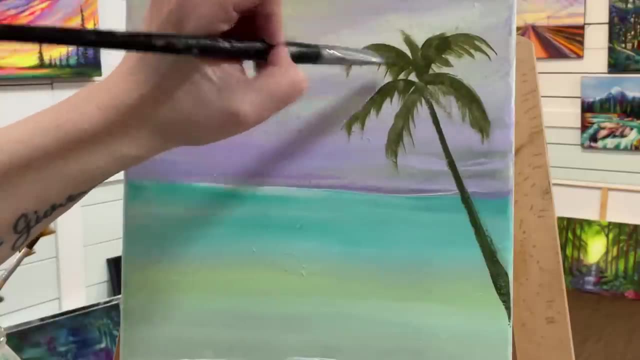 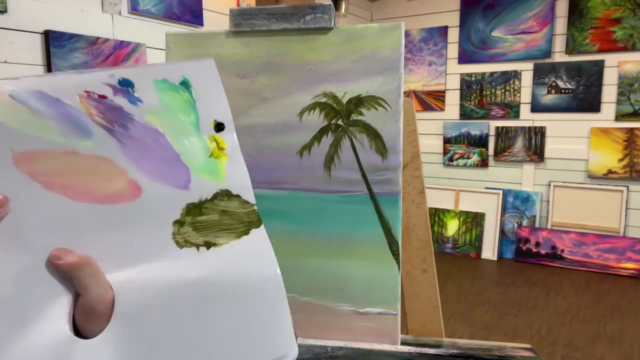 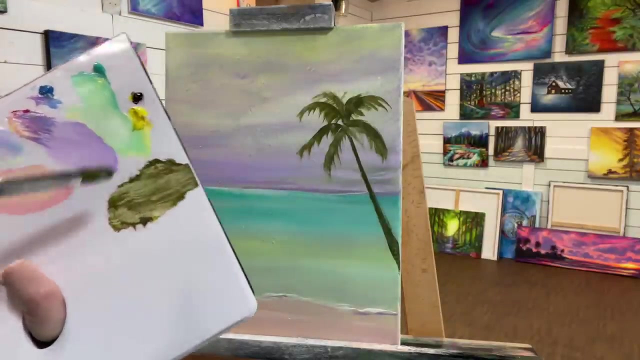 and a big part about um blending acrylics is the palette you're using too and you want. I'm using artisa paper palettes. they're very slick and you can see how it's shiny. it's waterproof, so it's not porous, it's not soaking up and taking that paint like a paper. 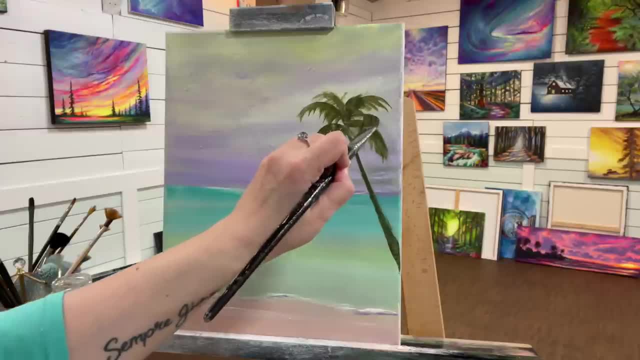 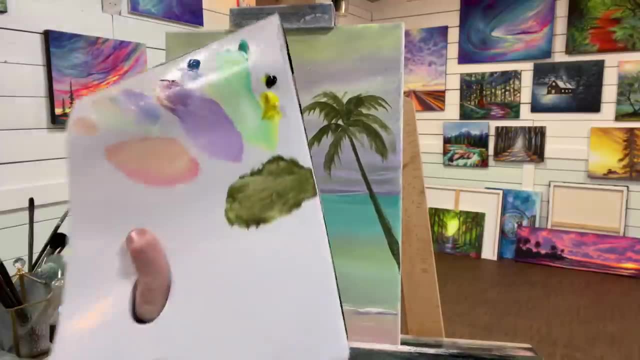 plate would. a lot of people don't use paper plates, guys, so I'm just going to go ahead and fill these in so you can see if you can be happy with the colors you want. if you happen to not have paper plates, then you don't want to waste so much paint. it just dries so fast and the paint 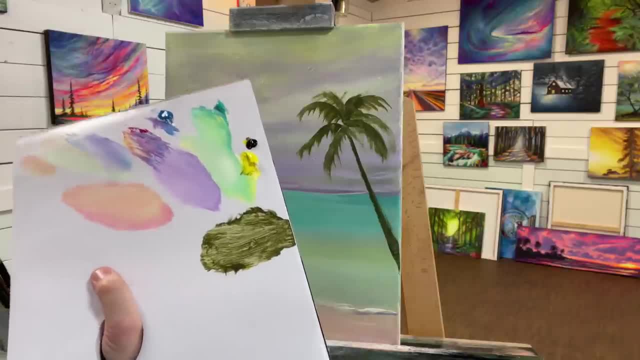 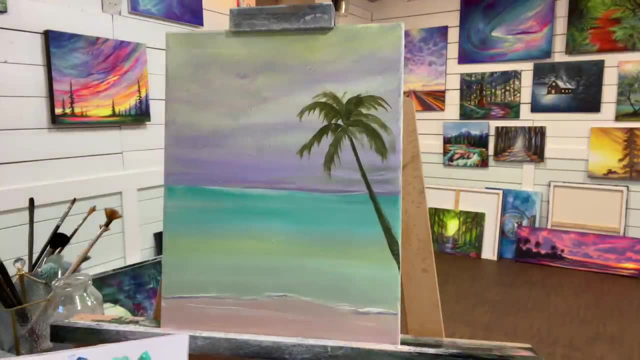 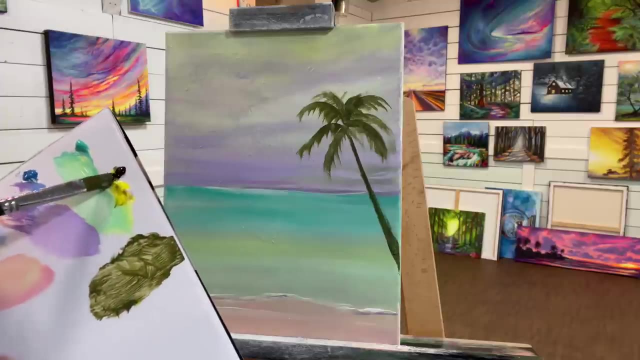 or the plate soaks it up. so use something that's waterproof, like this. you can use glass. you can use. there's glass palettes, resin palettes, anything pla old plastic lids, tupperware, a plate, a regular plate. don't use that for um eating off of after. keep that separate, obviously, even if you're washing. 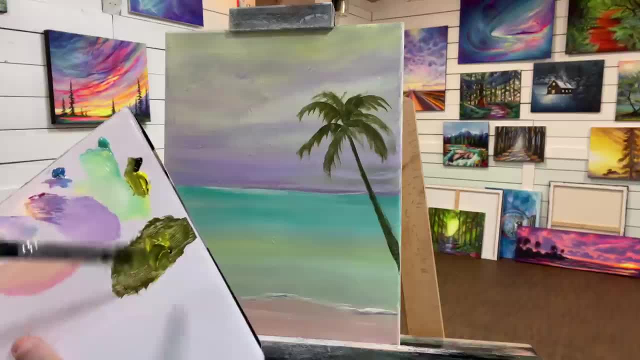 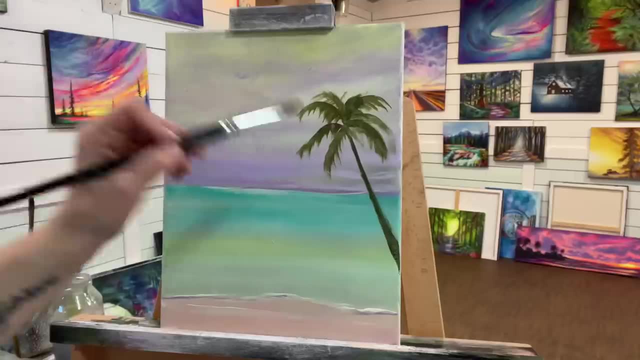 to mix up some more. I've taken a little bit of water, So don't you guys think this makes such a nice green? It's like a green, gold or olive green color. I love this green, especially when you're doing a painting with lots of pretty colors in it- Pinks and purples and stuff. It's nice to. 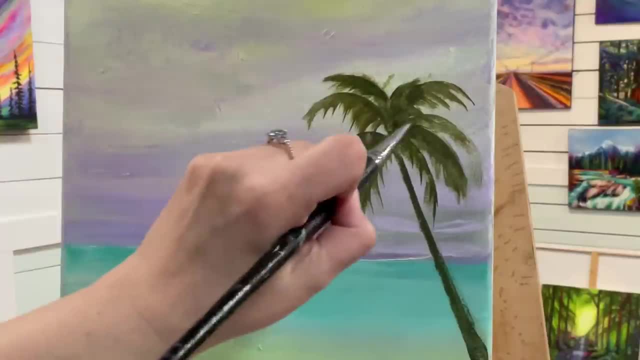 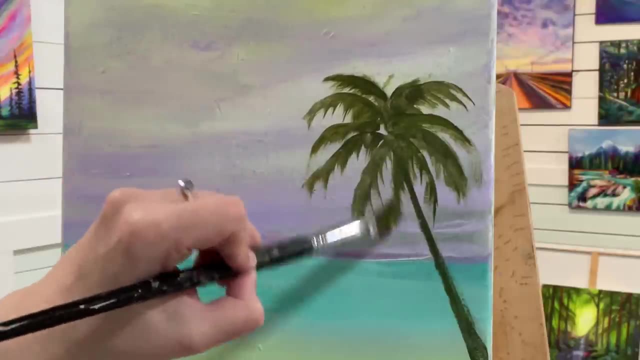 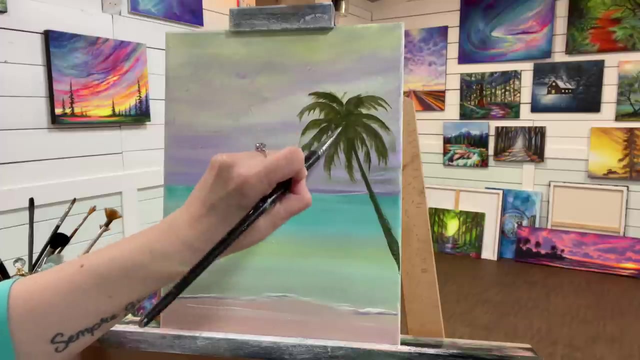 throw in some earthiness and I just love this color. So see, you've got a little bit of water on your brush and it takes a lot of practice. I can't really tell you exactly right how much water I'm using. It comes with practice. so just really, let's add a little bit of. 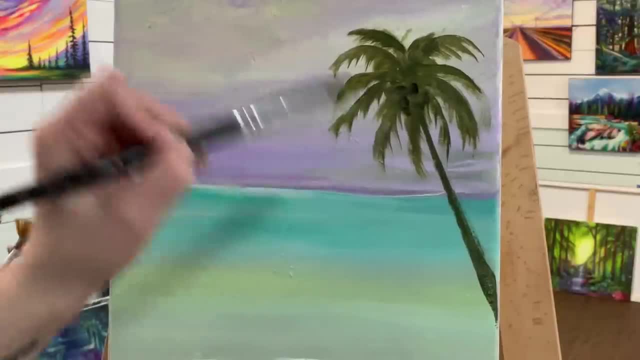 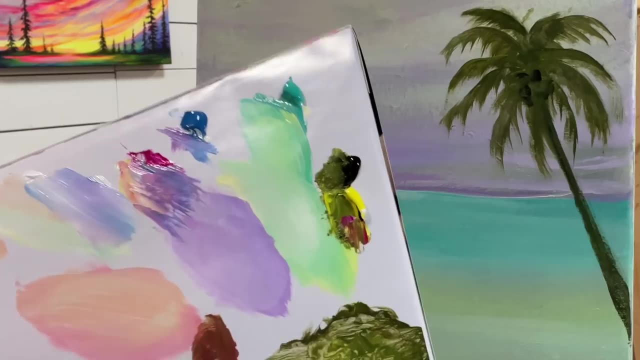 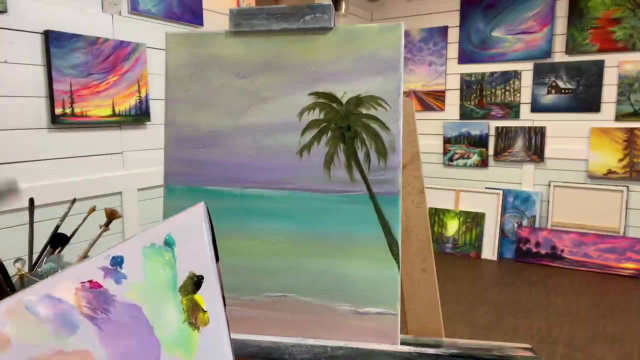 we've got some coconuts in there, a little bit of black, and it comes with practice and time, trial and error. Just take the time to practice one day and experiment with how much water you need and what it does and how it changes the flow of the paint. Okay, this is. 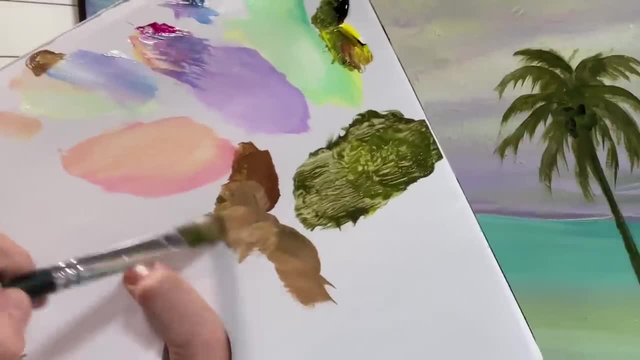 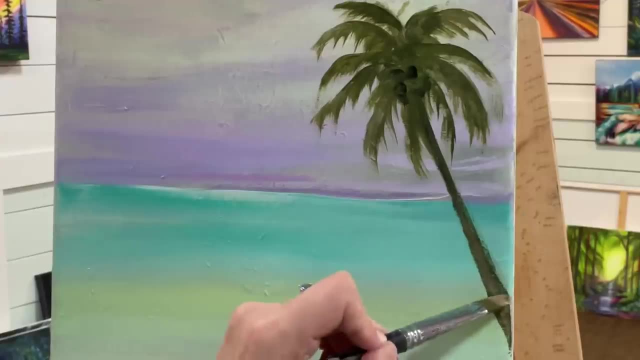 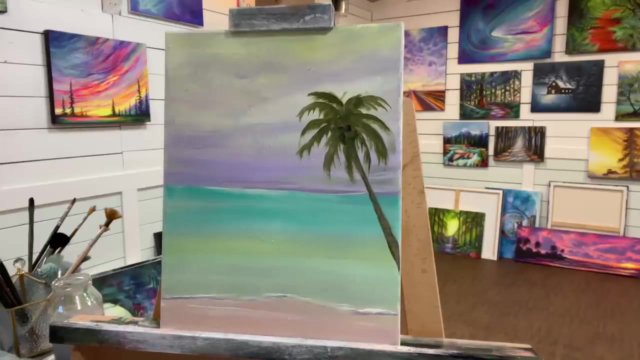 kind of where you want to be at. You want it to feel creamy and buttery, So I just took a little bit of my magenta yellow and white. This is for my tree trunk here. So before I finish up this video, I'll take a.